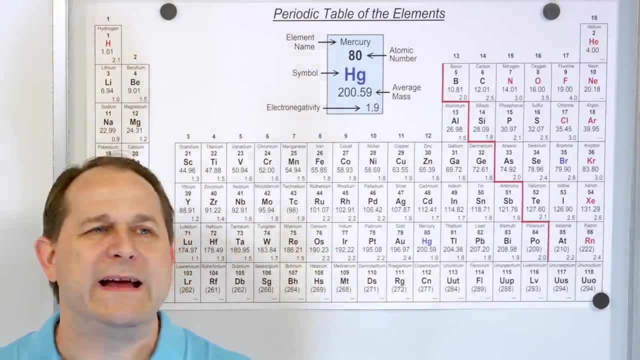 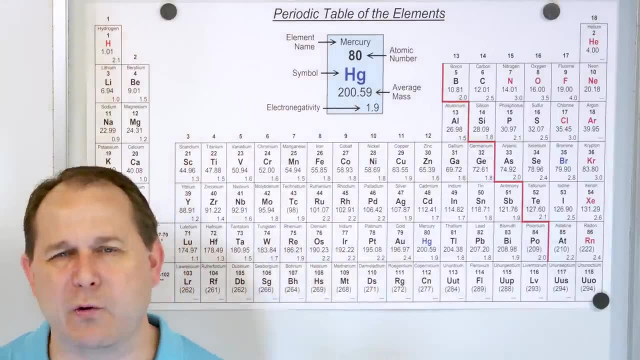 know uh had had uh pleasure or pain from, or any stimulus that comes into contact with your skin: a rash, any kind of food, any kind of- uh you know, playground equipment, cars, whatever, uh, your whole entire body is made of these elements and configured in different ways. 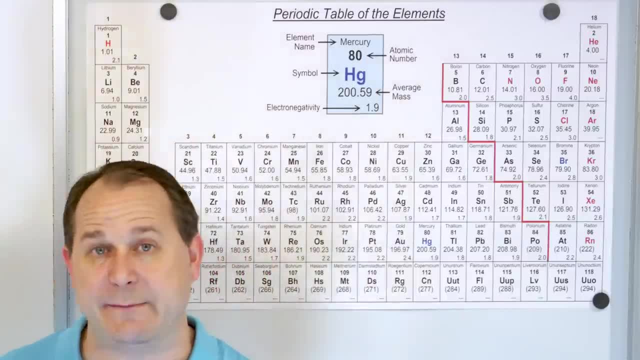 right. So what we're going to find as we study and examine this is that we're going to learn about the entire table. So let's get started, So let's get started, So let's get started, So let's start with our table. but we're also going to recognize that we're going to use parts of this. 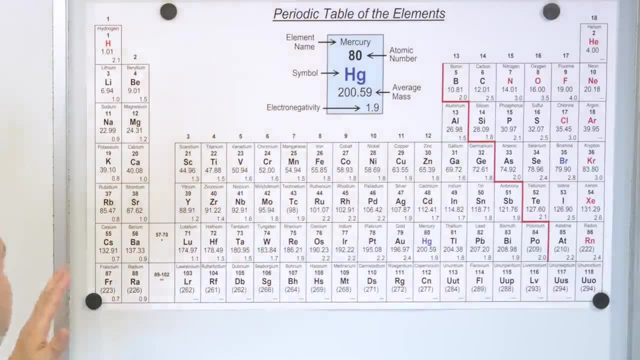 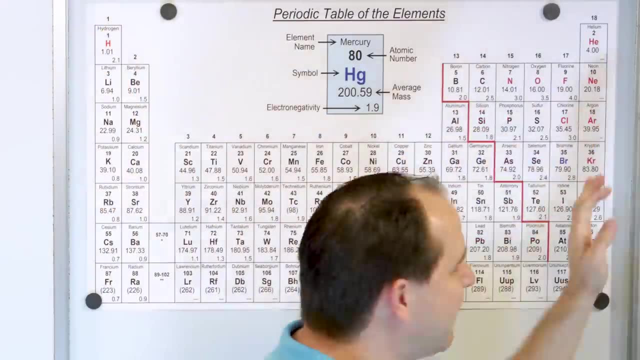 table a little more heavily than others. I'll tell you right now that we're going to learn the structure of this whole thing, but really we use the left-hand side of the table, and we use the right-hand side of the table more than anything else. Now, does it mean we never use the elements? 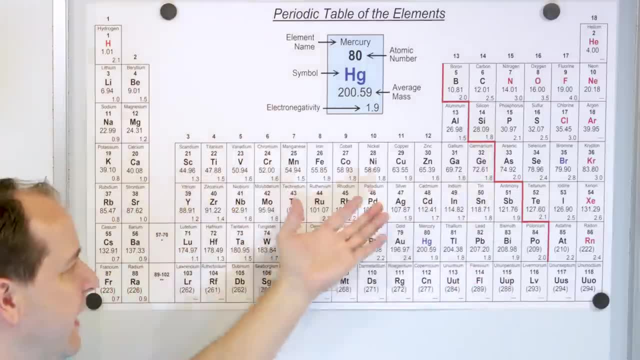 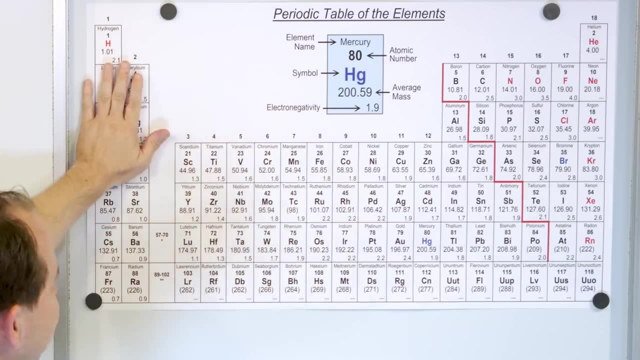 in the middle? Of course not, We use them, but we don't use them as much in a chemistry class, uh, which we call inorganic chemistry one or general chemistry. We use these elements here, and mostly these elements here, And of course we use these over here as well, Some as well. 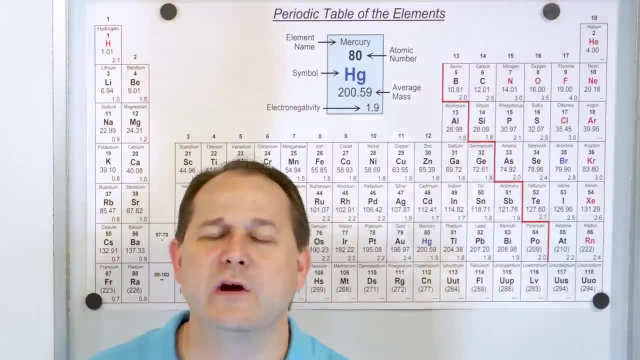 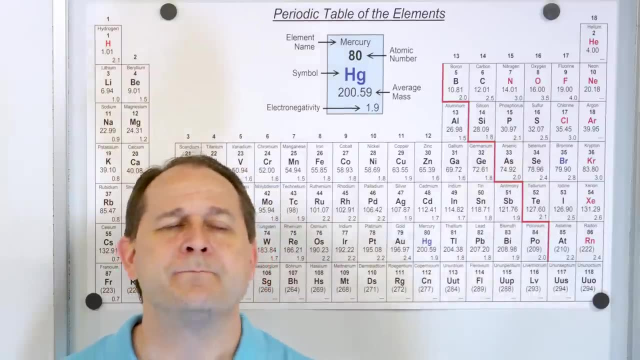 Now, later, after you take chemistry one and chemistry two, you take a class called organic chemistry. We're going to talk a lot more about what that means a little bit later, but basically organic chemistry is chemistry of compounds that contain carbon. All right, 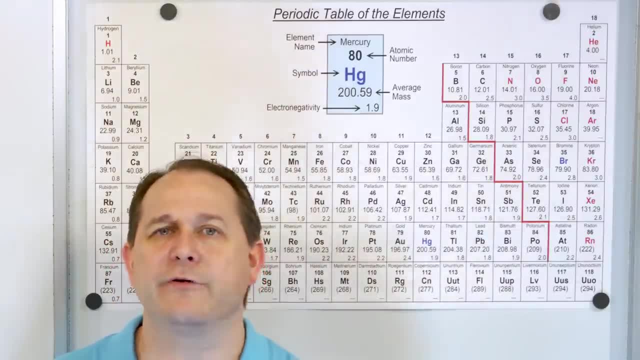 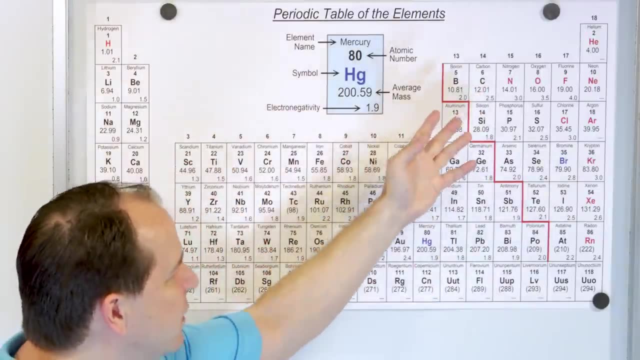 Carbon is a very special element because of the way it bonds to other atoms. It allows long molecules like DNA to exist. Carbon is right here on the periodic table And when we say, uh, organic chemistry talks about carbon, really it's carbon, along with a few other very important. 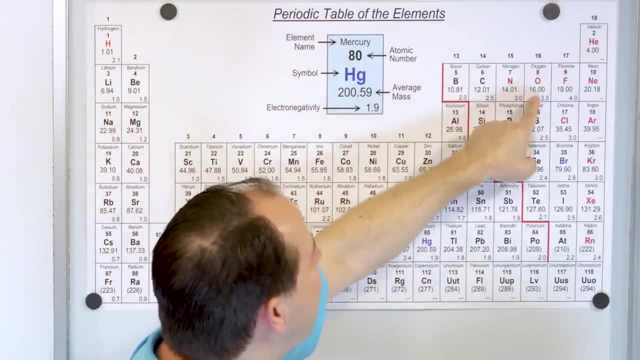 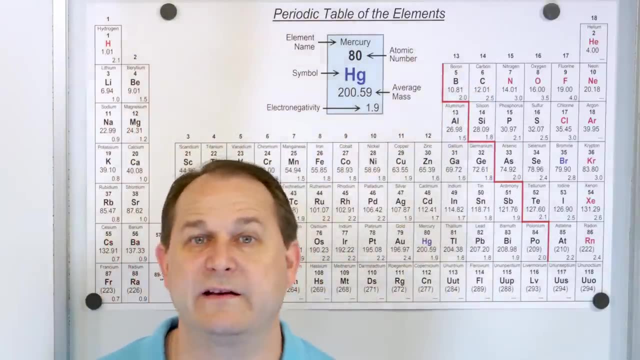 elements. So in organic chemistry you have carbon, nitrogen, oxygen, uh, hydrogen and then a few others sprinkled around And it turns out there's just a handful of elements. gives rise to life and the complexity of life, DNA and very complex molecules that we have to crawl before. 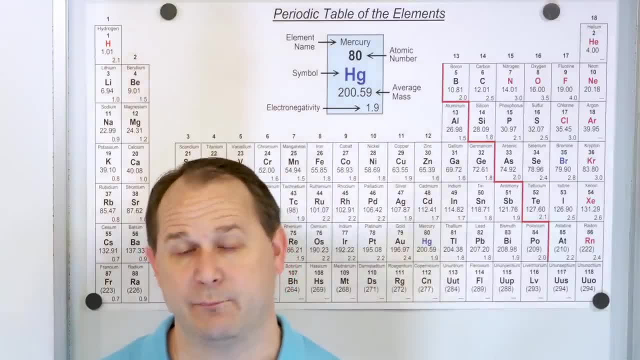 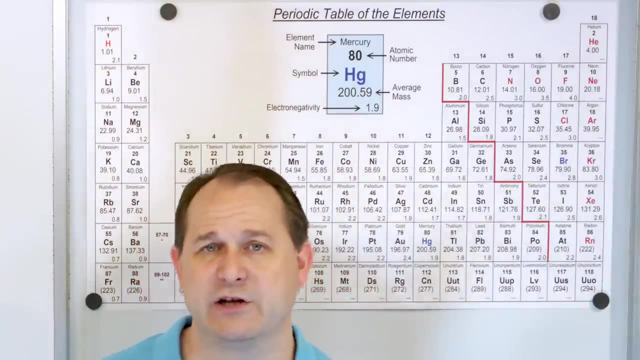 we walk. So how is this table arranged and why is it important? All right, The first thing you need to know is that this periodic table is arranged. It's a very complex table. It's a very complex table. It is arranged in order of increasing atomic number, Remember? uh, you can see right. 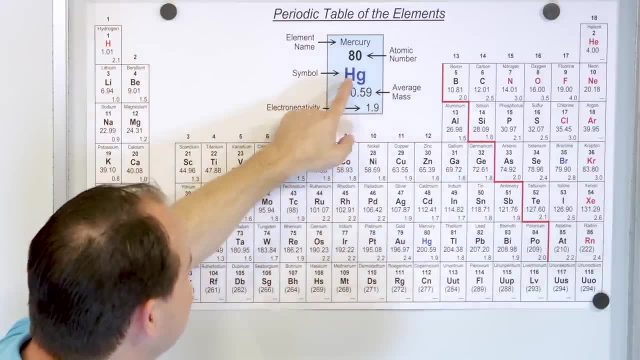 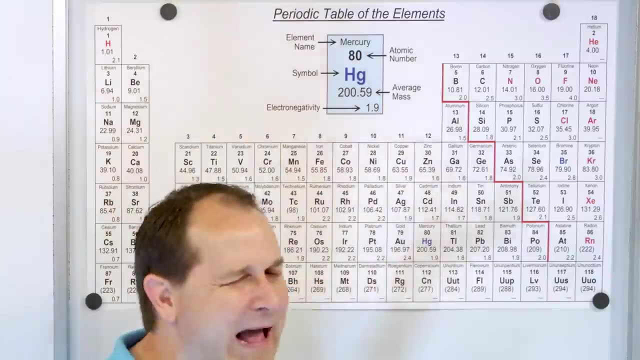 here in the legend, every square on this table has a chemical symbol or an elemental symbol, In this case H, G, uh is the symbol for mercury, And then the letters don't really match, because a lot of the time the element, the symbol for the element, comes from the Latin word that was used. 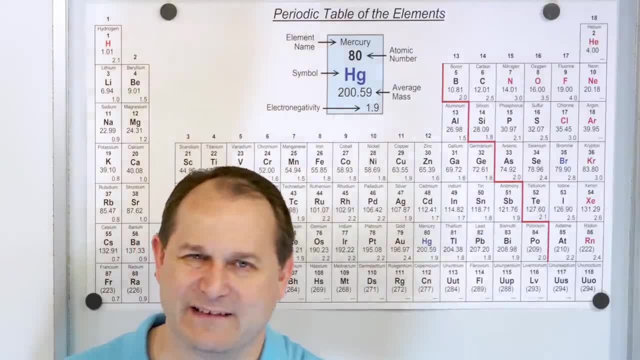 when it was first discovered. So H G, you know, is because of it's a Latin root, but most of the time it's like Oh for oxygen and N for oxygen, And then it's like Oh for oxygen and N for. 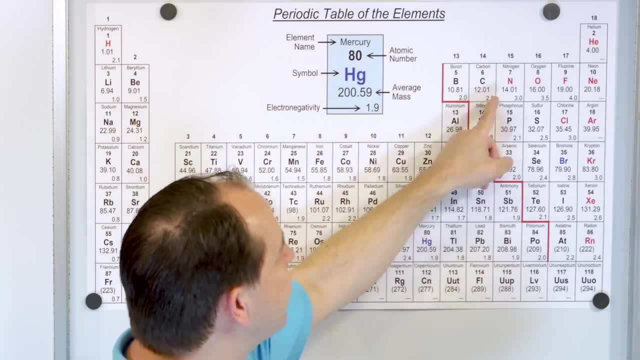 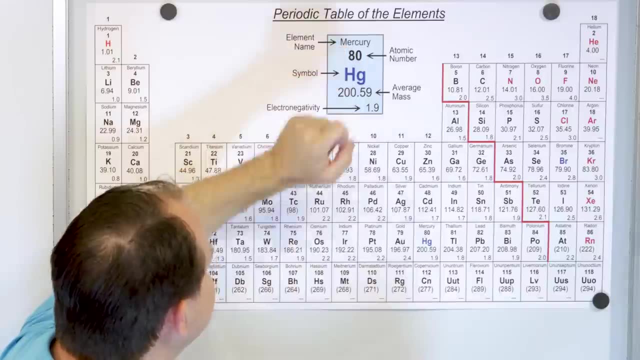 nitrogen, and C for carbon, and B for boron and P for phosphorus, And most of the time it lines up, but sometimes it doesn't, Okay. And then, on every one of these squares, we have the name of the element, We have the atomic number. Remember, we've already learned: the atomic number is the. 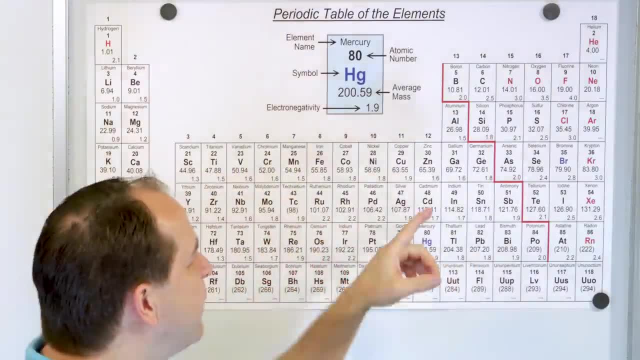 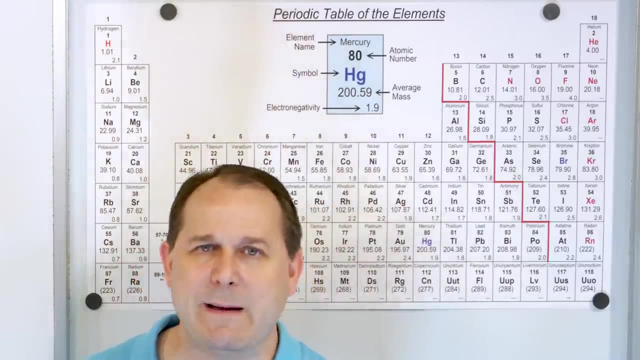 number of protons in the nucleus, All right, And then, of course, we have the average atomic mass down here, which we've already already also have learned about in great detail. The atomic mass, just as a reminder to you, is the average, the weighted average of all the different isotopes. 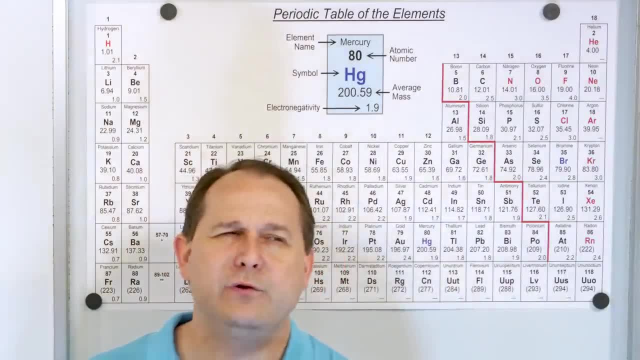 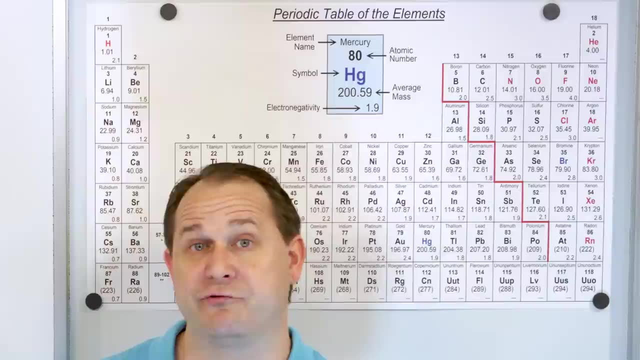 of an atom or an element. So if you don't know what those words mean, then go back to my previous lessons, because we discussed it in great detail. Basically, in the nucleus we have protons and we have neutrons. So what makes a element different from its neighbor is the number of protons in the 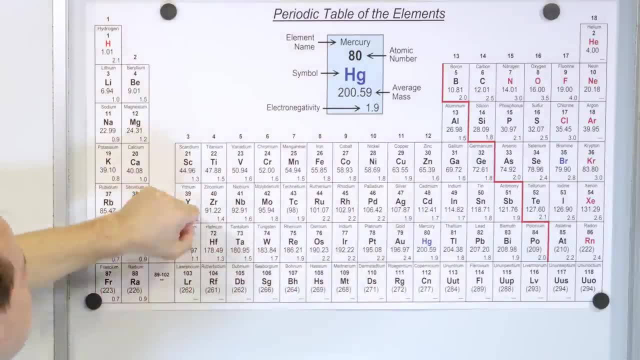 nucleus, right. So this is a hydrogen: has one proton in its nucleus and two in helium has two protons in its nucleus. Lithium has three protons in its nucleus. So this is a hydrogen: has one proton in its nucleus. and beryllium has four protons in its nucleus, But in the nucleus. 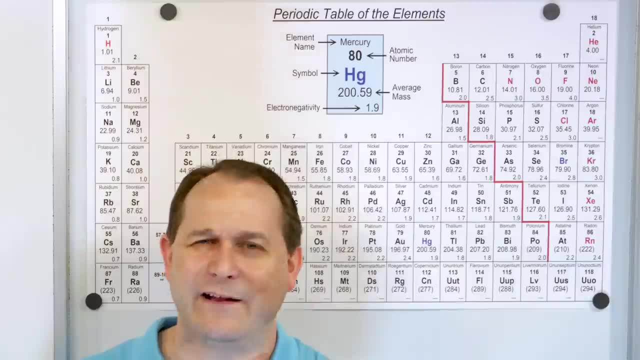 in addition to the protons, we also have neutrons, And that's where things get a little fuzzy, because the element is defined by the number of protons you have, but the nucleus can have a varying number of of neutrons, which makes it either heavier or lighter, And those we call 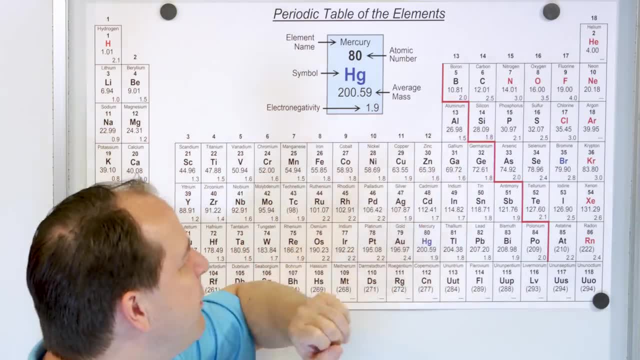 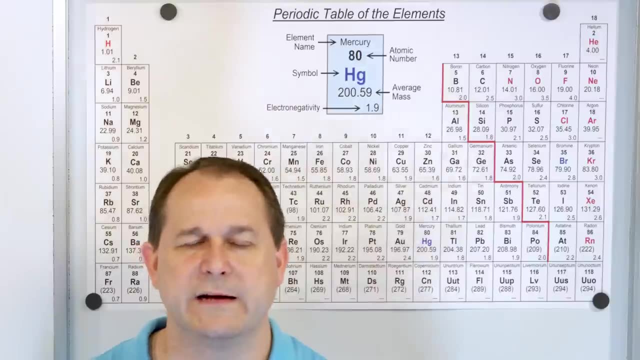 isotopes, So we may have different isotopes of oxygen, We may have different isotopes of carbon, but they're all chemically the same element. It's just they may have more or less neutrons in the nucleus, And so we have different isotopes of oxygen. We may have different isotopes of carbon. 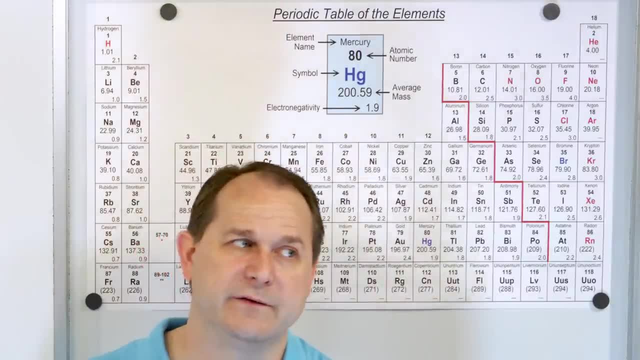 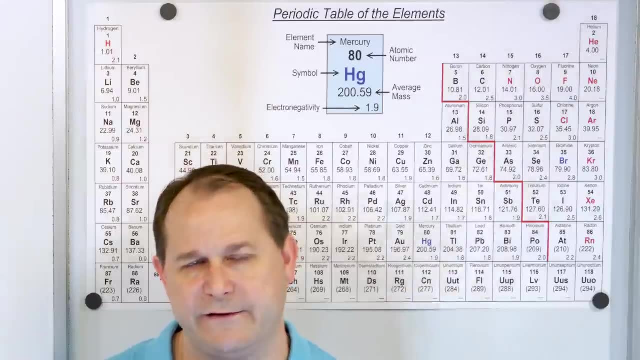 and that is what gives rise to different, different weights of of those isotopes And they exist in different, in different percentages in nature. There's always a most stable common isotope. So this average atomic mass is taking the average of all the different flavors of the. 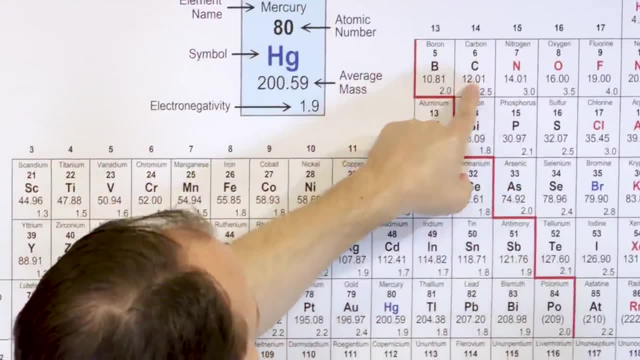 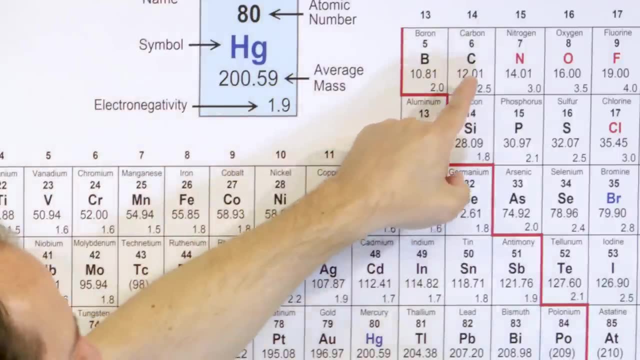 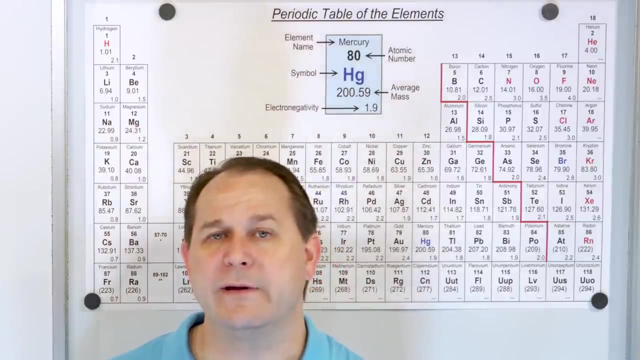 isotope. So, for instance, nitrogen, or let's look at carbon, has a average atomic mass of 12.01 atomic mass units. This is the weighted average of all the different flavors, which we call isotopes of carbon, that exist in nature. We have a very common stable isotope of carbon that we have all. 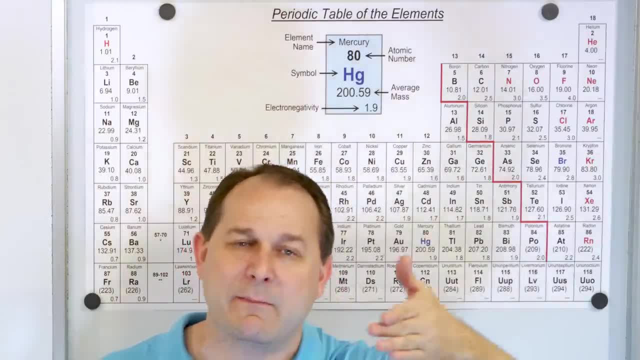 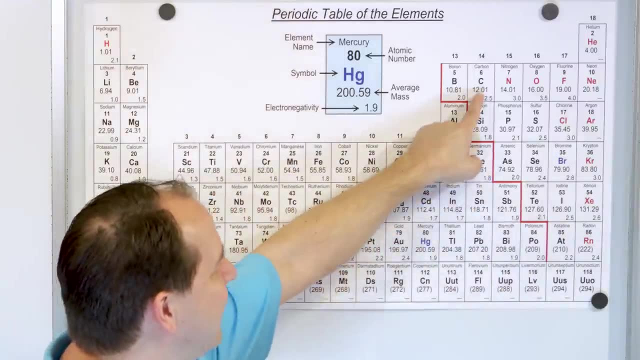 around us, And then we have some others that are not so common. So when we mathematically average all of the common ones with the uncommon ones, which all have different masses, we get an average mass. And that average mass is what is printed everywhere on this table. So every number 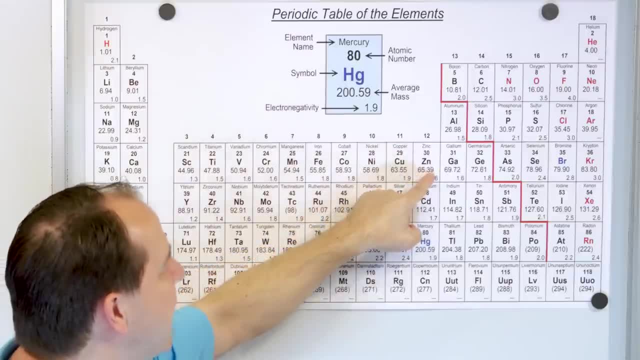 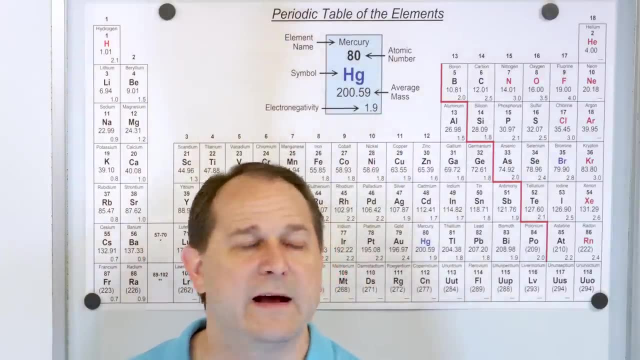 for instance, zinc here has a mass of 65.39 atomic mass units, but this number is the weighted average of the different isotopes that exist in nature for that element. And every number of the isotopes, every element is like this, Okay Cause, every element, with very few exceptions, I believe. 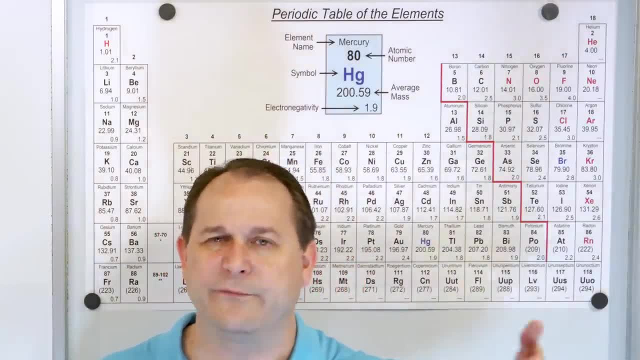 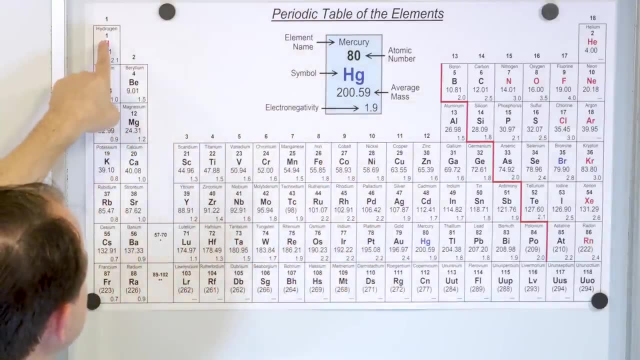 we always have different, different amounts of isotopes, which can be different numbers of neutrons in the nucleus. So the big big thing to understand is this thing is arranged: an increasing atomic number. If you have an element with only one proton, we call it hydrogen. 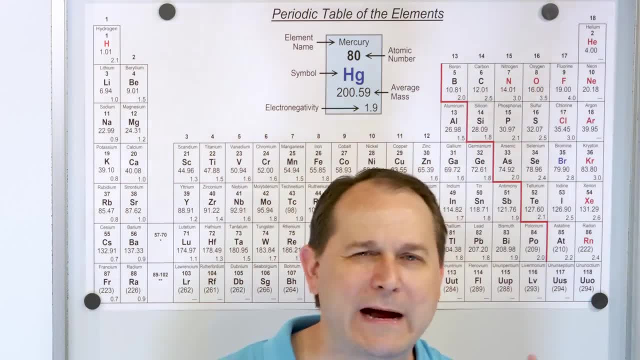 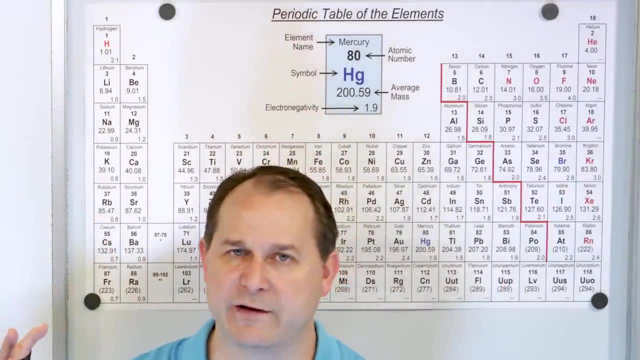 If you add a proton to it, then you get something called helium. Now remember, every one of these elements are neutral atoms. So you have to have for a neutral atom the same number of electrons on the outside orbiting around or in the electron cloud around the nucleus. you have the same number. 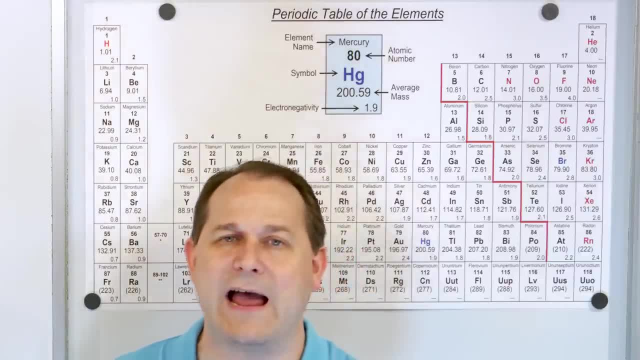 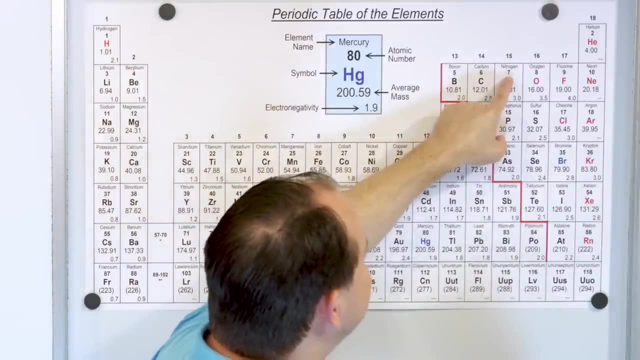 of electrons, as you have protons in the nucleus, in order for you to have a neutral atom. So, without writing it all out, you know that nitrogen, for instance, has seven protons in the nucleus and it must have seven electrons surrounding the nucleus. You know that chlorine has 17 protons. 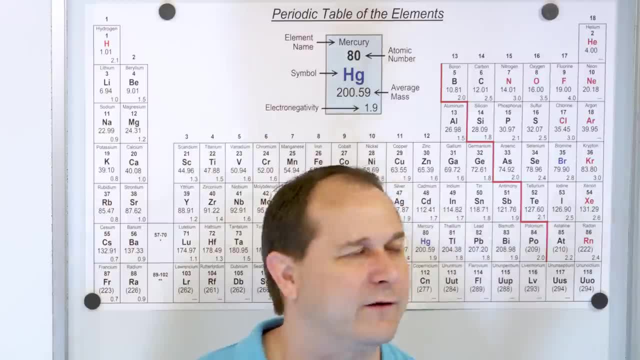 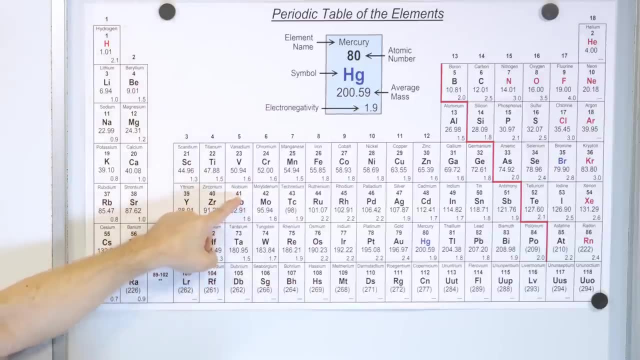 in its nucleus and it must therefore have 17 electrons around its nucleus. And the same thing you know, you have, you know niobium, for instance. niobium has 41 protons in the nucleus and it must therefore have 41. 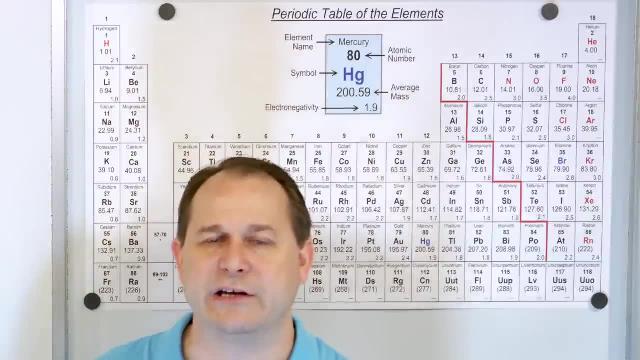 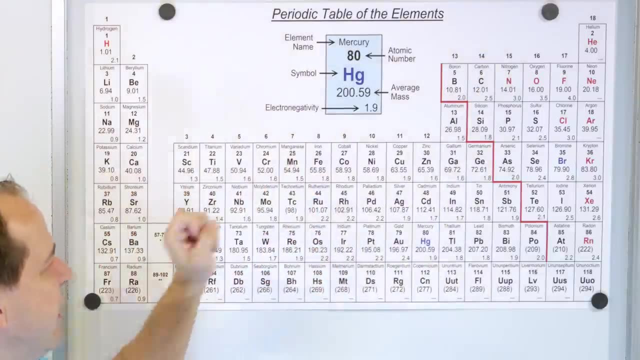 electrons surrounding the nucleus to have an electrically neutral atom, And then each of these also have varying numbers of neutrons, And so all of that goes into the calculation of the mass. So the thing to remember, though, is, as you add protons to the element, it becomes a new. 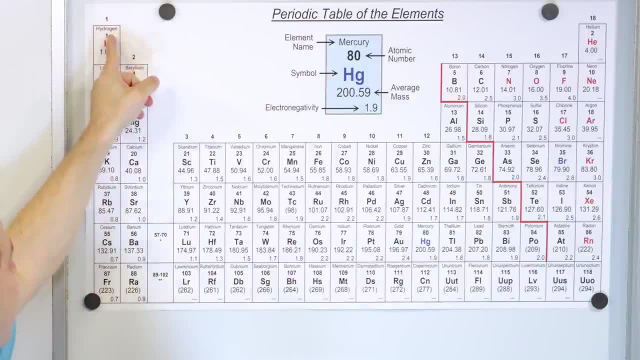 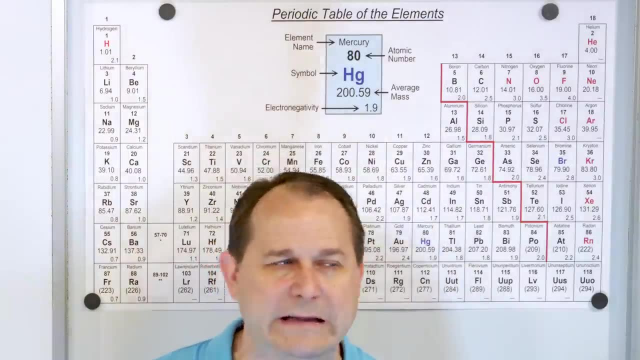 element. So if I start with hydrogen, if I could magically add a proton in the nucleus, then it would make helium. In fact, when you fuse hydrogen together in a nuclear reaction, it would make a proton. So if you start with a proton and add a proton to it, then you can make some helium, If you. 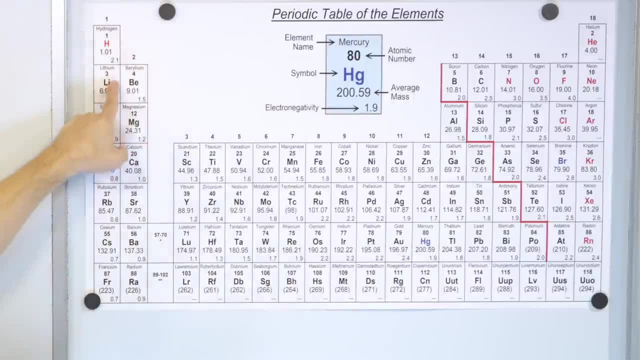 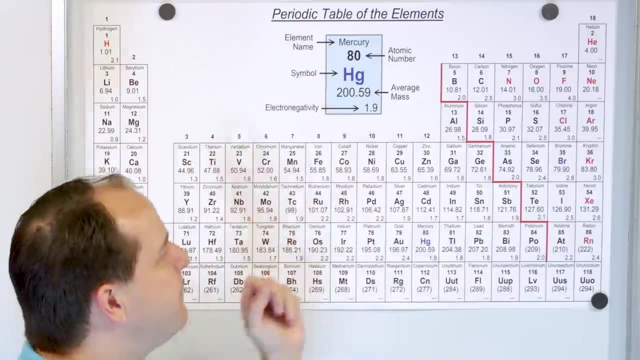 take helium and you can add a single proton to it, it becomes a new element called lithium. If you start with lithium and add a proton to it, then it becomes beryllium, And you see how this goes. So it's the periodic table of the elements, but it's arranged in order of increasing atomic number. 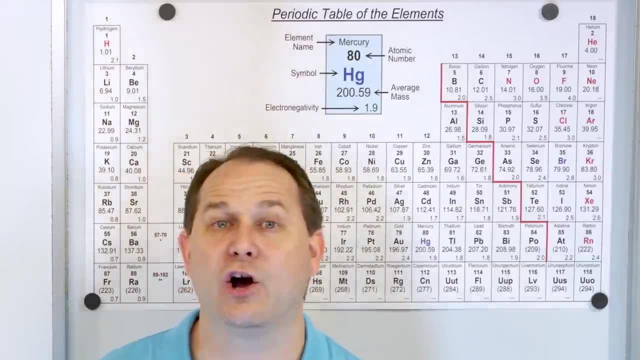 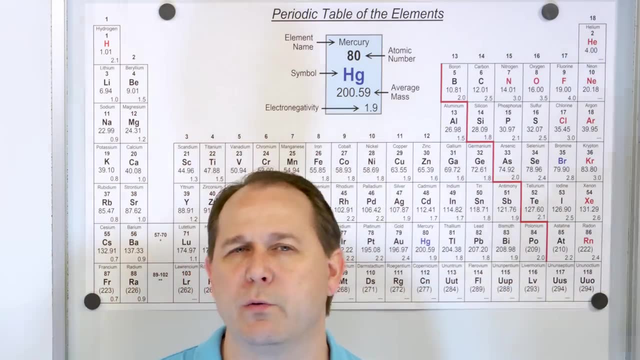 Now let's talk about the elephant in the room. Why is it called the periodic table of the elements? Why is it periodic is what I'm trying to say. So forget that we have this table now. Forget that we know what it is. Forget that we understand that we know what it is. Forget that we know what it is. 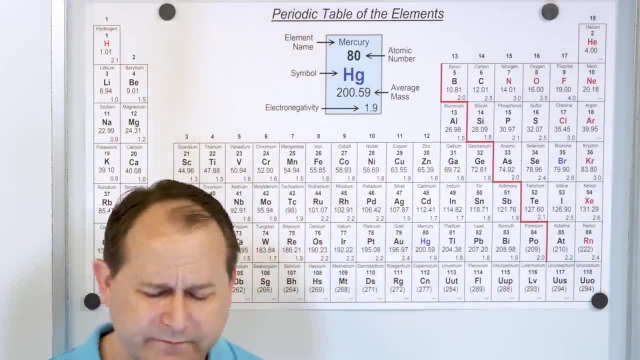 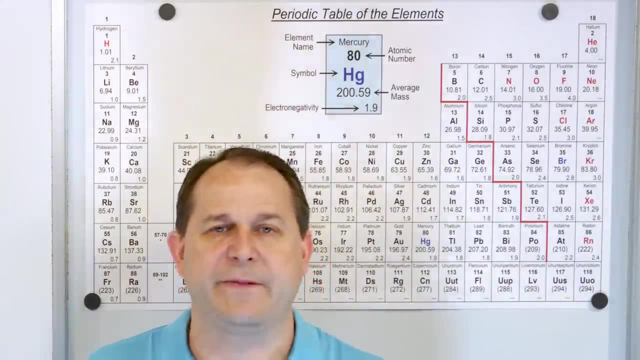 Anything about chemistry. You live a couple hundred years ago and you're a scientist and you just have a lot of things in nature that you're studying and you believe you boil them down to these fundamental things that are all different from each other and you call them elements, or 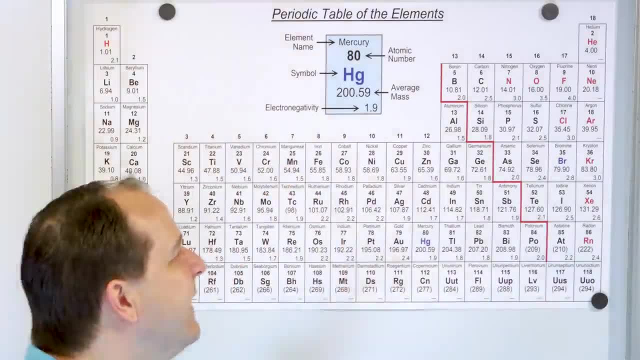 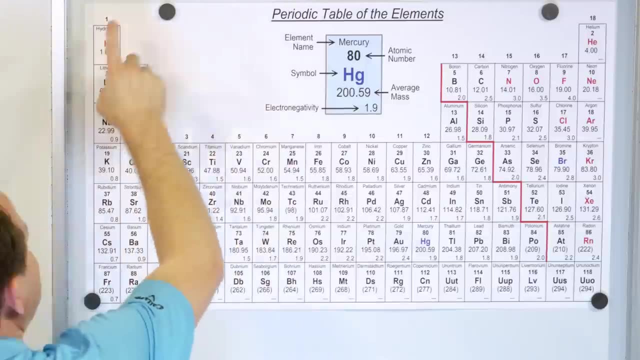 call them atoms. Okay, What you basically figure out is that what happens is when you, when you make a list of all of the things that you've collected from from you know, from your lab, and you arrange them in order of atomic number, what you basically have is you have some periodic 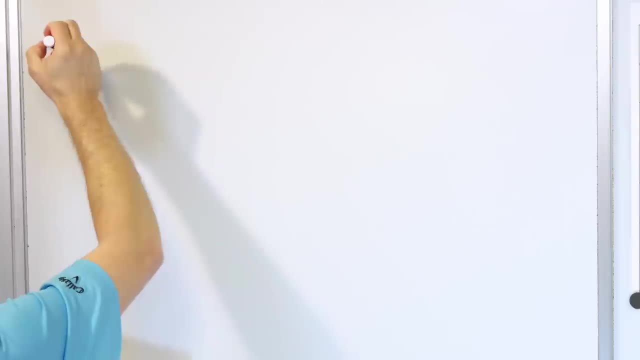 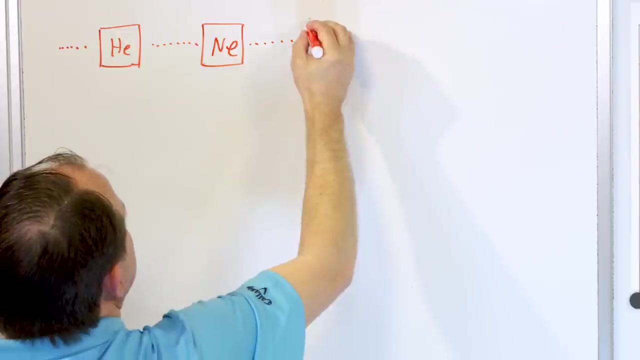 periodic behavior in the atoms. So what you have is you have an element over here and then you get to an element that you call helium, right, And then you have some other elements here, and then you end up with another element that you call neon, And then you have some other elements here. 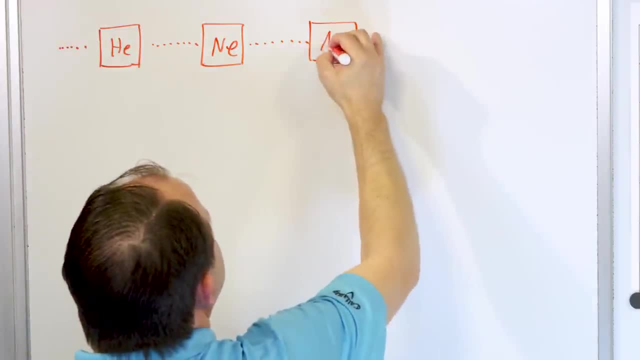 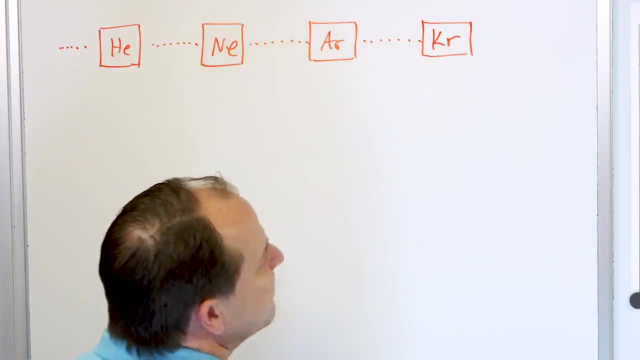 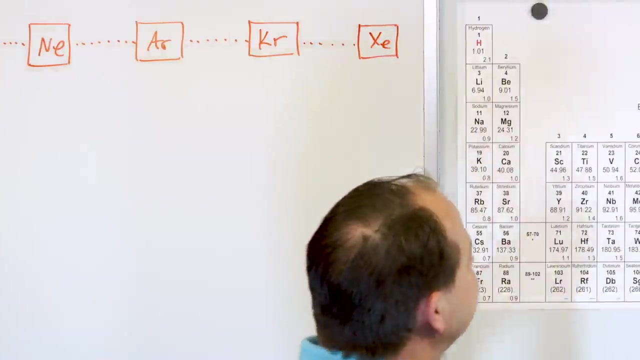 and then you, you end up with another element called argon, And then you have some other elements, and then you end up with another element called a krypton, like this, And I can keep going. I'll just do one more. And then you have another one here called xenon. You see, what I've done is I've basically written. 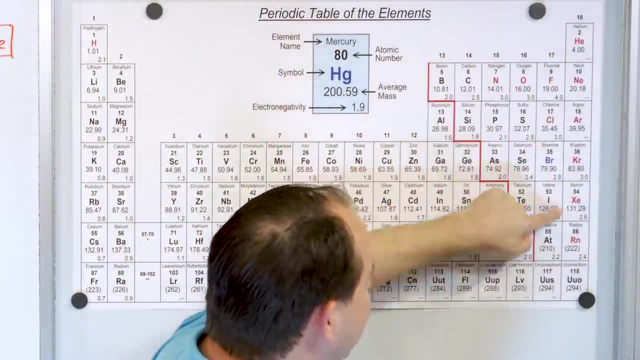 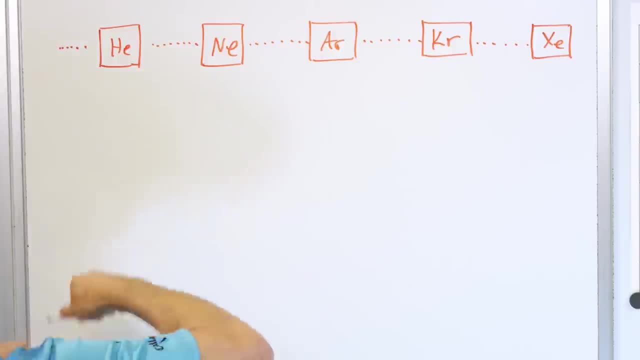 down these elements on the right hand column here. You'll understand why it's in the right hand column in just a second. But let's say you don't know anything about chemistry. What you notice is that every so often you have a non-reactive gas, non-reactive gas And the 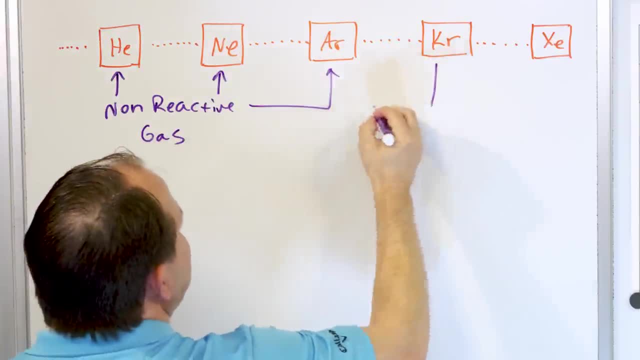 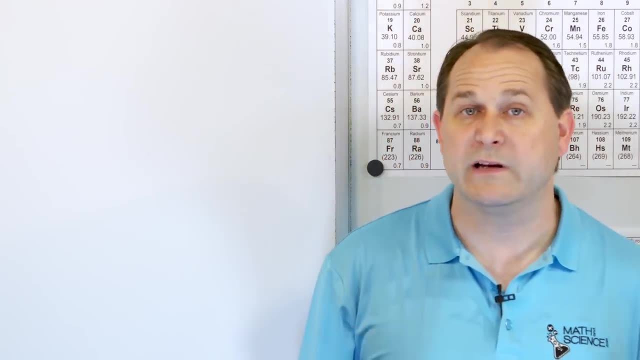 interesting thing is is: this gas is non-reactive, This one's non-reactive, This one's non-reactive And also this one's non-reactive. And what I mean by non-reactive is they don't participate really in any chemical reactions, right, And that is true. I'm going to boil it down and show you how this 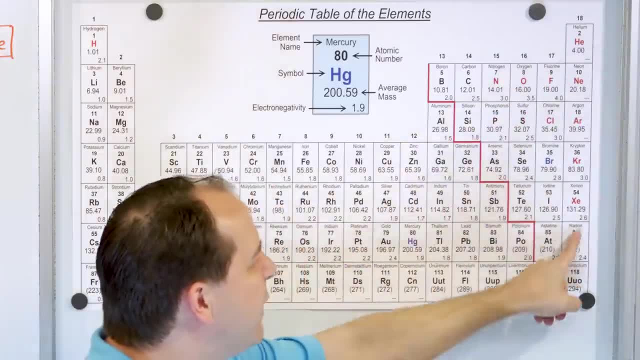 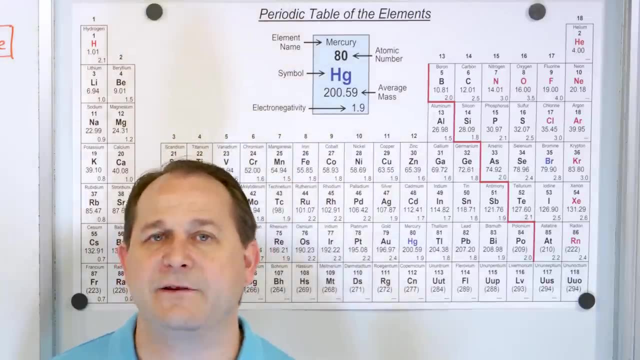 occurs in a minute, But basically everything in the right hand column. we call these the noble gases. They're noble, right? They don't? they're kind of like cheap to themselves. They don't participate in chemistry. They don't make any anything in a chemical reaction. You can try to. 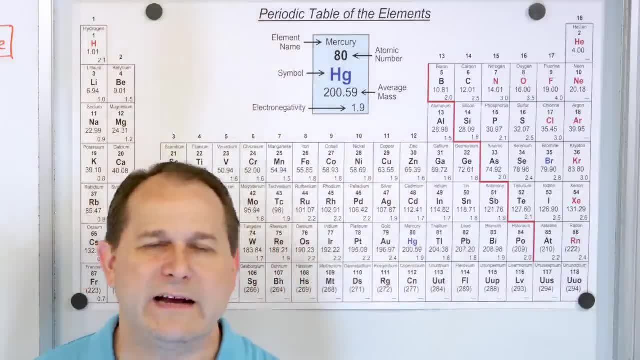 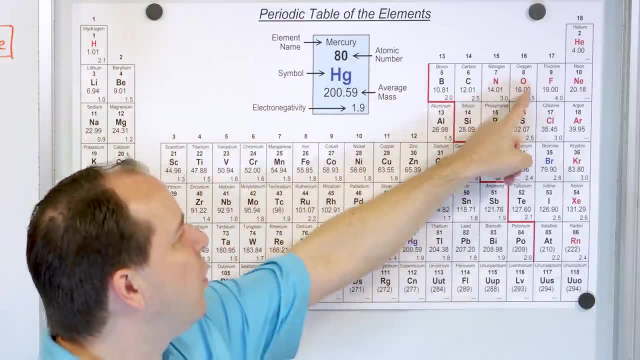 put whatever you want next to argon And, with very few exceptions, it's not going to bond with anything. Like you know, water, right, Is H2O, So two hydrogens and one oxygen. So they bond together and they make a molecule and you can drink it and you can cook with it and all of this. 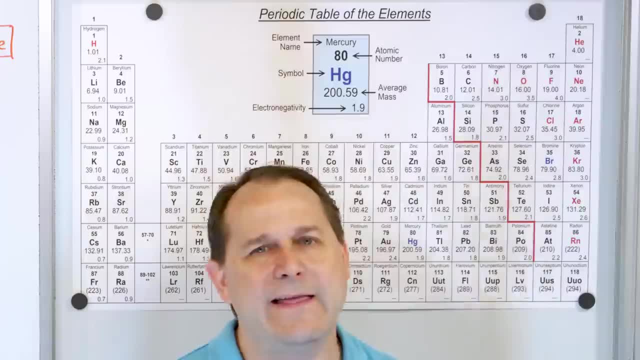 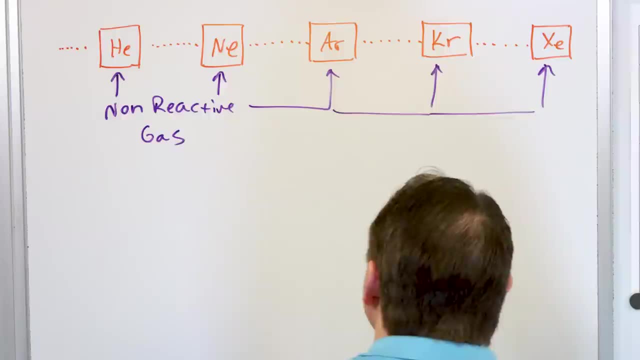 but you really cannot make these things react with anything, And that's a curious thing. But then people realize- even more interesting than that is the fact that whenever you look at these special gases, first of all they're all gases that are non-reactive. Okay, And then what you? 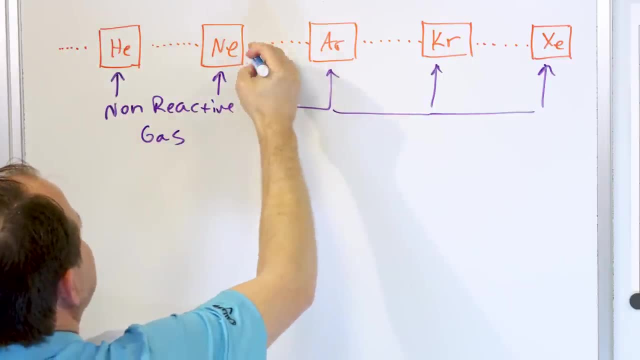 really look at is that the. the element that comes right after the non-reactive gas is the element that comes right after. uh, if again, when you're increasing atomic number, the element that comes right after each one of these is a very, very reactive soft metal. So I'll go down. 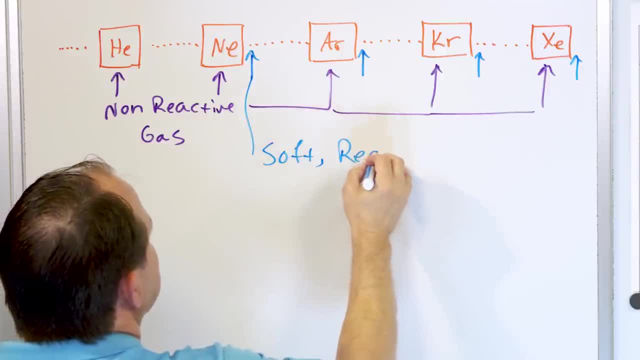 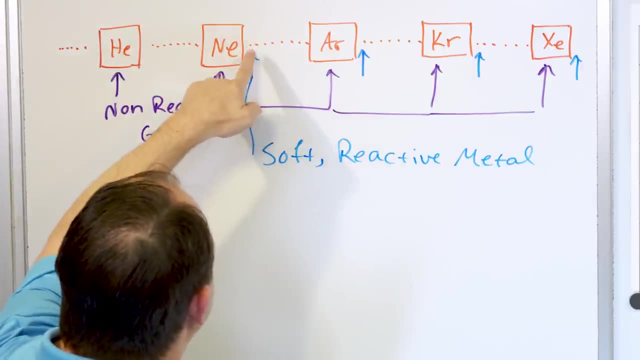 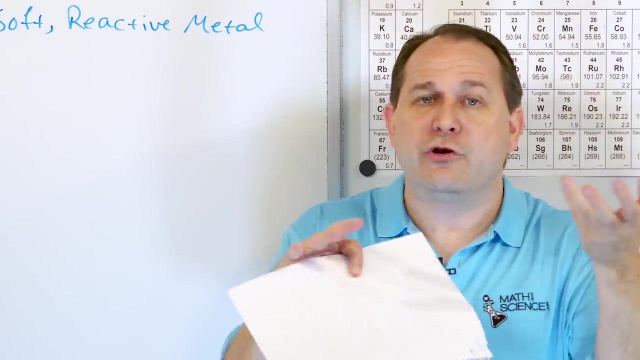 here Soft reactive metal, right Every every time. So so right after neon is a soft reactive metal. And what I mean by reactive is it reacts with lots of things. It reacts with oxygen, Maybe it reacts with water, And it just. you can just tell that chemistry is happening, Chemistry is. 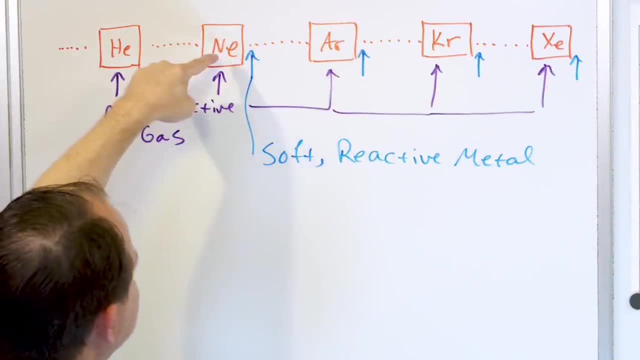 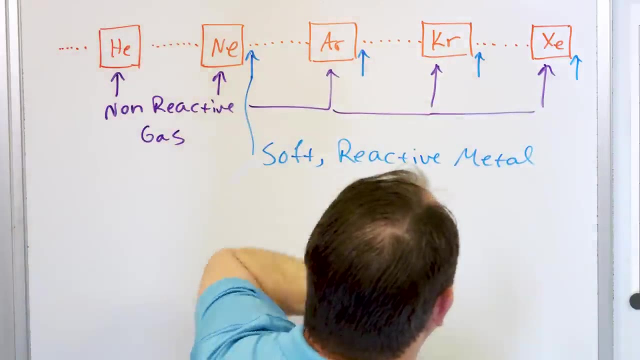 happening, And it happens, It seems to happen Like they have these perfect gases that don't do anything And then right next door you have a very, very reactive metal. Okay, It increasing as you go, increasing atomic number, And then also on the previous side, like over on on this side. 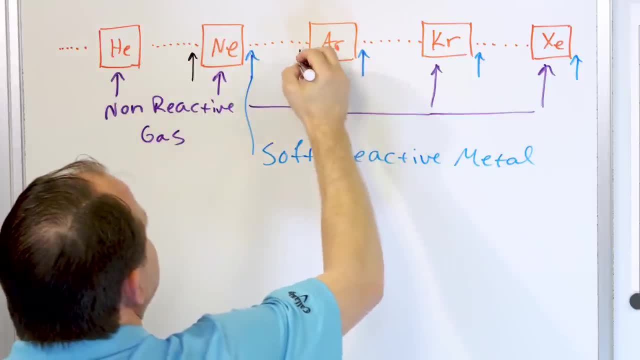 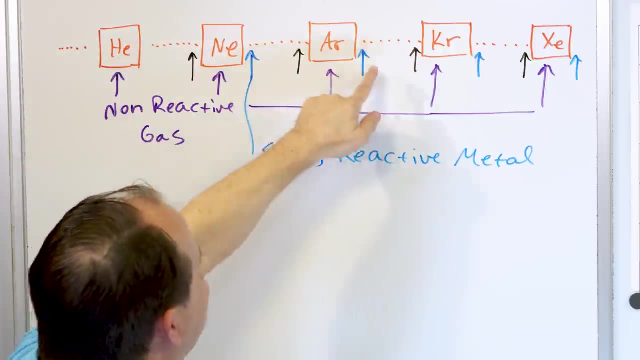 over here. I guess I'll use this color. There's an interesting little thing right here is that you, uh uh, you have in general, in general, a gas over here that is a reactive gas, All right, right before. So you see, you can just see that there is some periodic nature. 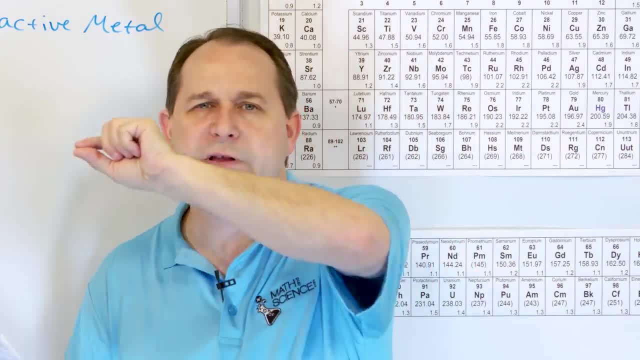 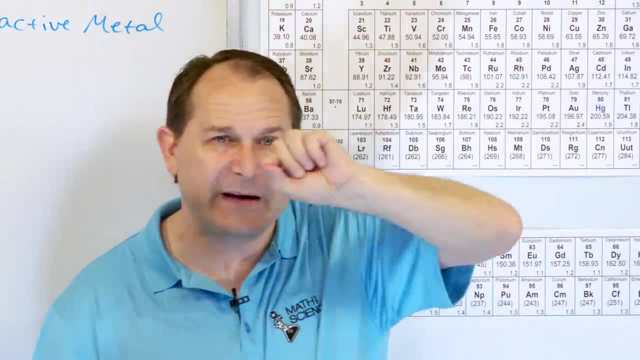 to what's going on, because when you take all the elements that you discover and you put them in order, forget about the table. you just write them in a straight line from beginning to end. There's a hundred and some odd elements here. You put them from beginning to end. What you're? 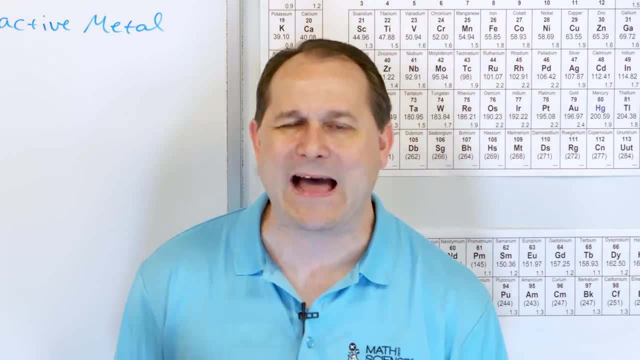 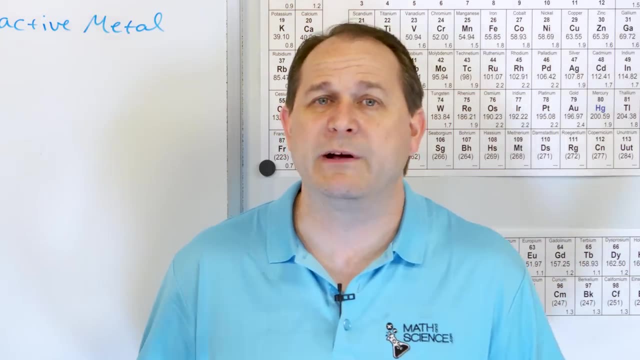 going to notice is that there's some kind of some kind of regular repeating patterns here. There are these special ones, these special elements which we now call the noble gases, which don't do any chemistry at all. no matter how much you want it to happen, it won't happen. 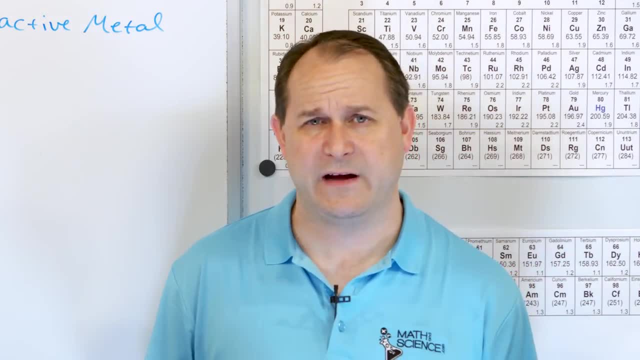 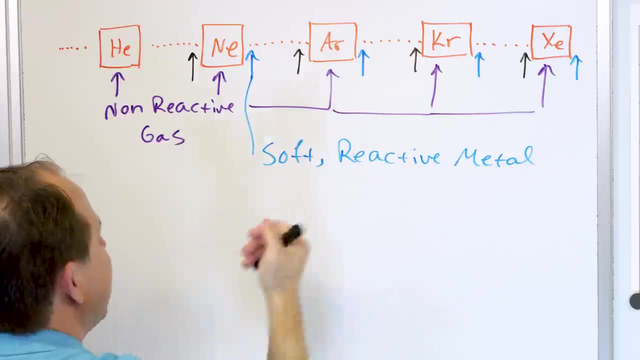 But then on either side of the noble gases they're extremely reactive elements And it always happens that the element of the noble gases, which we now call the noble gases, which don't do any chemistry at all, just after the gas is a metal that's soft and very, very reactive And just 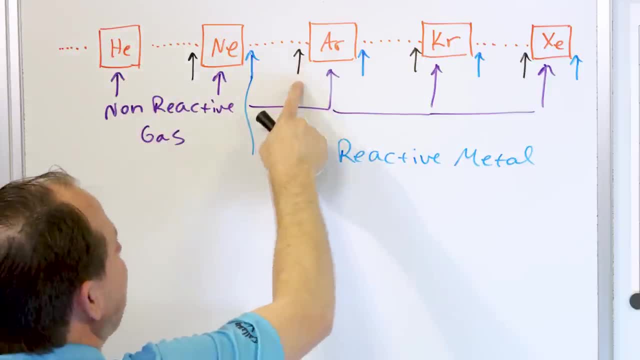 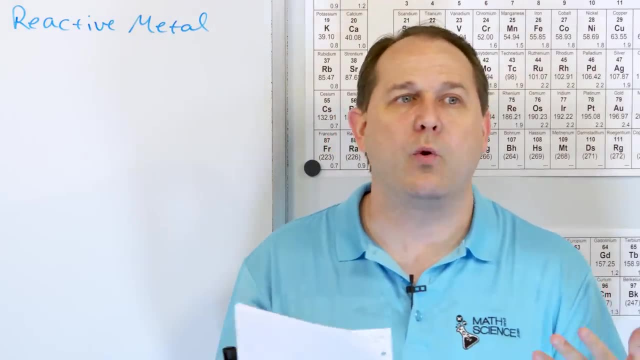 before the gas is a gas, another gas which is also quite reactive. All right, So this is what happens when you put them in a line. So people start playing with this table and trying to figure out- what does it mean and why do they behave this way? And eventually, after a lot of different, 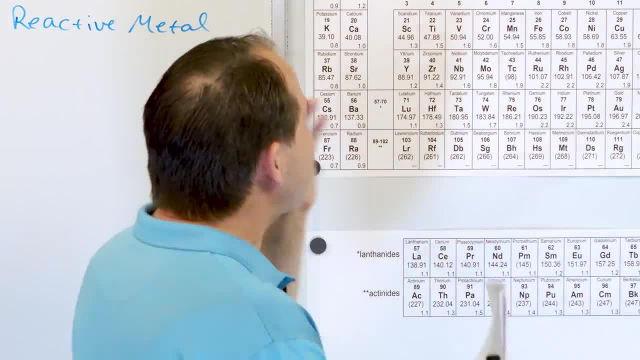 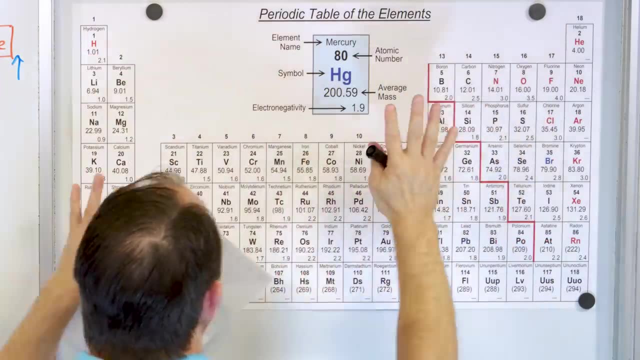 scientists, they come up with the formulation of the periodic table. So now, knowing the periodic nature of what it is, let's look over here. Well, the way we've arranged this is increasing atomic number, but of course the table looks weird. There's a big gap. 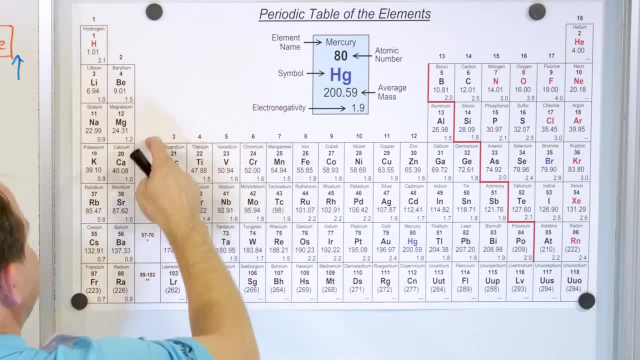 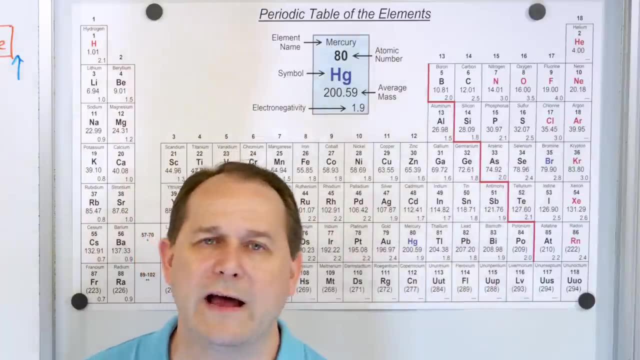 right here. This is not lined. There's a big gap here. There's a gap right here. It doesn't look like a nice square table, And I'm going to tell you right now that the reason it's laid out the way it is, it all has to do with how the electrons around all of these atoms are actually set up. 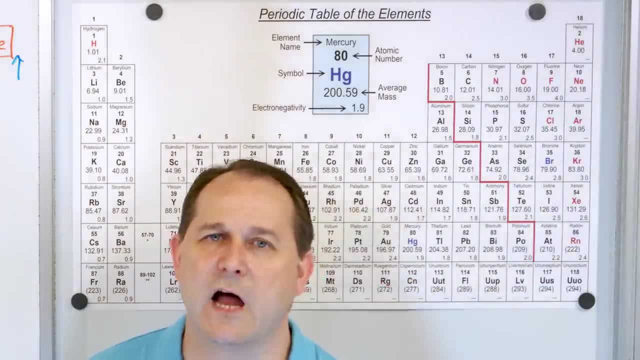 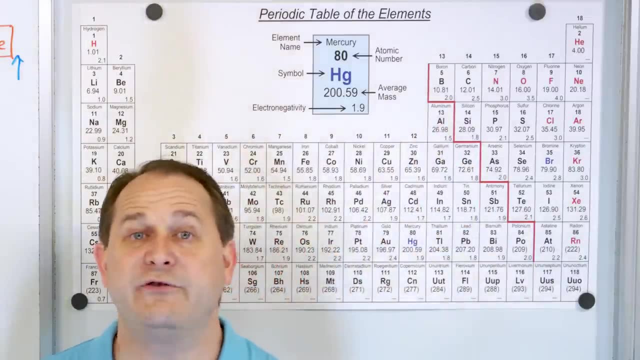 how they're actually orbiting there. We're going to get to that a lot later, So we can't do too many things at once. I cannot tell you the electron structure around aluminum right now. it's going to be too much at once, but you're just going to have to trust me that the way that 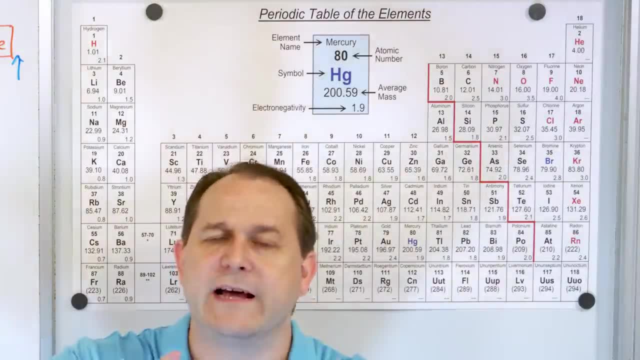 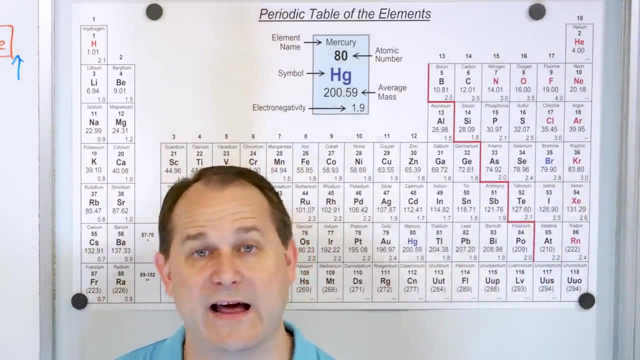 this table is laid out the way that the that it looks. it comes directly from how the electrons fill in to the orbitals that surround all of the atoms. We're going to get into that in a great detail a lot later, but if you notice, here is helium. it's one of these noble gases. 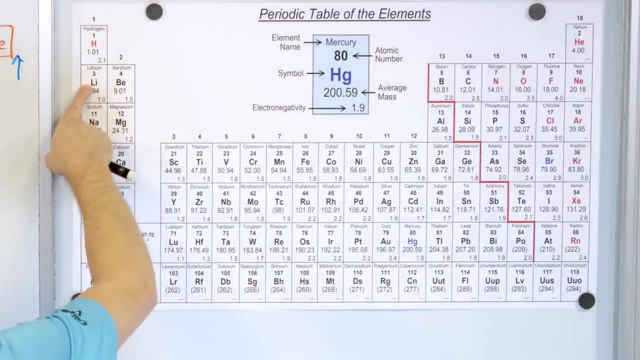 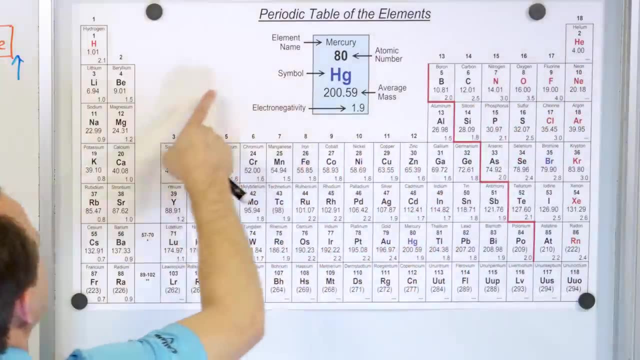 And just after that is lithium, which actually is a very highly reactive soft metal. And then you keep going over here and you get to neon And right after neon, remember, should be a soft reactive metal which is sodium. That's a soft reactive metal. 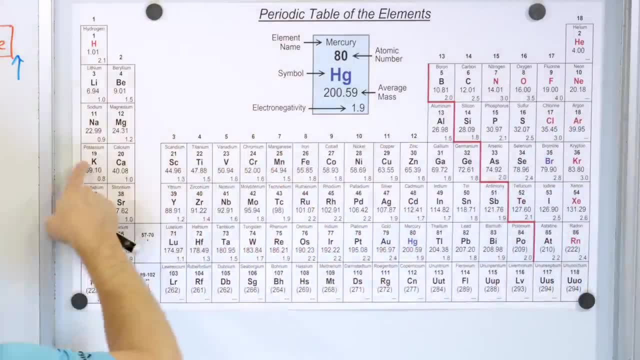 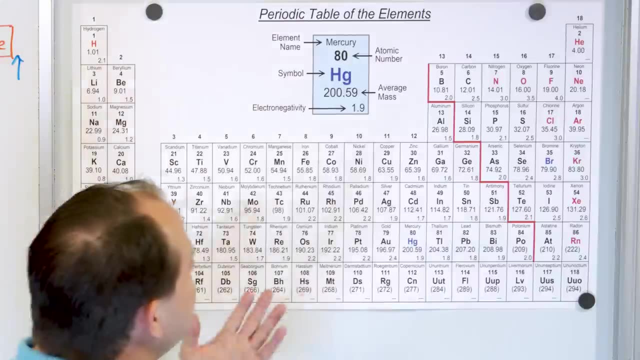 And then when you get to argon, right after that one, because this is non-reactive, you get to potassium, another very soft reactive metal, And after krypton you get to rubidium and the same kind of behavior. And then also we said, remember, after the noble gas comes a soft. 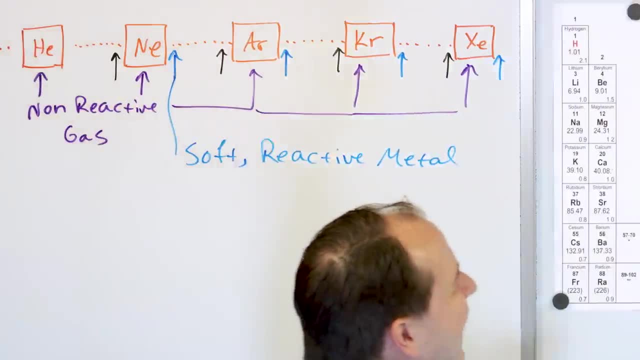 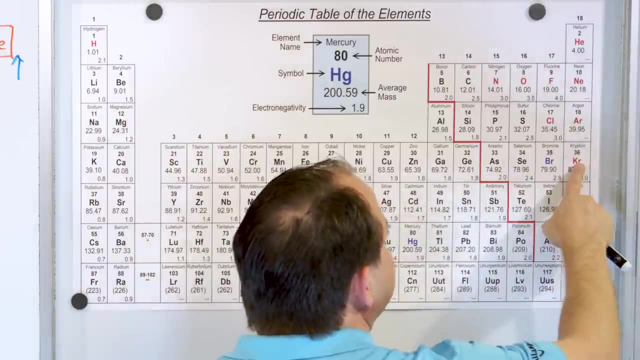 reactive metal and before is in general a very reactive gas. So here in front of neon, we have fluorine, very reactive gas. In front of argon, we have chlorine, very reactive gas In front of krypton. now this is not a gas, Bromine is not a gas. So there's some exceptions here. They're. 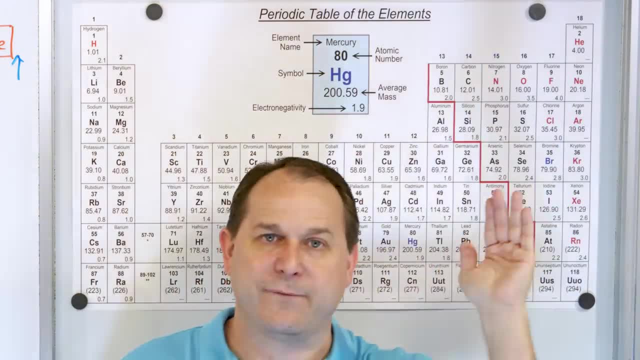 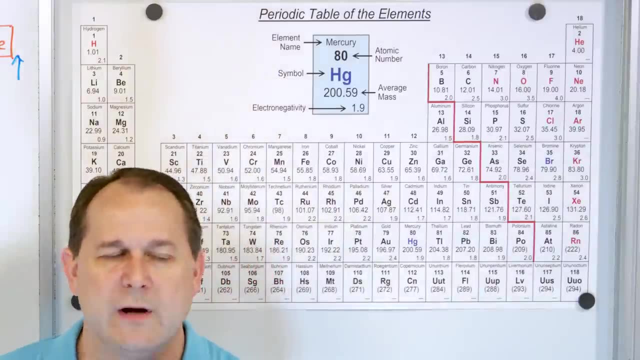 not always gases that are on the right, before the noble gases, but it's often the case. So it's enough to convince you that there's some periodic nature. Now let me give you a clue, because we can't study it in detail in this introductory lesson. 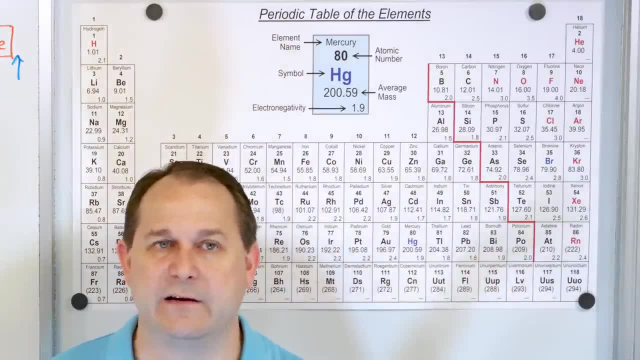 The reason why there's periodic structure to the atoms in nature, the reason why we see these patterns is because the way the electrons fill in all of the orbits around the nucleus, it follows a regular repeating pattern. That's the reason why. Now, of course, 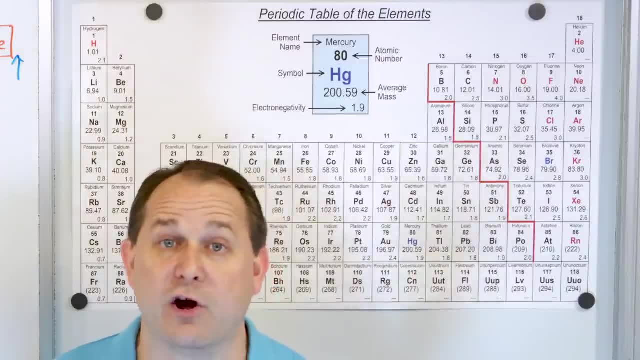 in the beginning, when they made the periodic table, they didn't know about electrons at all. They hadn't even been discovered yet. That's what's amazing: They put this table together without even knowing what the atom was. Okay, They also didn't know about protons and neutrons. 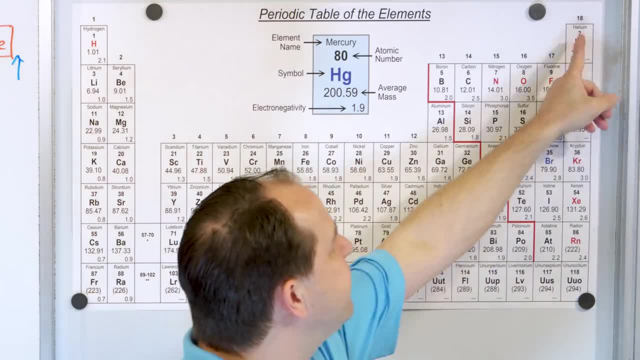 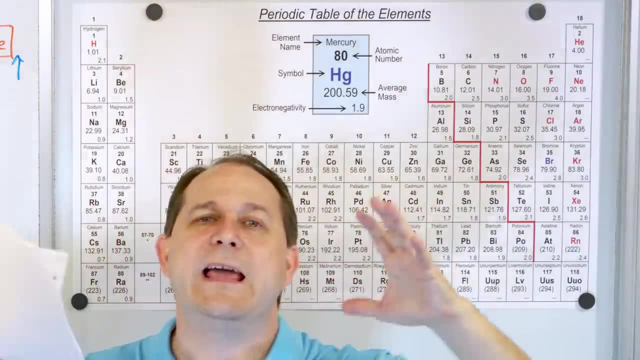 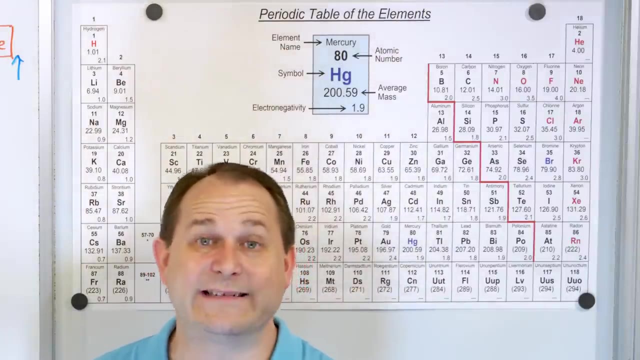 either. But now we know that the reason why all of these noble gases are very unreactive is because they have the very same electron configuration in their outermost shells, which are all very similar. Now what do I mean by very similar? I have to save that for another lesson, because it 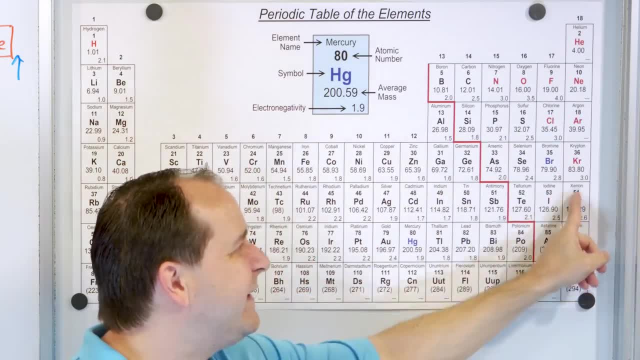 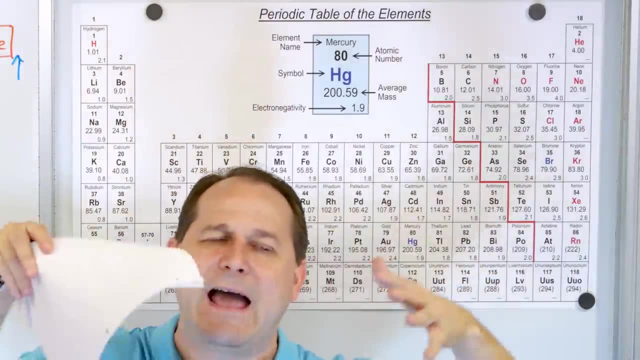 goes into some details, but every one of these have a very similar outermost shell. Okay, Outermost shell, We're going to talk about what shells are, but basically the electrons. you can't just pile them in, They have to occupy certain states around the atom and 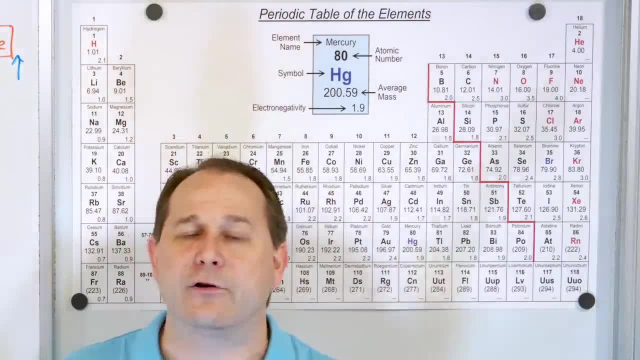 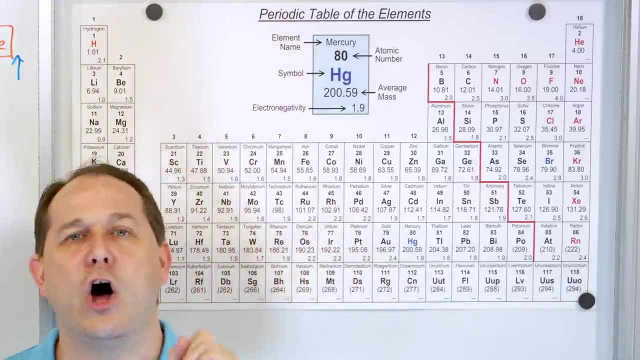 they're organized into shells and other things, And so the outermost electrons of all of those are extremely stable, And that is why they don't like to react with anything, because they don't want to move. All chemistry, chemical reactions, basically centers around how do the 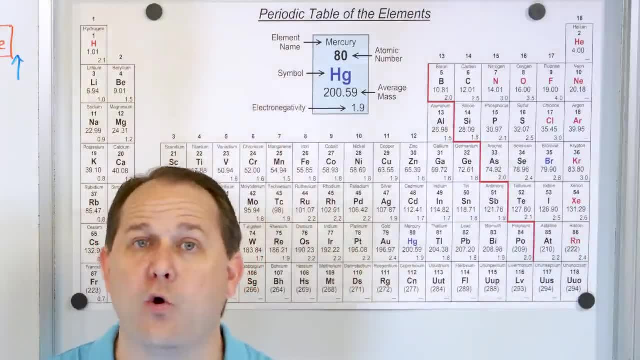 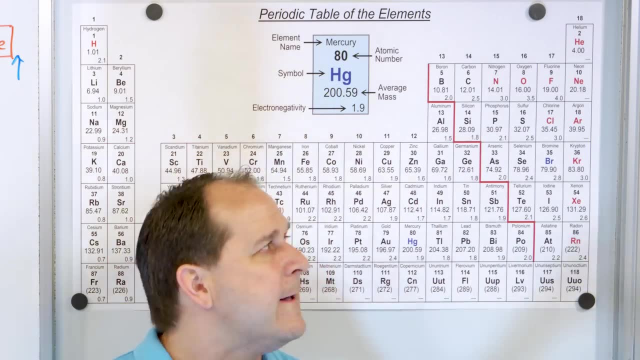 electrons move around. When you have a reaction, you have an electron sharing or an electron transfer taking place, and then the atoms can rearrange themselves And then you have something new, the product of the reaction, But in here because the electrons are all extremely stable. 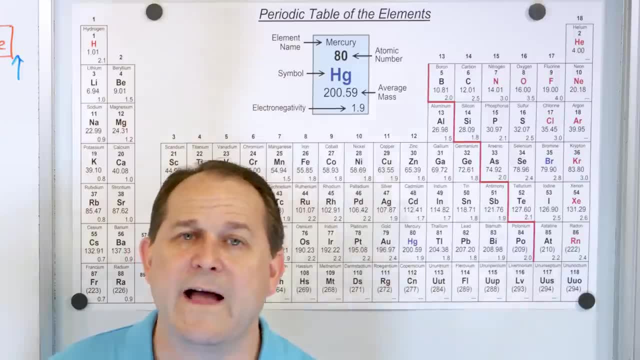 around all those atoms. they don't want to react with anything because the electrons don't want to move, And that is why the noble gases don't react. All right, So we said that we had the noble gases in the right-hand part of the table. 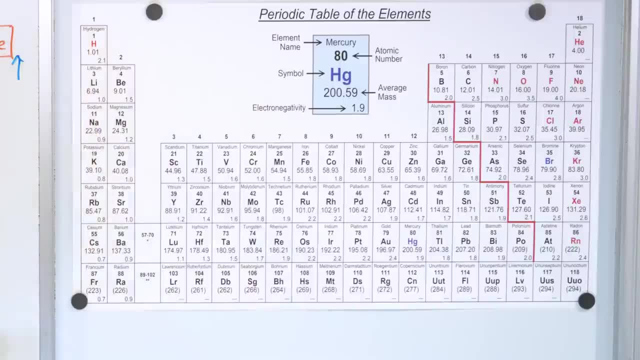 Okay, All right. So we said that we had the noble gases in the right-hand part of the table. We're going to talk about what it means later. We said that just after the noble gases, we had a very reactive column here of very reactive metals And then we talked about in every one of these squares. 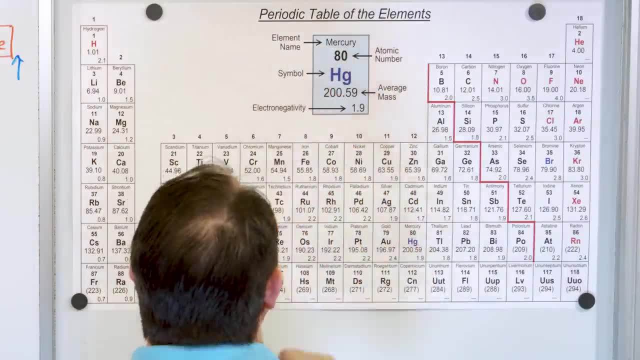 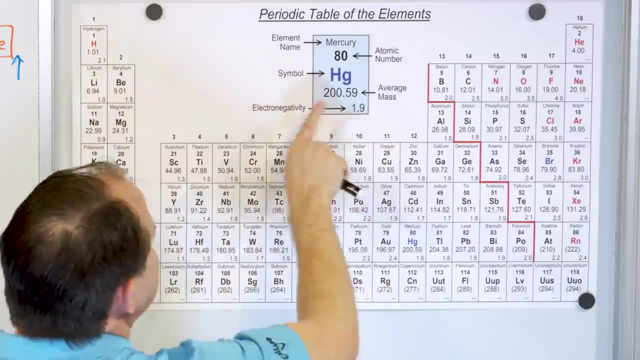 we have an atomic symbol and atomic number, which is number of protons and the atomic mass, And, depending on the table that you have, you might have other information in here. This table also has something called the electronegativity. We're going to talk. 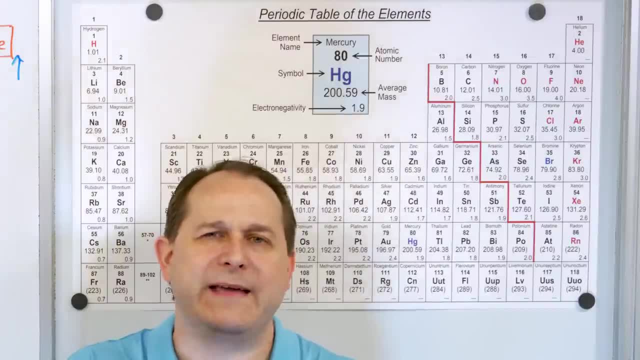 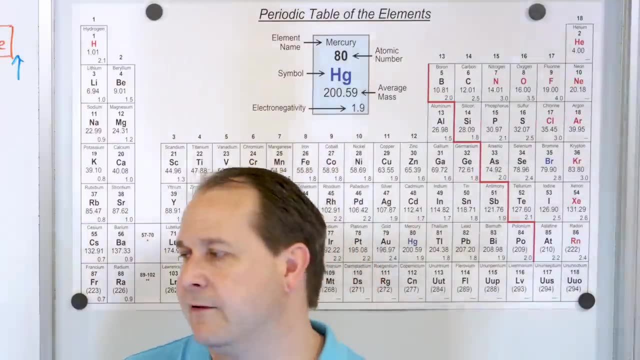 about what it means later, Don't worry about it now. It has to do with how the atom attracts electrons. Okay, But you could have all kinds of things in different periodic tables. You might put the melting point of the substance or the boiling point of the substance. 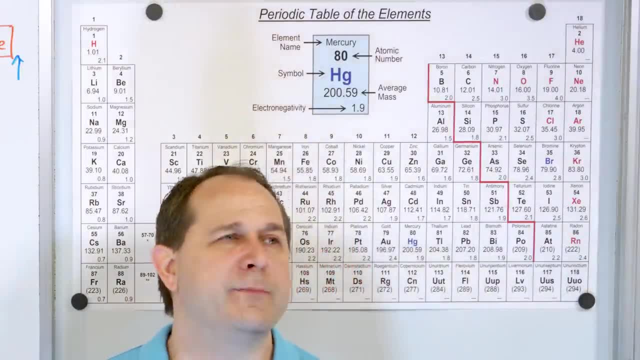 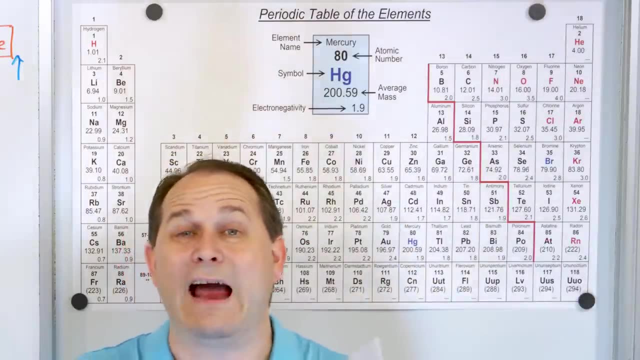 or what kind of a crystal structure the substance has. or you might put you know like this one has electronegativity. You could have all kinds of things in periodic tables, but the most important things, the ones you'll see everywhere, is: you'll see the symbol. 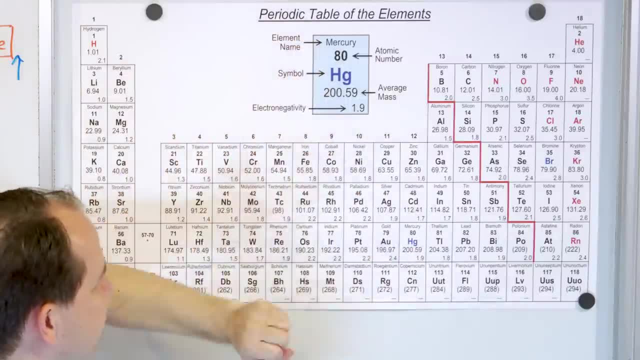 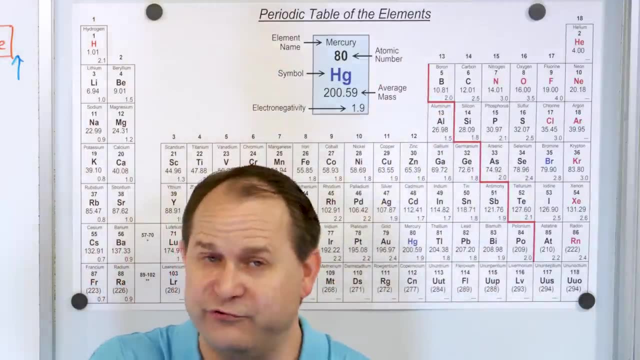 You'll see the atomic number and you'll see the atomic mass. Anything else is just. you may or may not see that. That's the core of the periodic table. Now, before we go any further, we've told you that, I've told you that there's a periodic nature And I've told 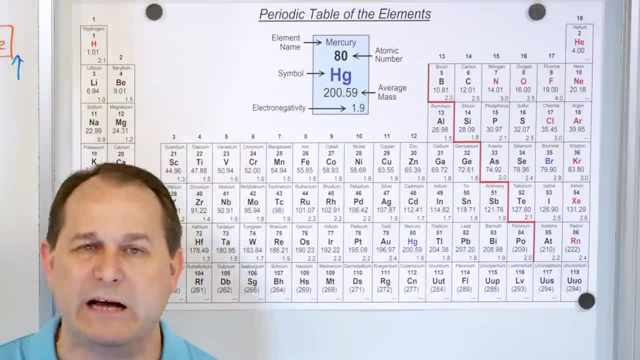 you the reason why there's a periodic nature in some of the properties. It's because of how the electrons are situated around these atoms. Now I need to give you more definitions. I'm not going to write these definitions down because it'll be a waste of my time and your time. 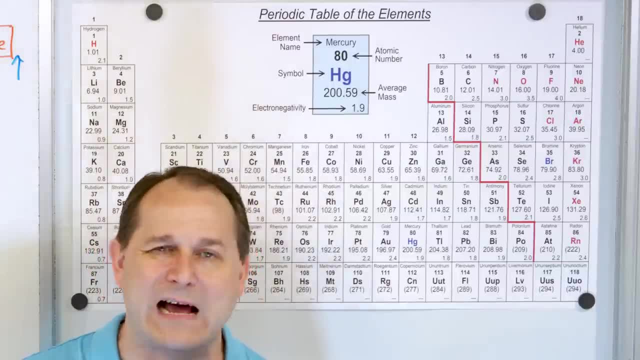 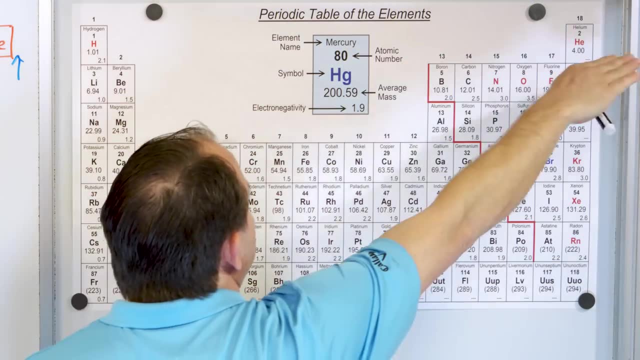 but I will tell you and I encourage you to watch it several times to make sure they sink in. They're not hard, but we have to talk about them. So this periodic table consists of rows over here and columns, which are here. Okay, But we don't call the rows and columns, We actually call the. 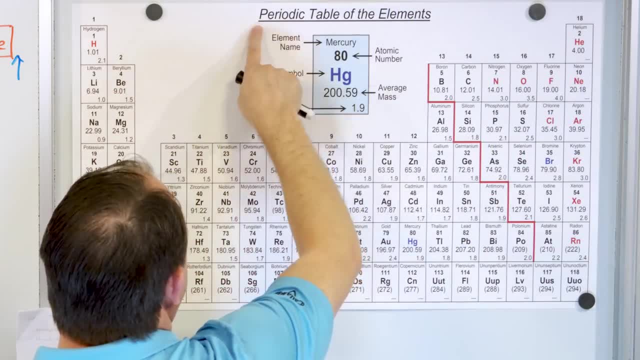 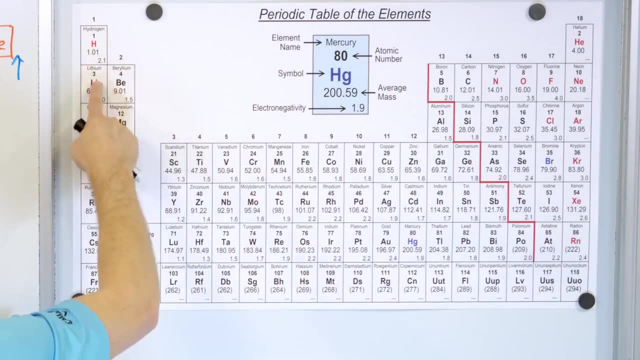 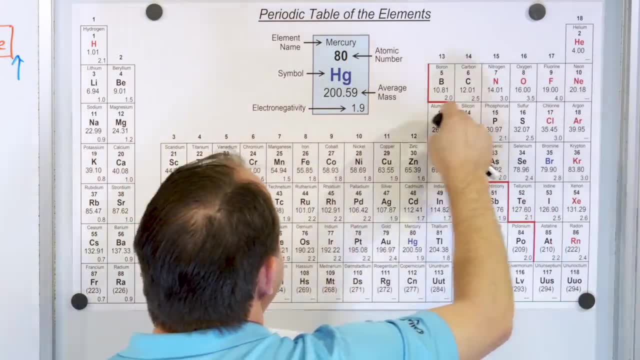 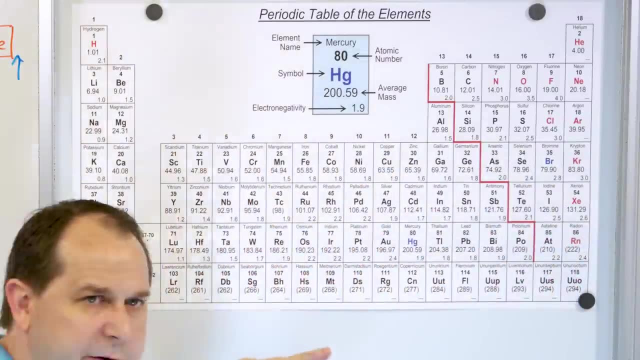 being connected to the right side, sort of You draw your finger all the way across. This is period number three, period four. This is period five, This is period six, And this one down here is period number seven. So the periods go across Periodic period. Okay, Now the columns. we don't. 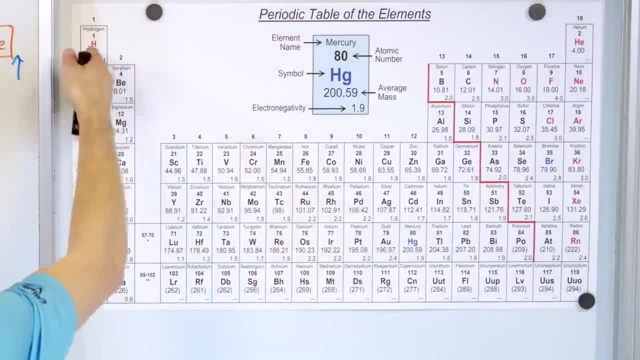 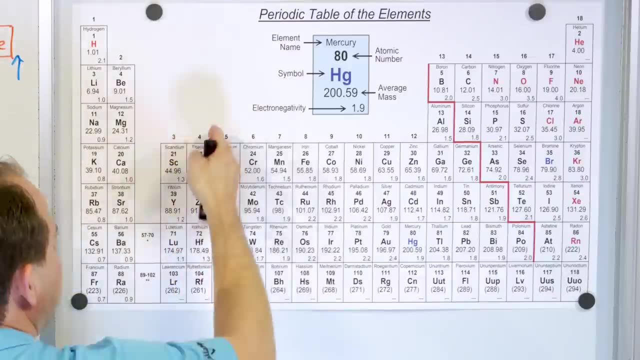 call them columns, We call them groups. So this is a group. See, it's labeled at the top: group number one. This is a group. It's called group number two. This is group three, group four, And you can see that every you have a nice little. 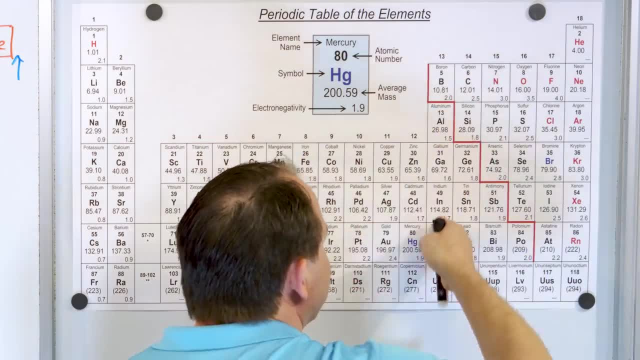 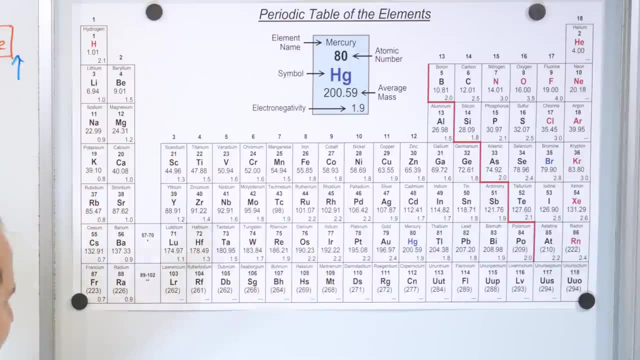 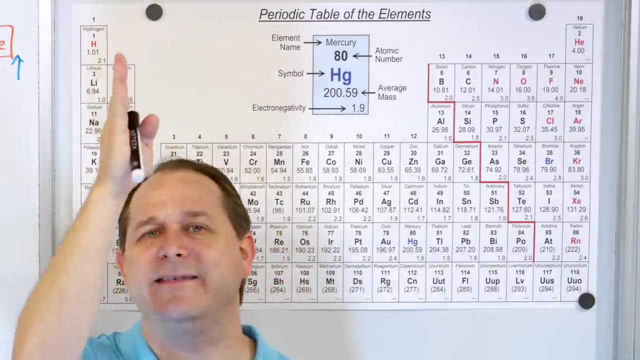 vertical nature to it. We have the groups, and then we have group number 13,, group number 14,, group number 15,, 16,, 17, and 18.. All right, Now the interesting thing about the groups is that the groups, one of the main reasons why we use the periodic table, is because the elements 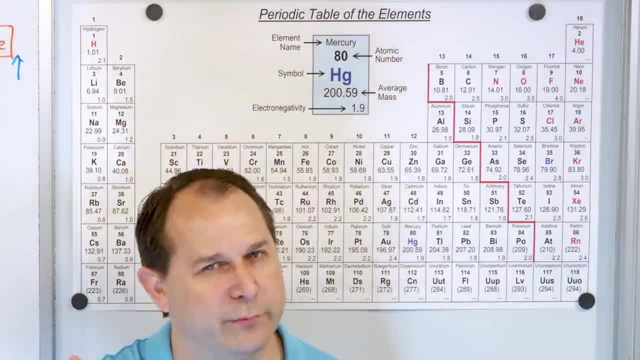 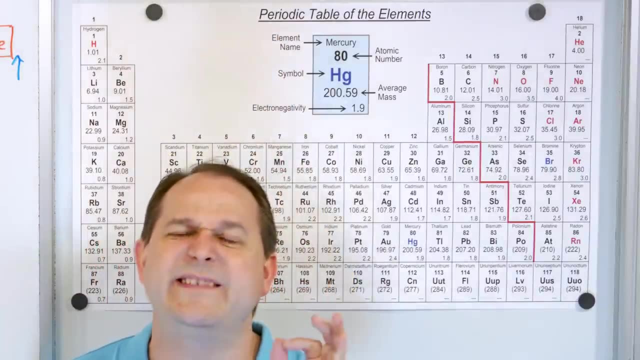 that are in the same group, which is the same column. Remember, column means group. Elements that are in the same column have similar properties. I'm going to say that again: Elements that are in the same group have similar properties. I'm going to say that a third time. 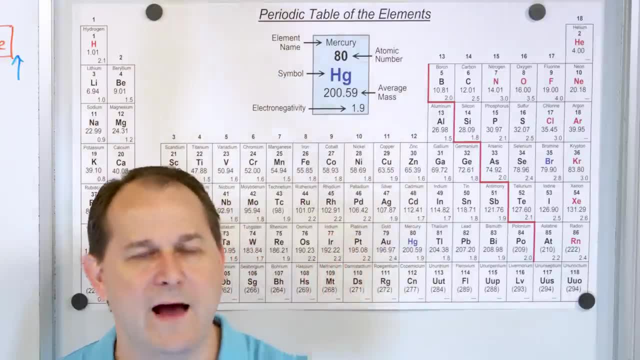 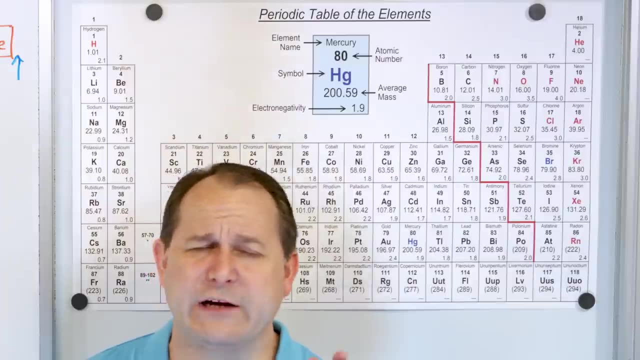 Elements in the same group have similar properties. A fourth time, elements in the same group, up and down, have the same or similar properties. That's critically important to you, Critically critically important to you. In fact, it's one of the most useful things on this table. 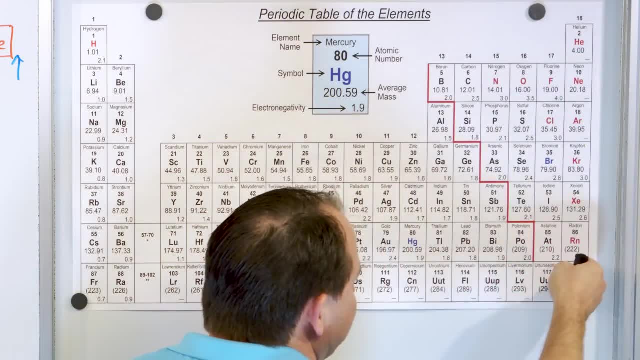 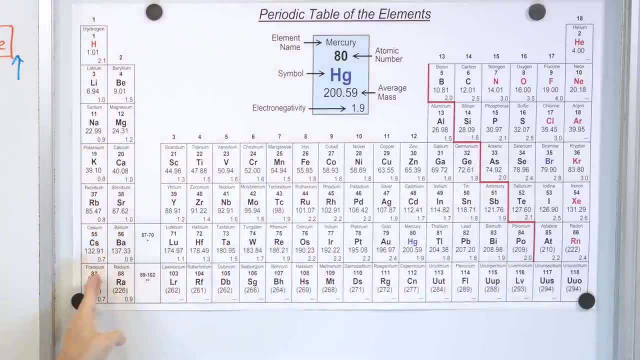 because you can see right away that these must have similar properties. And what is that property It? they're non-regulatory, They're non-reactive gases. Okay, That's a big one. These have a similar property in group one right here: They are extremely reactive metals. but let me come back to hydrogen, because hydrogen 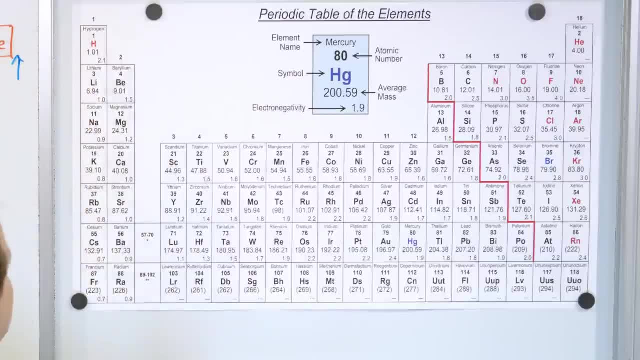 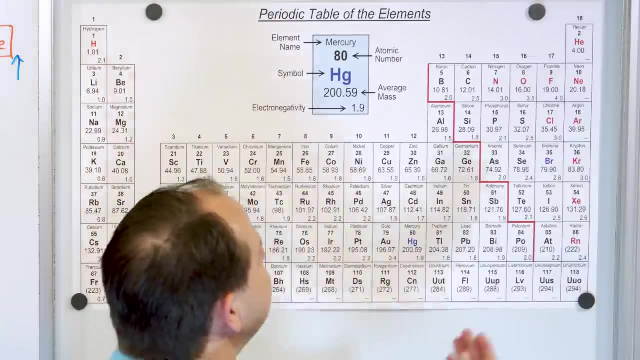 is a little bit of a weirdo. Obviously it's not a metal, but everything else is an extremely reactive metal. These are also extremely reactive metals, but not quite as reactive as these right Now when you go to this side of the table. these have similar properties. They're mostly 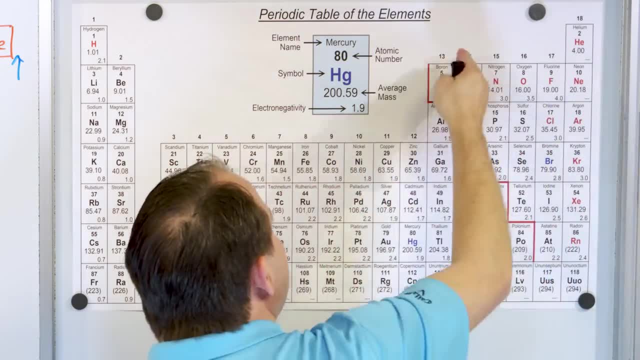 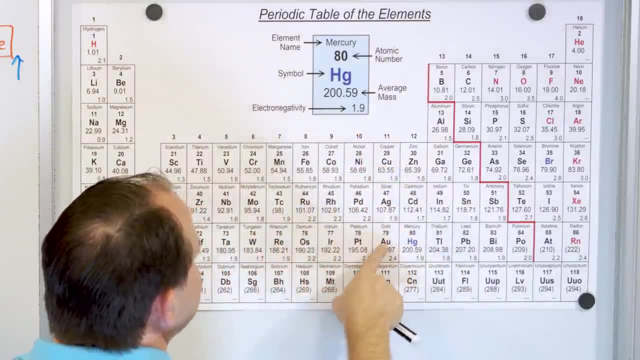 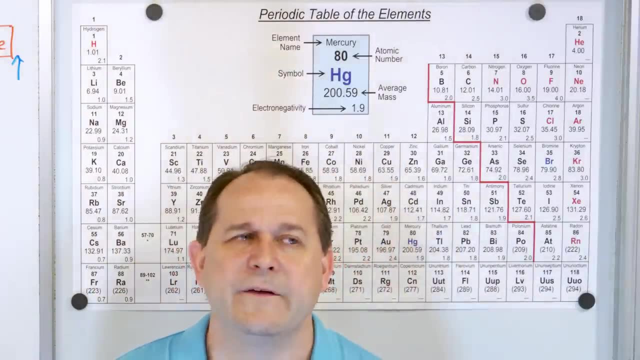 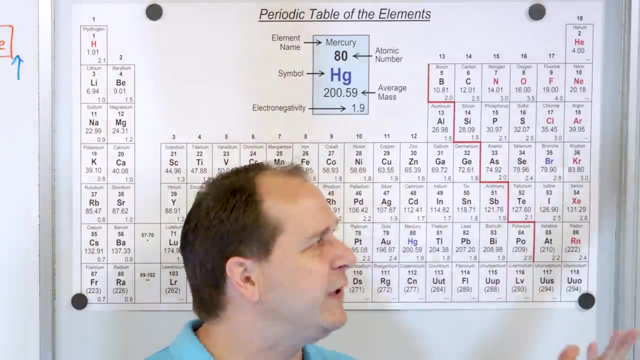 because in this column you have copper, you have silver and you have gold. Copper, silver, gold are basically what we have used over the years to make all of our currency, So sometimes we call it the currency group right- And the reason why we use these particular elements. why don't we use 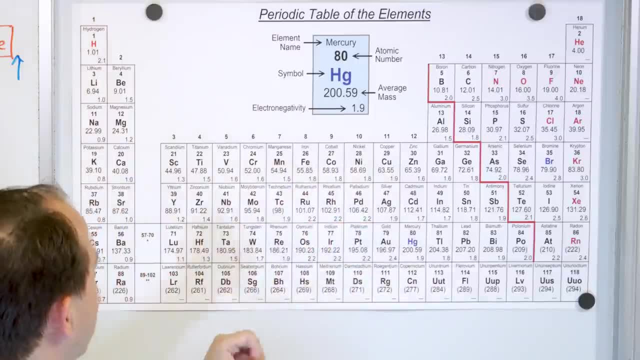 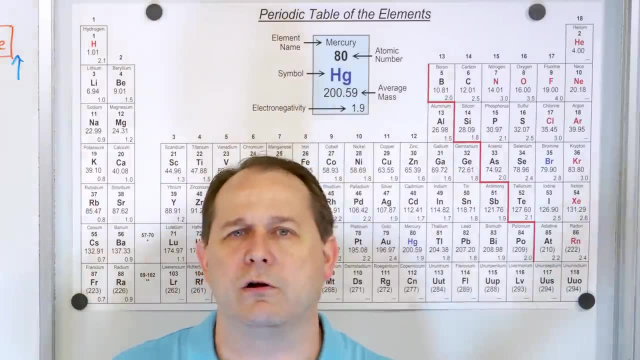 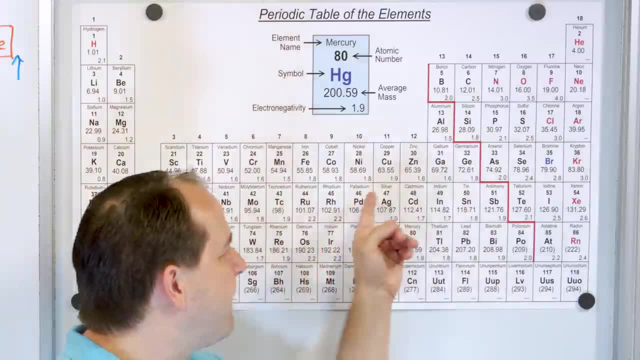 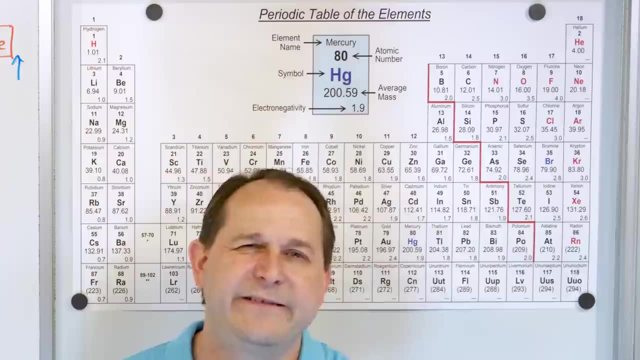 they don't all exist in the same abundance on earth, okay, But copper, gold and silver are in reasonable, reasonably high abundance on earth and they're relatively non-reactive. as far as metals go, I mean silver does tarnish a little bit. It turns like a little little grayish after. 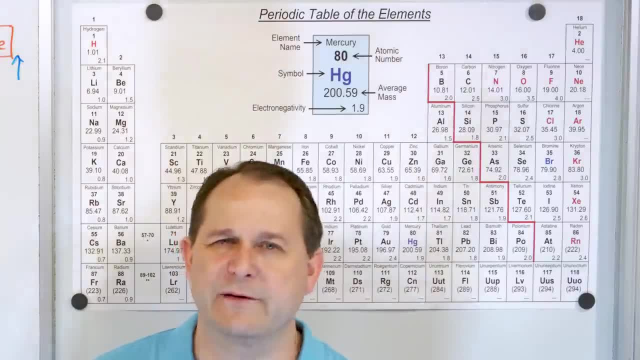 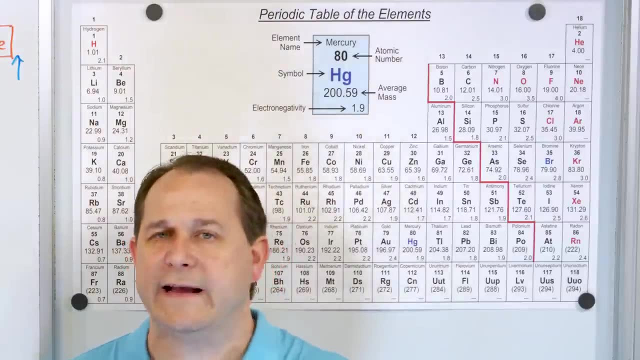 a while It does tarnish. but gold and copper- I mean there's a little bit of copper- reacts a little bit too, but in general, compared to other metals, they don't react as much and they're very strong and they last a long time. and we can, we can stamp them, We can also pull them. That lets. 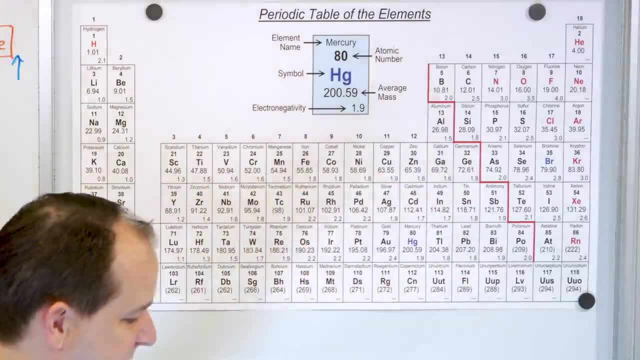 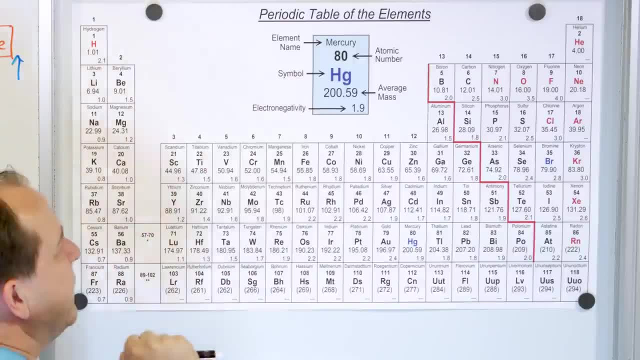 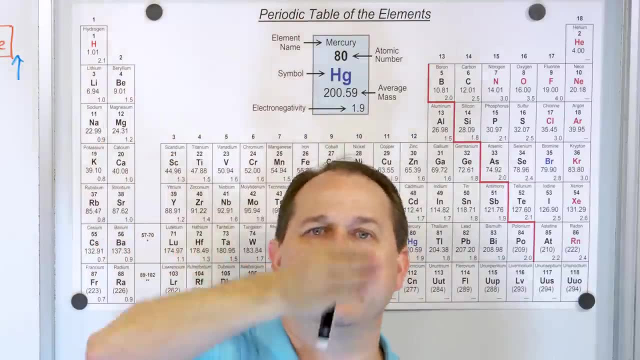 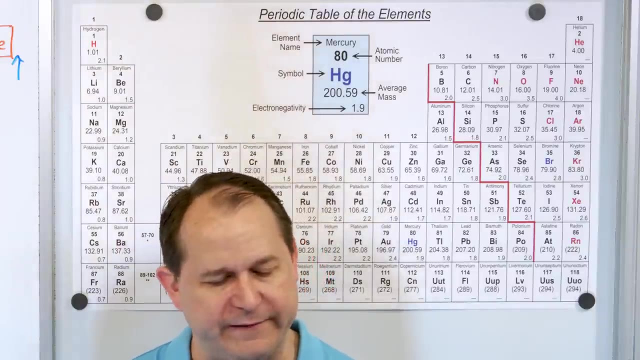 I'd like to do is tell you at this point, other than the idea of periods, which are rows, and groups, which are columns, and I want you to know, that the elements in the different groups have similar properties, one of the absolute, absolute, most important things that you have to understand. 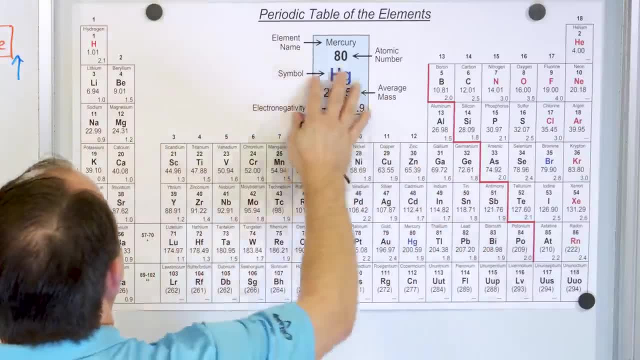 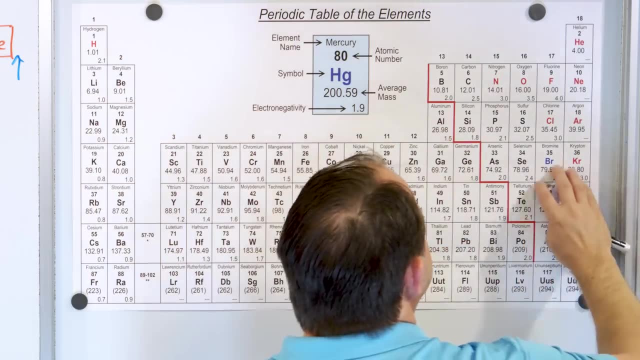 here is that the left-hand side of the table, the entire left-hand side of the table, is, in general, metals. in general, metals on the left-hand side, On the right-hand side of the table, is, in general, non-metals- over here and in the middle. 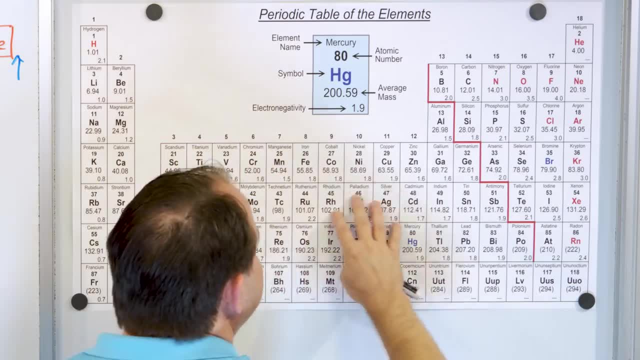 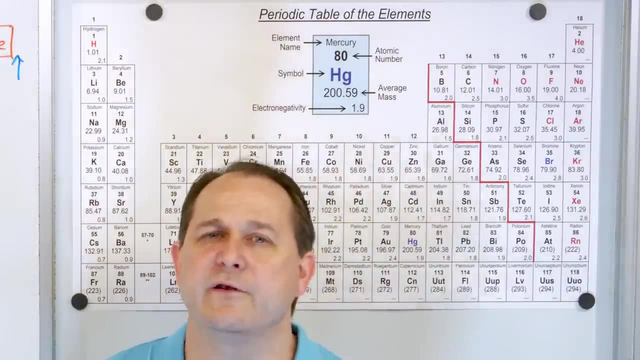 what we have here down here, set down, set below. we call these the transition metals here, and we're going to learn a lot more about why they're called these different things a little bit later. This is an overview lesson, but if you just take a look, notice that there's this: 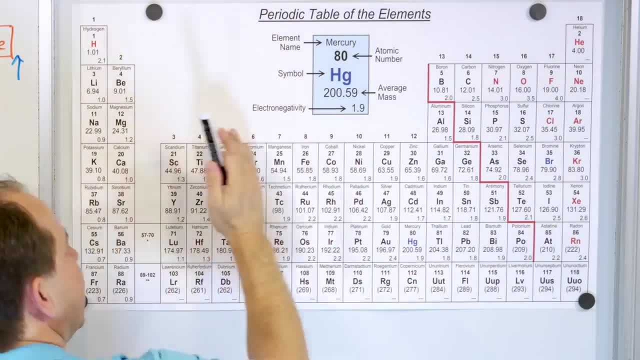 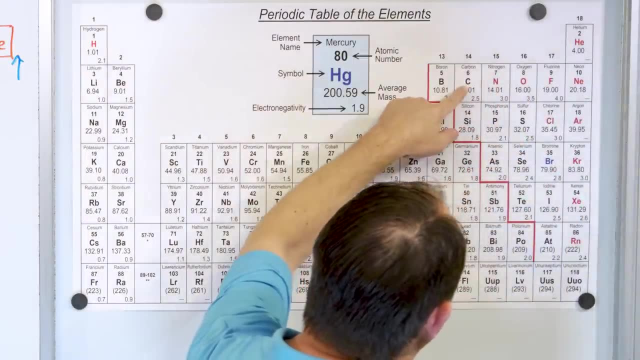 stair-step line right here. It kind of divides the table from a left-hand side to a right-hand side, everything to the right. you might guess that it's a non-metal. I mean chlorine, oxygen, nitrogen, carbon. carbon is definitely not a metal. and then you have all these gases like 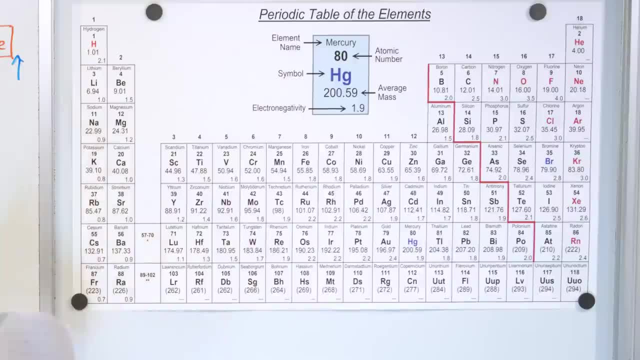 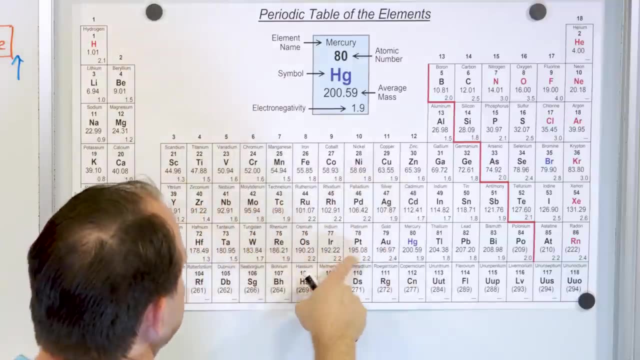 neon and helium and things like this, and then over on the left-hand side are the things that you might think of as metals. You have your copper, your zinc, your nickel, your titanium, some of these others you may not know about as much. you know you have rhenium and gold. 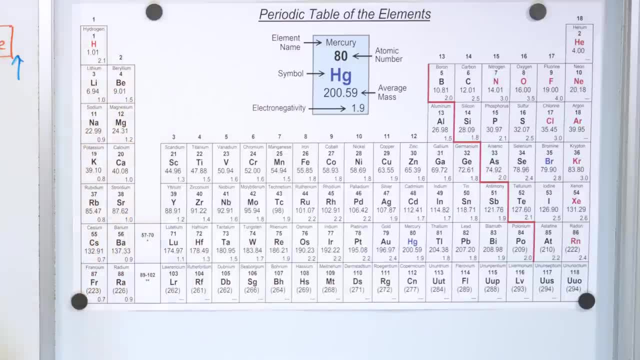 and mercury and platinum, and then over here these are metals as well, but we don't, you know, see them much every day because they're so reactive. They're usually already combined with oxygen, like here you have sodium and lithium. Now 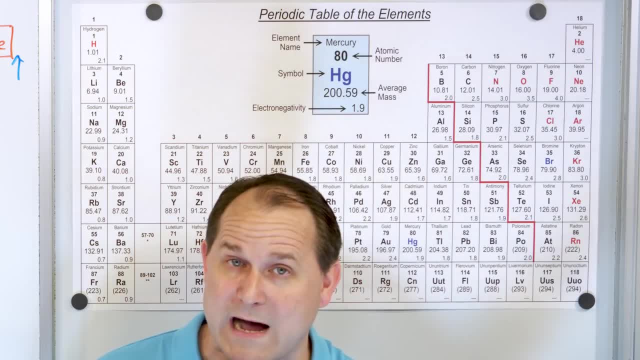 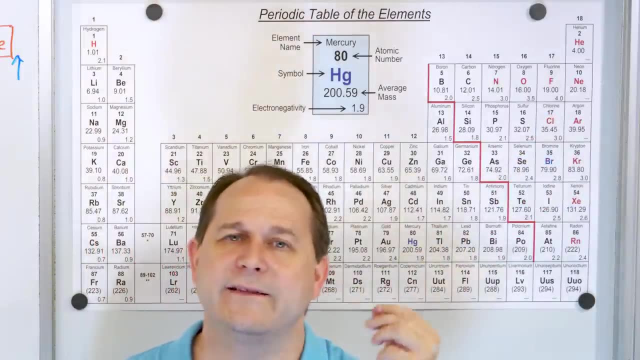 you actually eat sodium every day, because sodium chloride, which is an atom of sodium combined with an atom of chlorine, makes something new called sodium chloride and that is table salt. So these things you have experience with, you just may not know that table salt is sodium chloride. 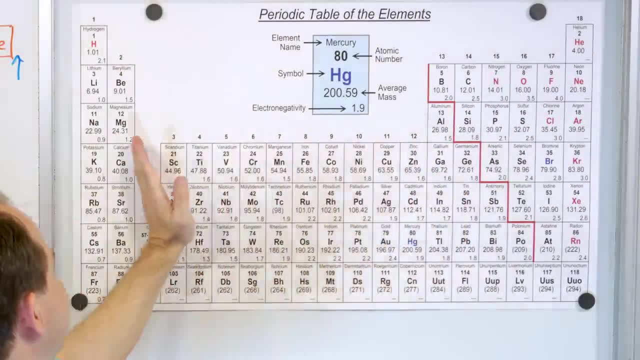 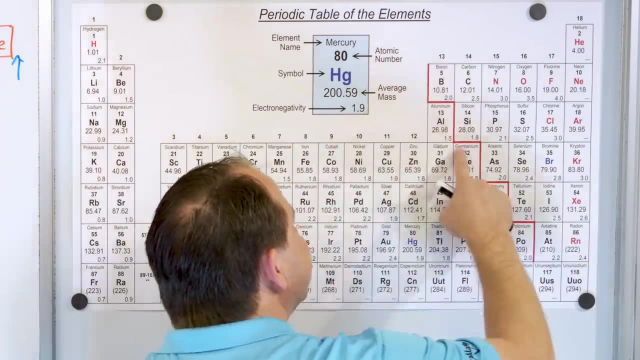 okay. So anyway, the left-hand side of the table are the things that you typically consider to be metals, and the right-hand side of the table are things that you typically consider to be non-metals, and right around this stair-step line is the border between the two, and so the 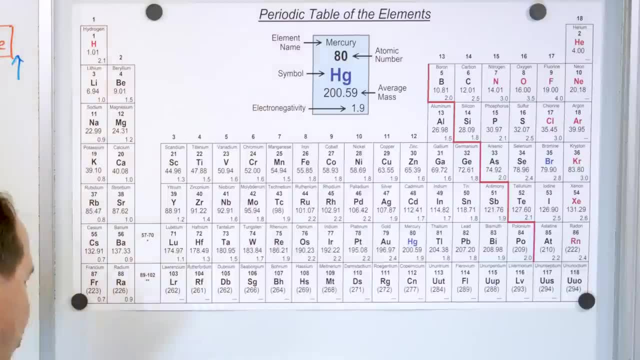 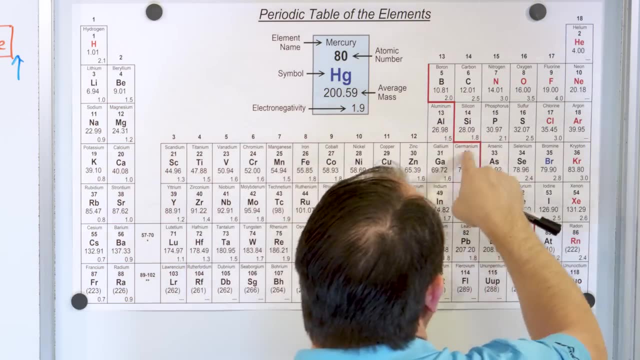 elements that are right on the border. we typically call those metaloids. We call them metaloids, all right, And you know germanium and silicon are probably the most important ones, but boron and some of these other ones on the border here. So silicon is probably the one you've heard of. 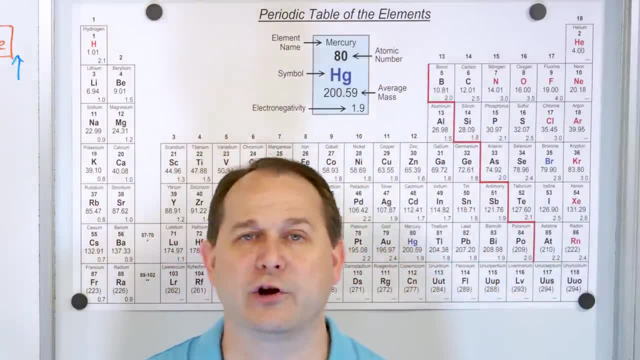 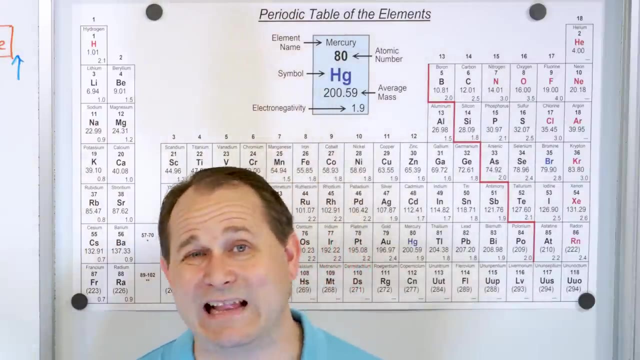 the most Silicon, is extremely important for making all of our computer chips. Imagine the world without computer chips, And when I mean computer chips, I mean any kind of chip, any kind of transistor, which is what we make our radios out of. So you have no radios, no phones, no televisions, no internet, no satellites. 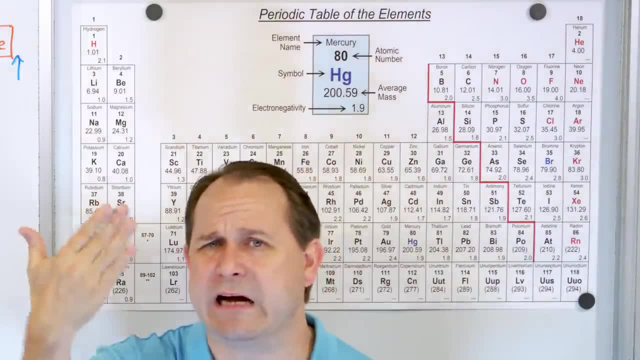 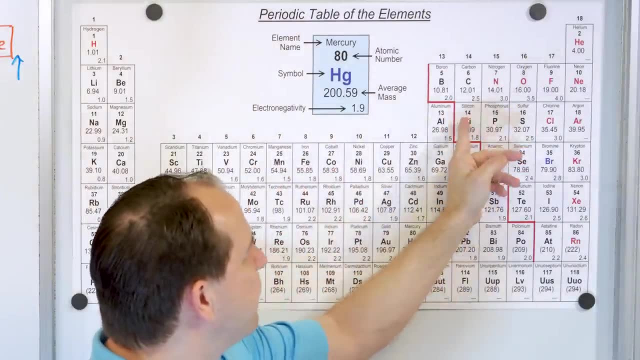 no spaceships, no screens of any kind, any kind of screen without any silicon right. So silicon is really important and silicon is right on the border of the metals and the non-metals, because silicon has properties of being a metal and also properties of being a non-metal. You know what? 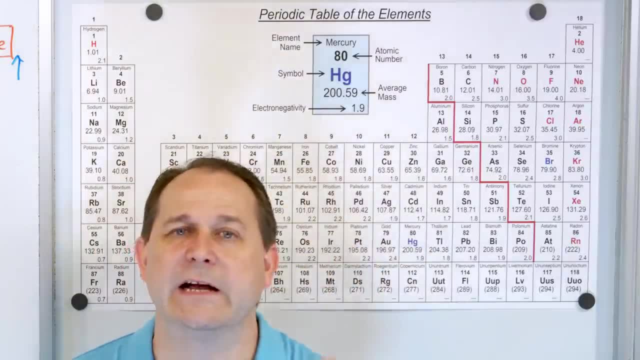 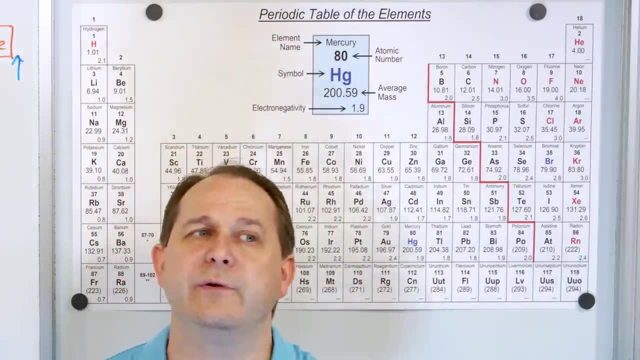 that lets us do That, lets us build things that are not metal, and that lets us build things that are silicon, that can behave as an on-off switch. So when we want silicon to conduct electricity, we can make it do that, but when we want it to not conduct electricity, we can make it do that too, So it can. 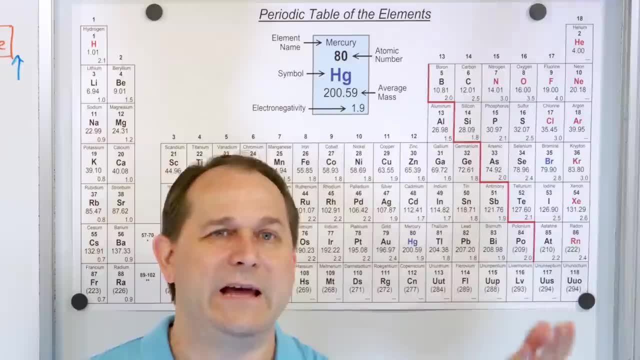 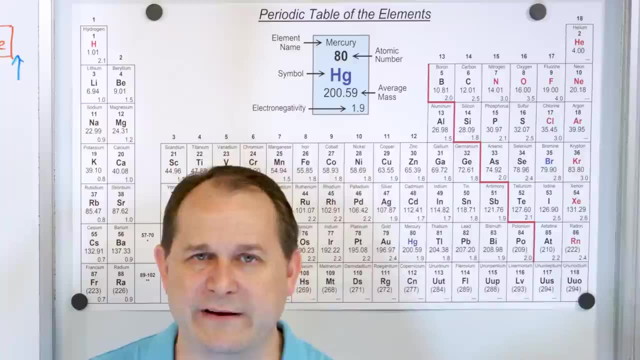 behave as a switch. And guess what? A transistor is basically a switch. That's what a transistor is. It's a tiny, microscopic switch made out of silicon, And when we put a bunch of transistors on a chip then you can have a computer. And so without transistors you can't make computers Without. 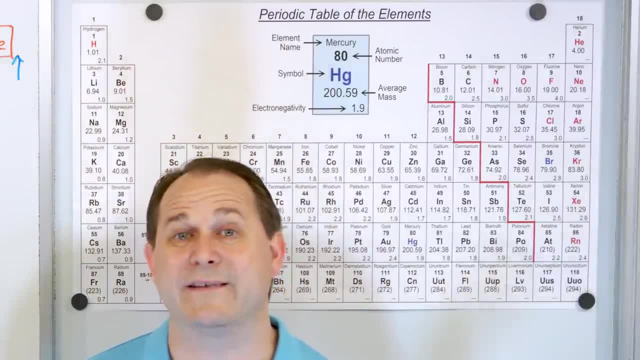 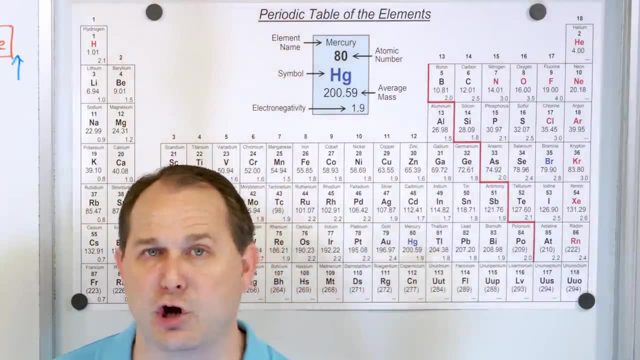 computers. you can't do anything In the modern world, and none of it's possible without silicon. So this is an extremely important element. Right above silicon is, of course, carbon, and carbon is the building block of life on Earth. I mean, who knows if there's life elsewhere that's not based on carbon? but 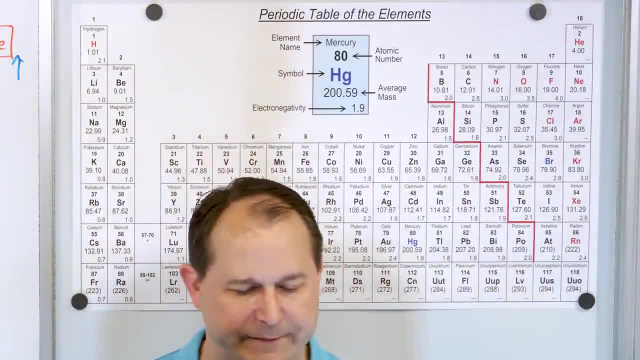 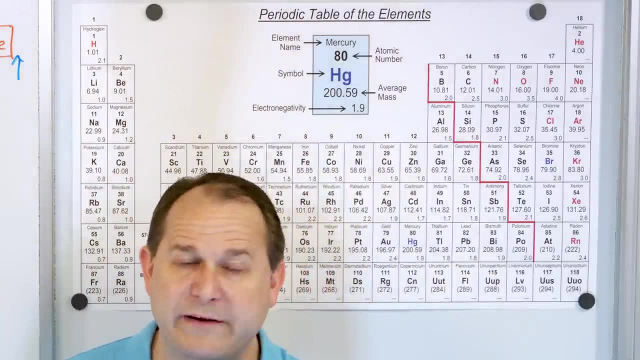 on Earth. anyway, as far as we can tell, it requires carbon to exist. So I want to make sure I get through everything, because I have a lot of stuff to say. We talked about the periods, We talked about the groups, We talked about the properties of the elements and the groups being. 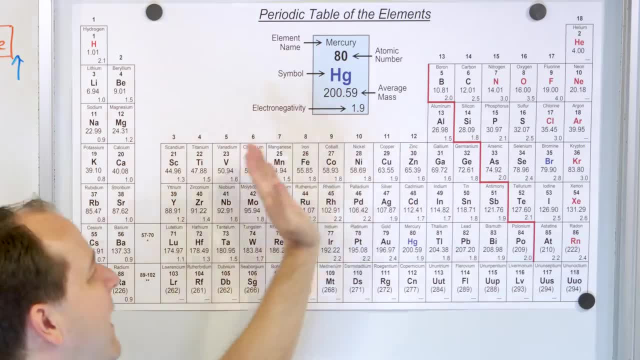 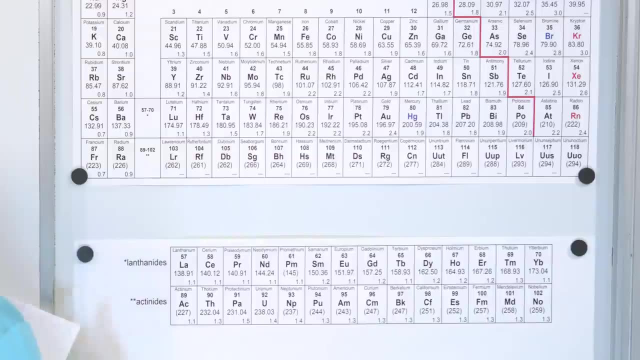 the same Now. on the left-hand side of the table we have the metals. On the right-hand side of the table we have the non-metals, In the middle we have the transition metals And, if you notice, down below the periodic table. 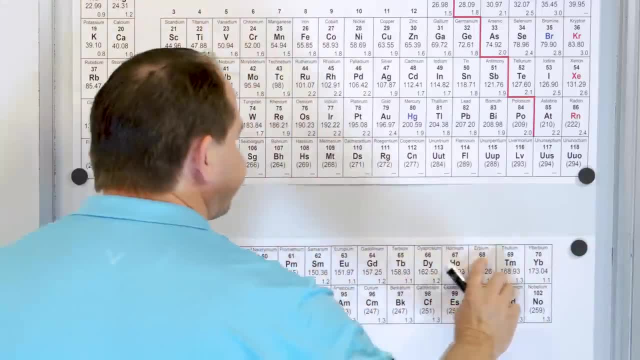 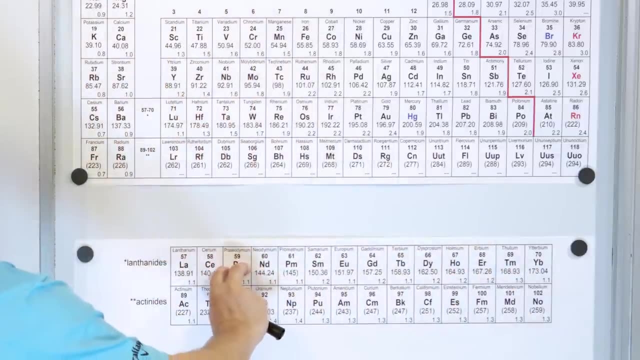 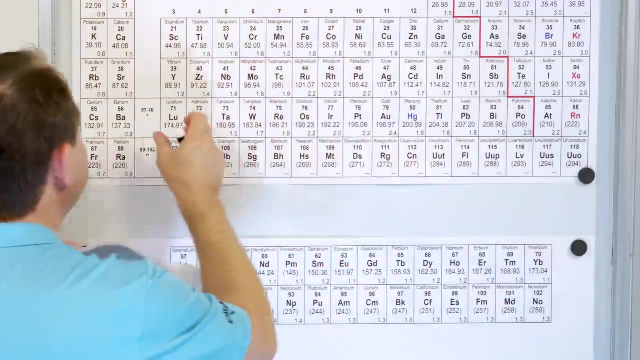 we also have this extra row right here which actually this extra row consists. these are pretty high atomic number atoms here, And we have these actually fit inside of this little region. You see 57 to 70 and these numbers here, This entire row right here actually fits. 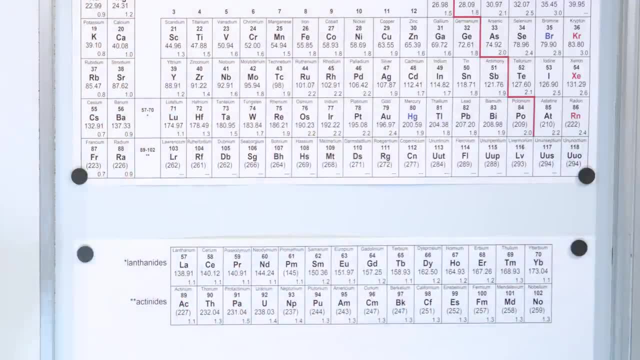 inside and pushes the table to the right. I'm going to show you a picture of that in a second, but all of these elements kind of live inside Here, so just hold tight. I'm going to show you what that looks like. What I want to do now is I: 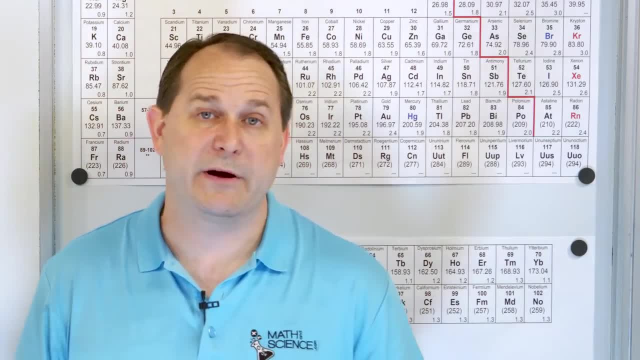 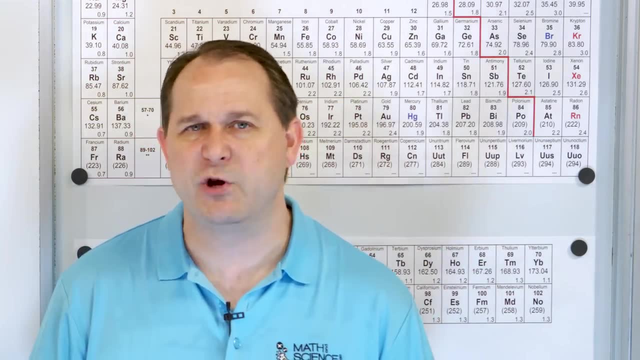 want to tell you one of the absolute most important things that you need to know about the periodic table. I don't really have to mention it now, but we're going to use it so much I want to introduce it to you If you don't remember it at the end of this. fine, no big deal. What you really have with. 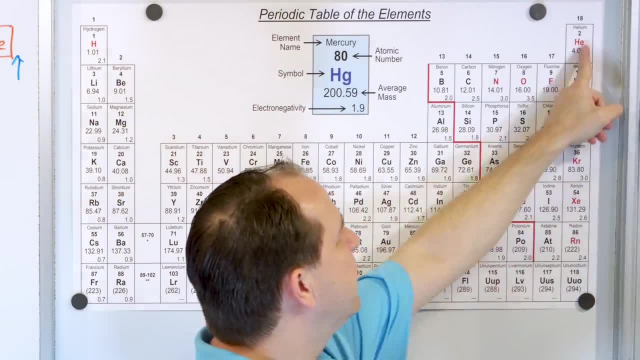 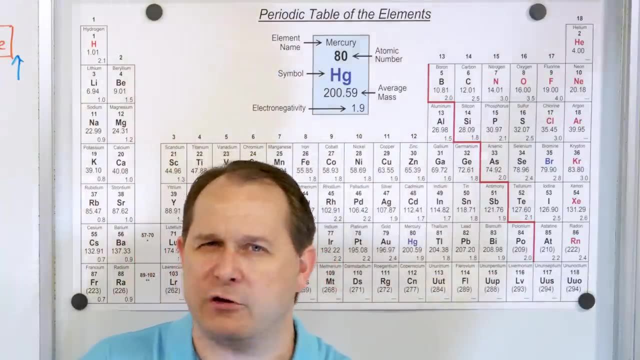 this periodic table is. you have these non-reactive gases, which we call noble gases, And they're non-reactive because they don't. their electrons are stable and they don't like to be shared or given away, And so they don't react with anything. That's what we have there. 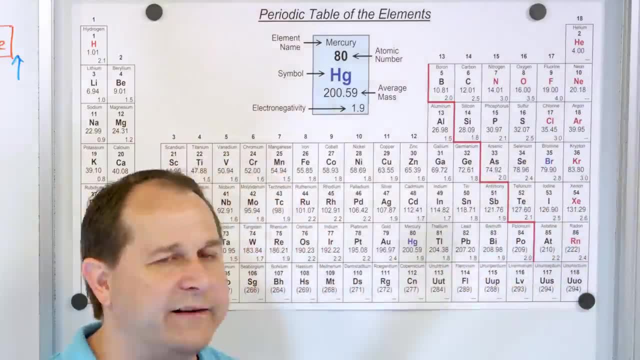 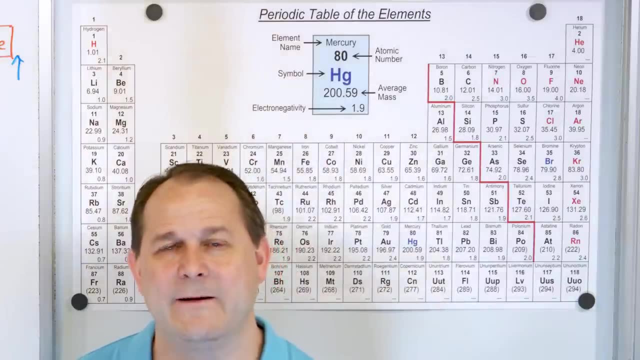 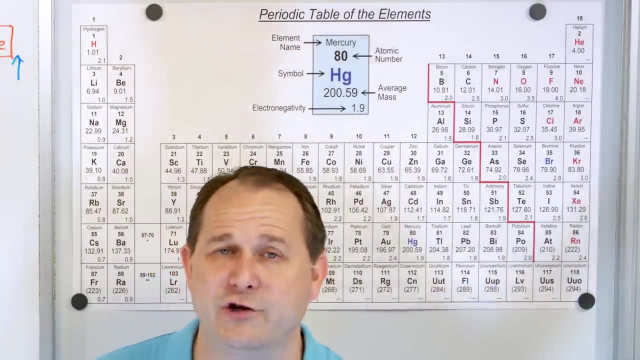 It turns out that the other elements nearby, the noble gases, are always trying to get to an electron configuration that is as similar to a noble gas as it can get. I'm going to say that again: All the elements on this periodic table are always trying to get their electrons to look like. 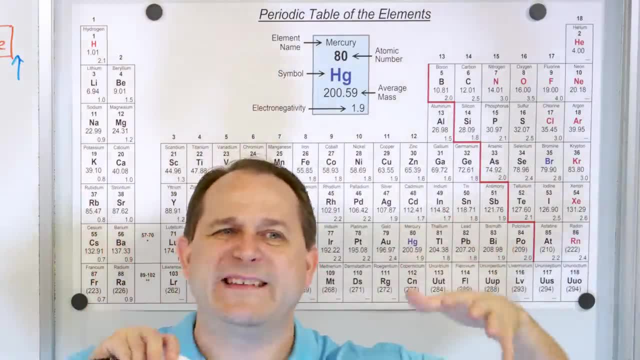 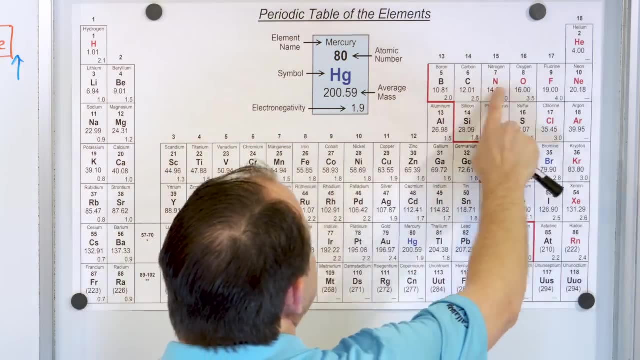 noble gas electrons. What I mean by look like it is we want them to have the same number of electrons in the same orbital shells that we're going to talk about later. So what we have here is notice that neon, for instance, Neon. 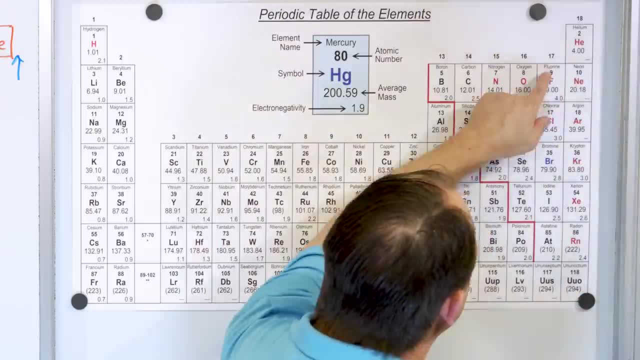 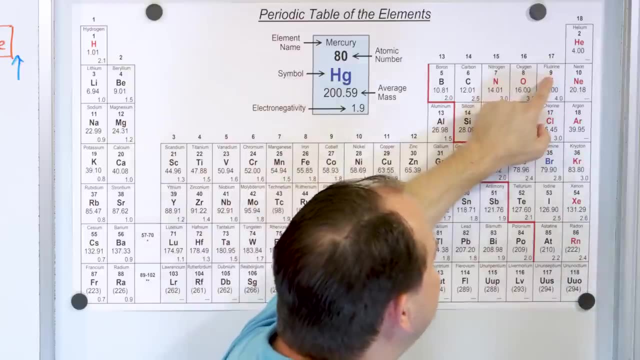 as always, has 10 protons, and so it must have 10 electrons. So fluorine is right next door. it has nine protons, and so it must have nine electrons. But fluorine is always trying to be as close as possible to the nearest noble gas it can be, which is right here, next door, at neon. 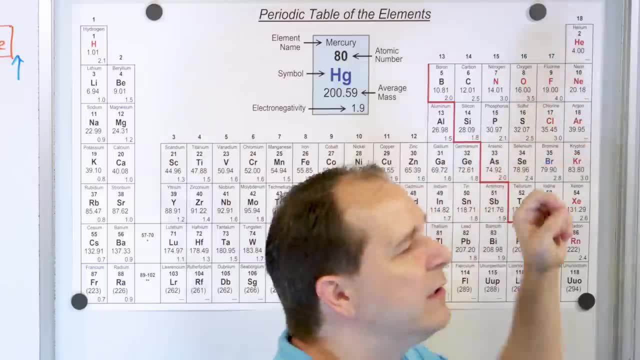 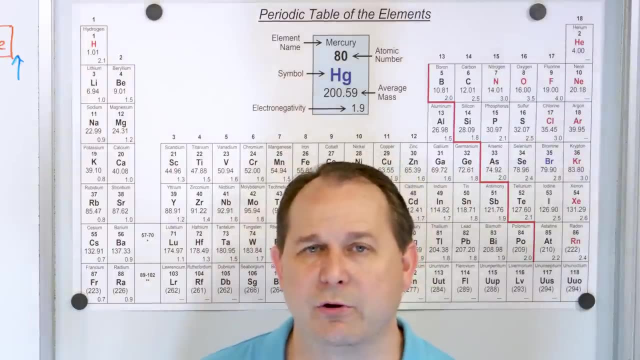 So if it has nine electrons, all it needs is one additional electron to have the same number and orientation of electrons as the noble gas. Everybody's trying to be like a noble gas, And so what does fluorine want to do? It wants to gain a single electron. It wants 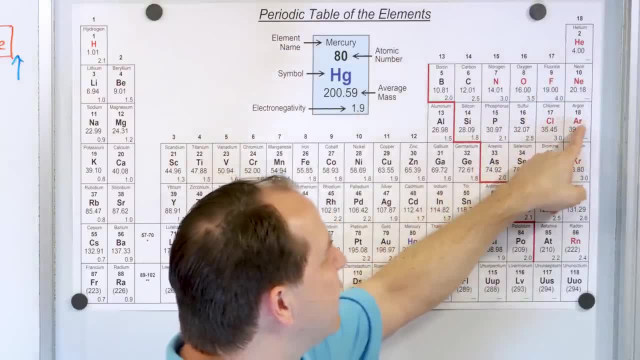 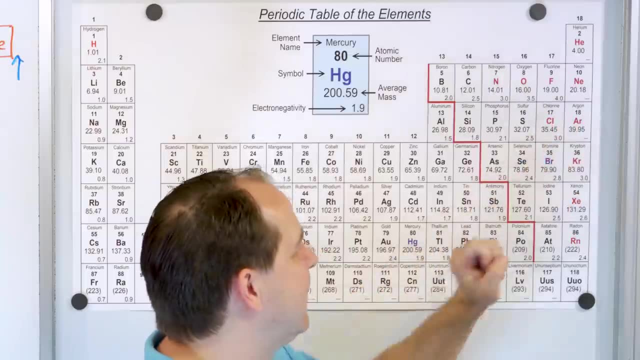 to gain an electron. Chlorine is always trying to be as close as possible as it can to argon in terms of its electron count and the structure of its electrons. So it's always trying to gain an electron, And the same thing with these other ones here. But see, oxygen is. 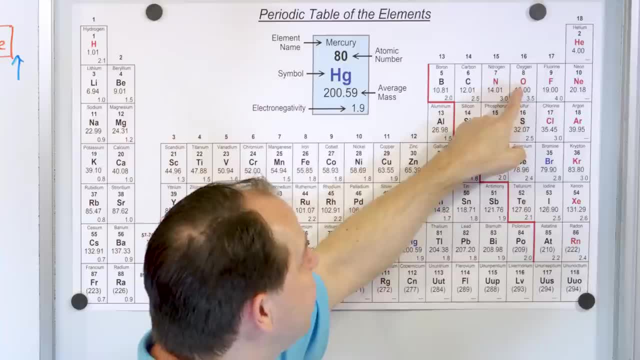 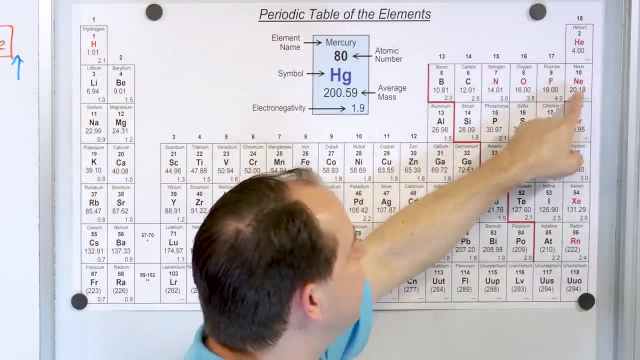 two spots away from neon, And so the closest noble gas is neon. Of course you could go this direction and say that there's another gas called helium, but that's too far away. It wants to be nearest to the closest one, So it wants to gain two electrons because 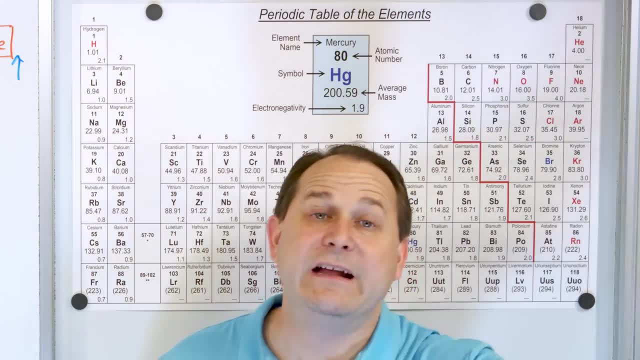 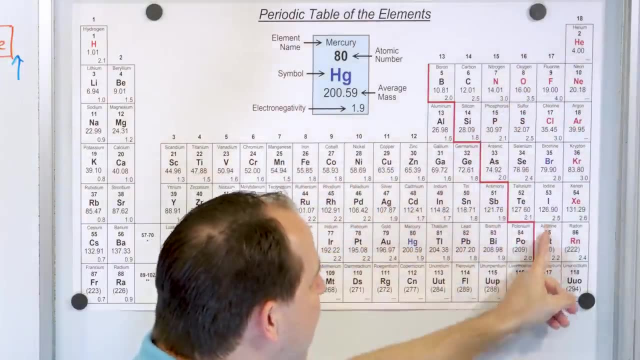 it currently has eight and it wants to have ten, And if it can gain two electrons it'll have the same outer electron configuration as its nearest noble gas. So the column that it's in is telling you how many electrons these things want to gain when they participate. 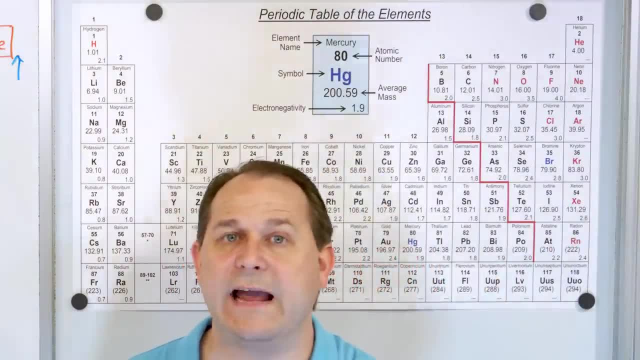 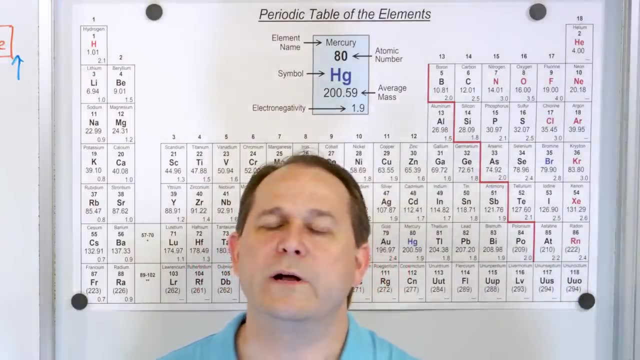 in chemistry. That's what drives the chemistry. They want to gain electrons because they want to be closest to as they can be to a noble gas, and that's what drives the chemistry, because when elements gain and lose electrons, that's what makes chemistry. 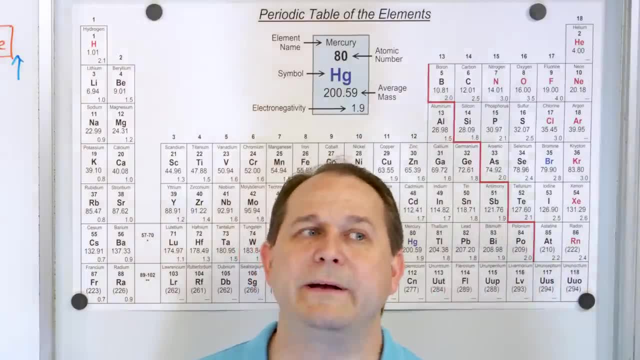 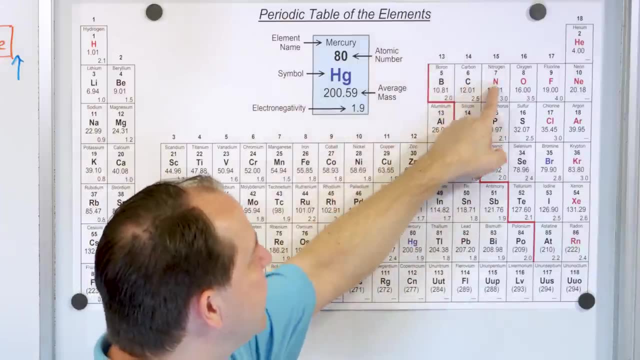 happen, And I'm telling you now how you can figure out on your own how many electrons it wants to gain. In this case, oxygen wants to gain two, fluorine wants to gain one, and so on. Carbon can gain up to four electrons, and that has to do with the importance of carbon, for instance. 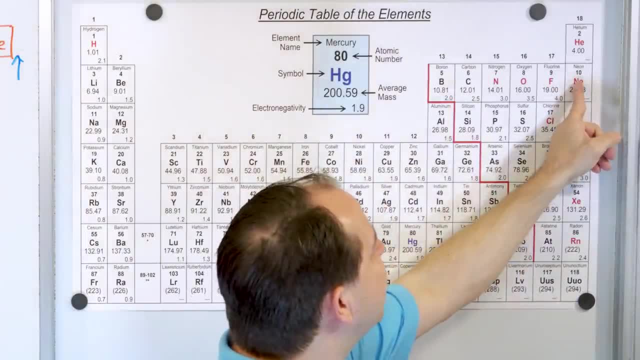 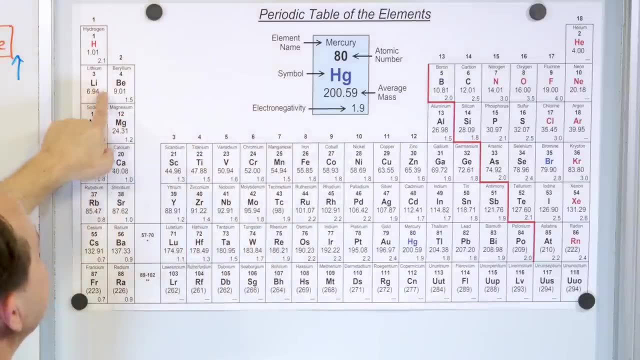 Okay, Now over here, notice to the left of neon. if we unfold the table and just write them in a straight line, one spot to the left is. well, let me go look at sodium. I guess Atomic number 11.. 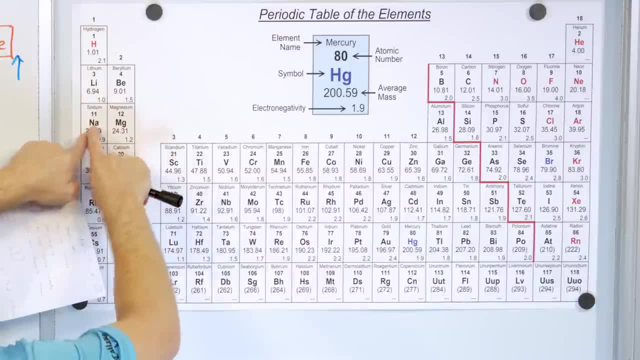 So what noble gas does this thing want to be next to? Well, it can go all the way down here and you could say it might attempt to be like argon, But actually the nearest noble gas to this one is the noble gas just on the previous row, because this has 10 protons and 10 electrons. 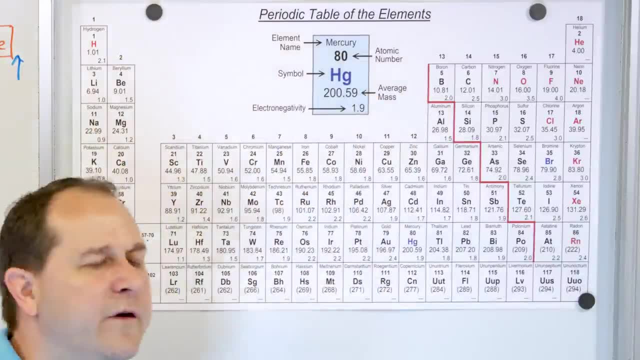 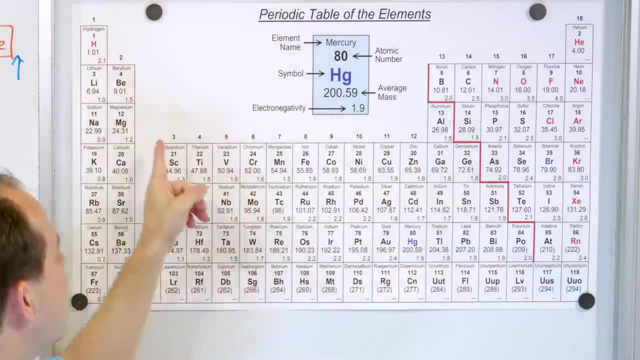 but sodium has 11 protons and 11 electrons. So how could sodium, if, given the choice, be as close as possible to the nearest noble gas, The much easier way? sodium would have a hard time gaining all these electrons. to be like argon, That would be very difficult, okay. 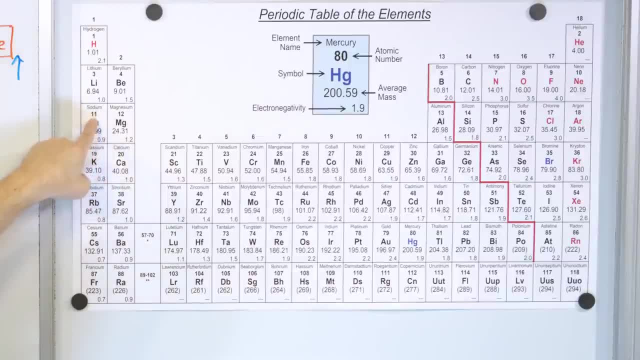 But what it can do is it can just give away an electron. What if it just gives one of its electrons away? So now it only has 10, and then it would look just like neon. You have the same thing with potassium. Potassium wants to be like its nearest noble gas. It's going to give away. 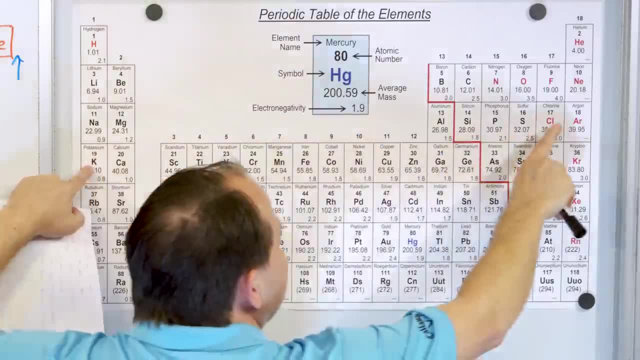 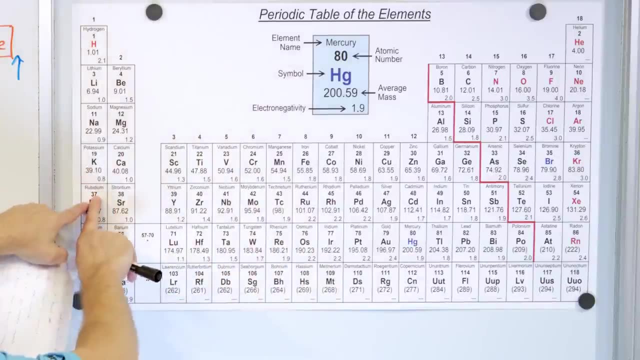 an electron, thereby having 18 electrons. and look at this Argon has 18 electrons. So if it gives an electron up, it becomes like the nearest noble gas. If this one gives up an electron, it becomes like its nearest noble gas, and so on, And we can do the same thing in the column next. 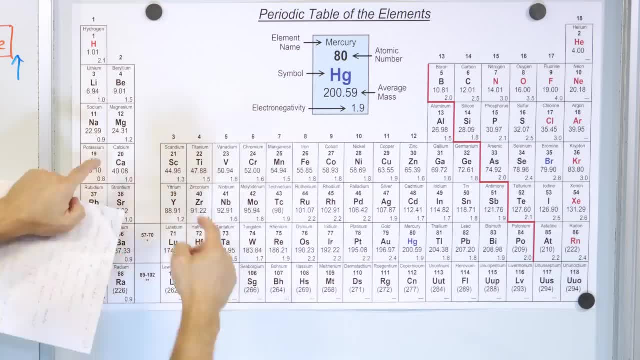 door. What would magnesium want to do? right, Of course it could try to gain electrons and go here, but that's too far away. It would rather just give up two electrons and become like neon. So everything in this column is going to give up two electrons and become a positive ion. 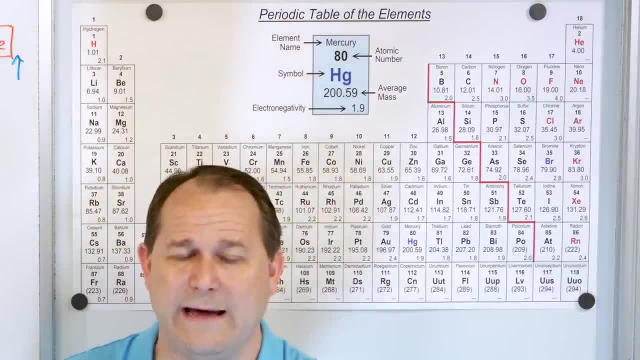 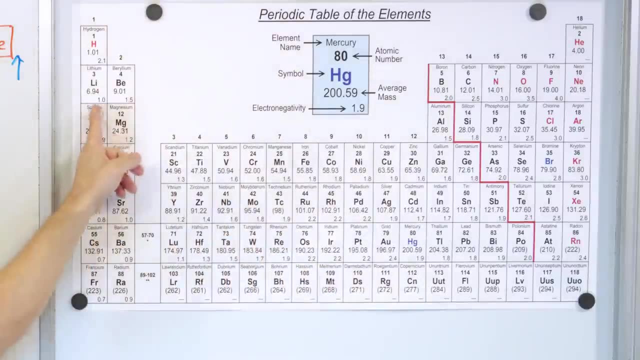 because, remember, if you're neutral and you give electrons, you're going to give up two electrons away. then your nucleus has an extra positive charge. You're going to have a positive two charge. So when you give away electrons, you're going to have a positive charge remaining left. 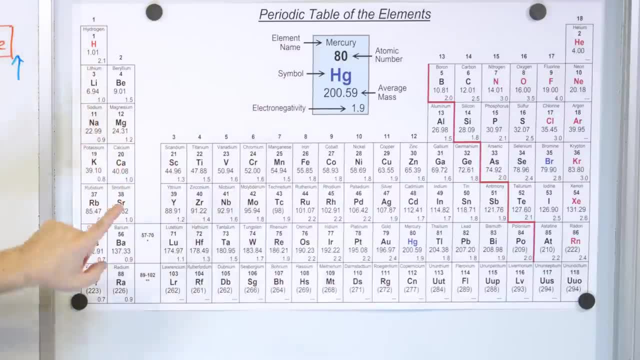 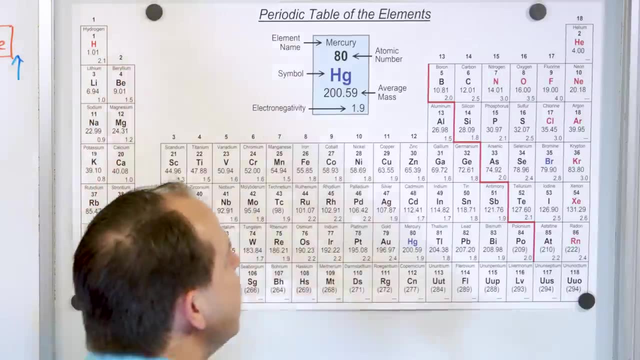 over on the atom. We call that an ion. We're going to talk about that in a little bit. But this column wants to give away two electrons. This column wants to give away one electron. This column wants to gain an electron becoming a negative one ion. This column wants to gain. 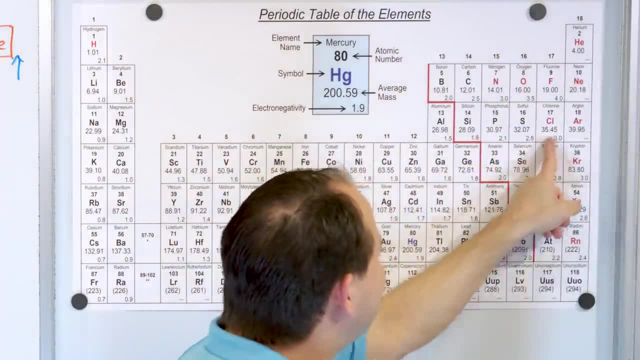 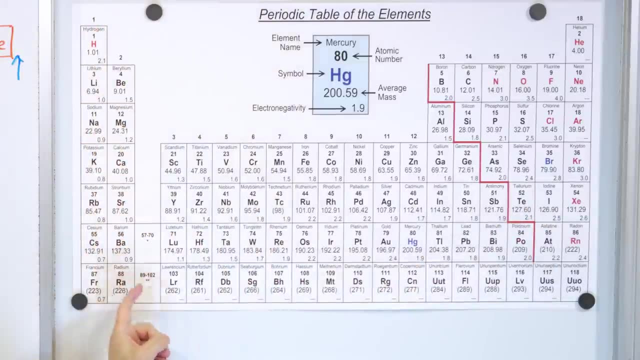 two ions. So, once again, this column wants to gain one electron. This column wants to gain two electrons. This column wants to lose one electron. This column wants to lose two electrons. And this column doesn't want to do anything. It doesn't want to gain or lose anything. Now I want to. 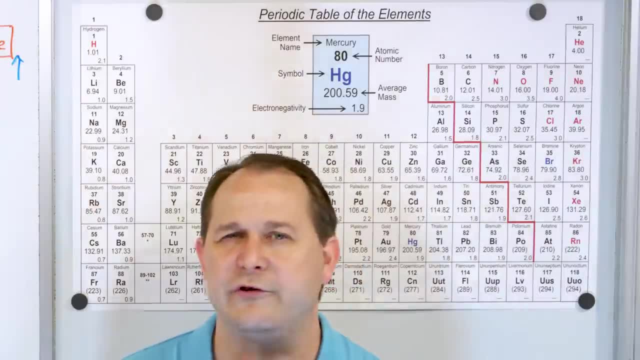 take a second and tell you about a pet peeve of mine: that when you read different books or you just talk to people, I don't like using the words: this element likes to do this, this element likes to do that. I know I've said that a bunch here, but I really don't like using it because it's. 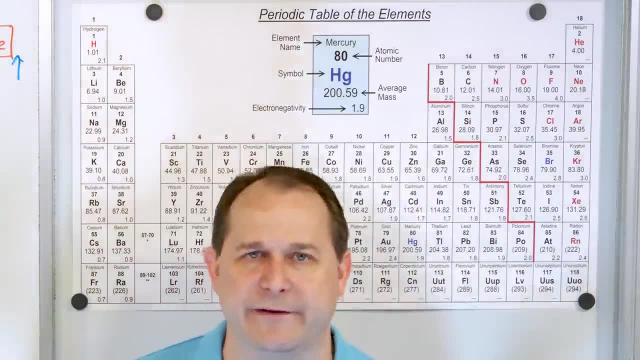 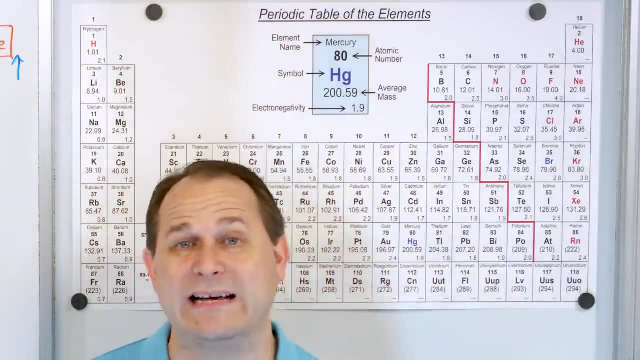 because it leads you to believe that these elements have a personality and they just have preferences. It's not that they have preferences. It's not that they want to be like a noble gas. It all comes back to what I told you in lesson number one: Everything in chemistry comes down. 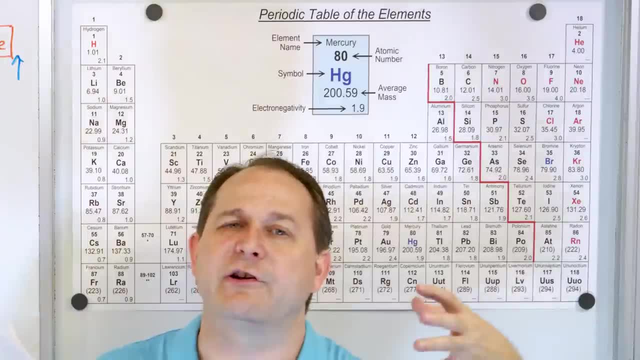 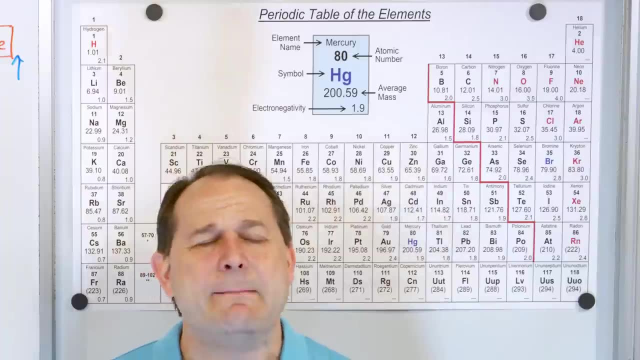 to the electric force. The electric, the force of electric charges, is millions and millions of times stronger than gravity, And I showed that to you in a previous lesson. right. Millions and millions of times stronger than gravity. We think gravity is really strong, but actually the electric. 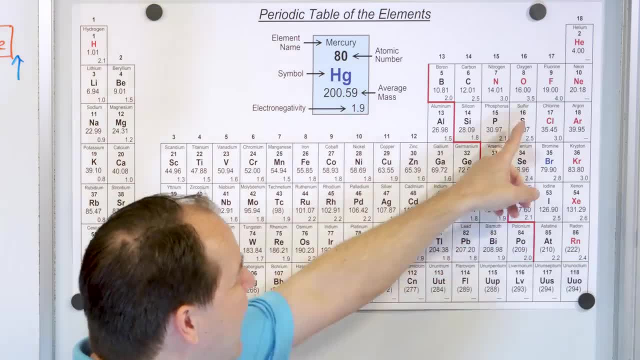 forces are way stronger than gravity And we think gravity is really strong, but actually the electric forces are way stronger. So why does this thing want to gain an electron? quote unquote- want to gain an electron? It's not because he wants to, because he has a preference, It's because the 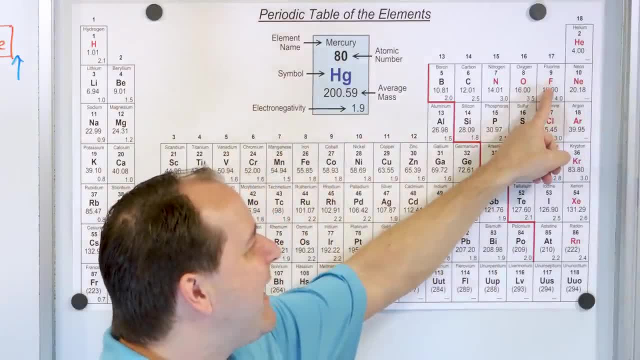 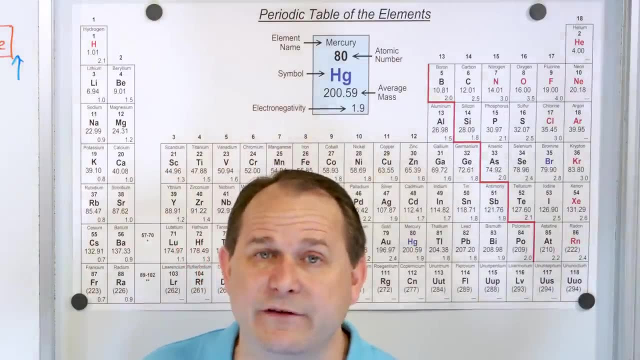 electric forces are so strong on this thing that they allow fluorine to suck an electron in from almost anything it reacts with right. Why is it allowed to do that? We're going to have to talk about that later, when we get to showing you what the structure of the electrons look like in the 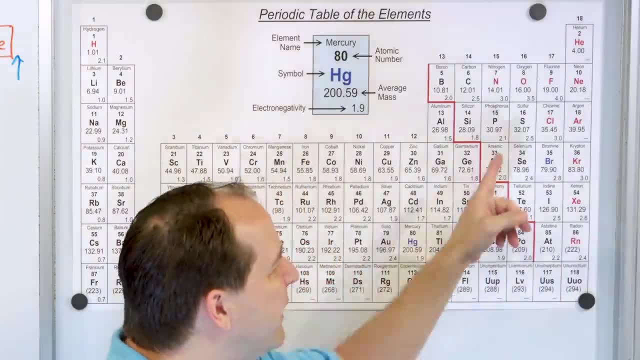 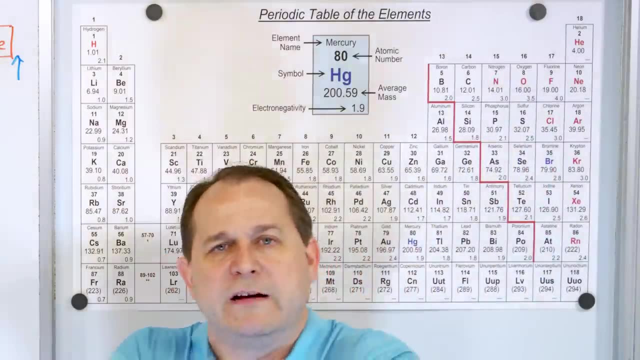 electric forces that happen. I can't do it all in one lesson but the reason fluorine and chlorine and bromine and ether are so strong is because they allow fluorine to suck an electron in from these things want to gain an electron so readily is because the electric forces are so strong. they 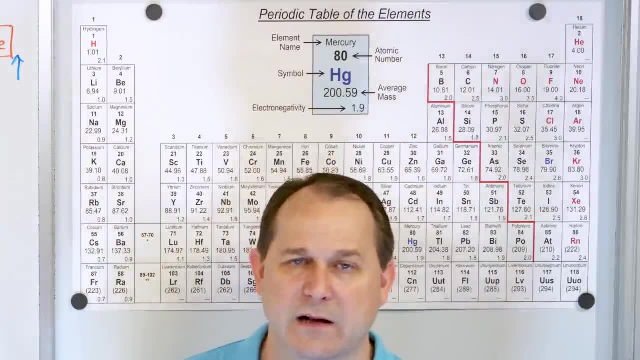 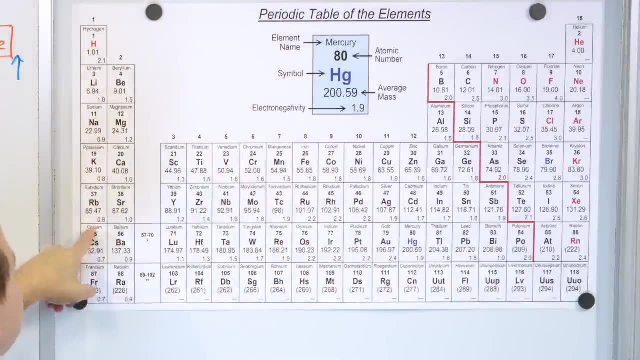 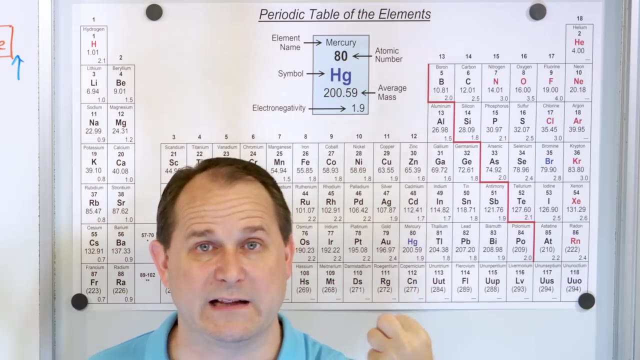 can suck in and attract and rip out a negative electron from something else. And why does sodium and lithium and these other things, why do these elements here want to lose an electron? Well, it's because the outermost electron on those atoms is not held very, very strongly from the electric 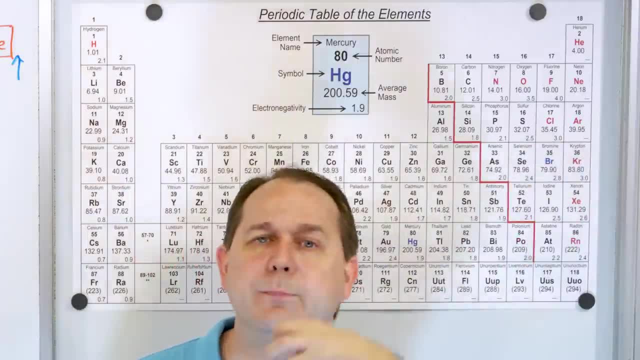 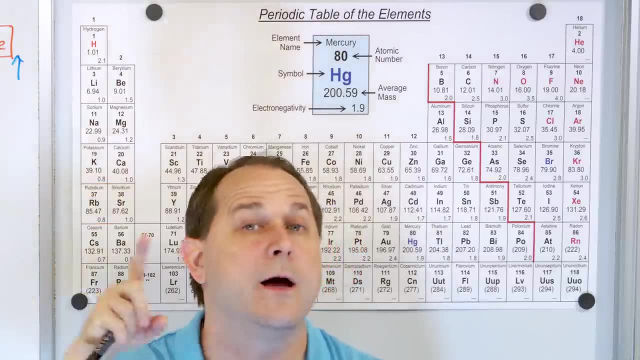 force. So the hogs like fluorine and chlorine are able to rip it away. So you see, on the left side of the table you have outermost electrons that are not really tightly held on by the electric force. We're going to talk about why later. but these atoms have outer electrons that are not 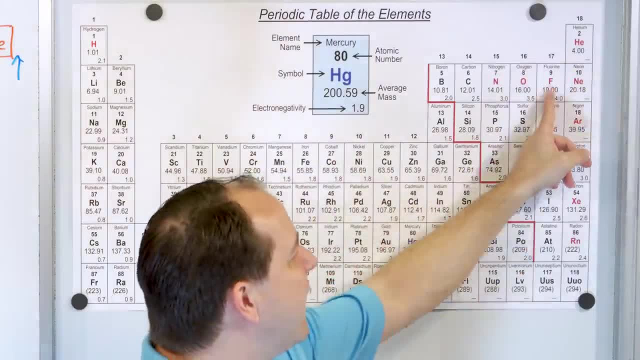 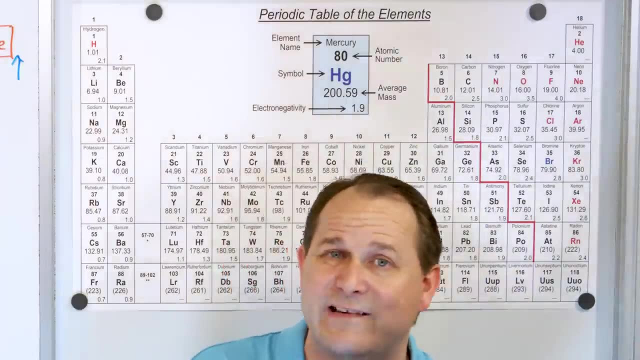 held very tightly by the electric force. And these elements over here, over here, they want to to attract, and they do attract electrons so readily, because their situation is opposite and they are able to attract electrons with overwhelming force. So what happens? is it just? 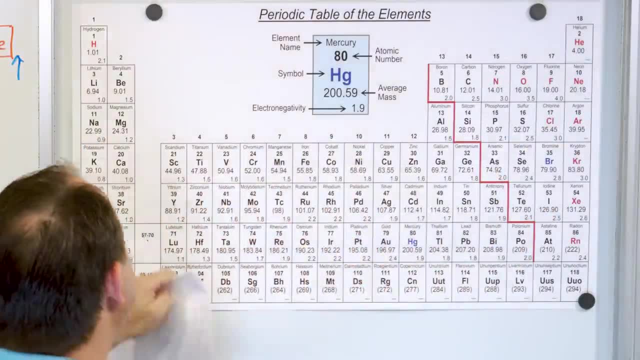 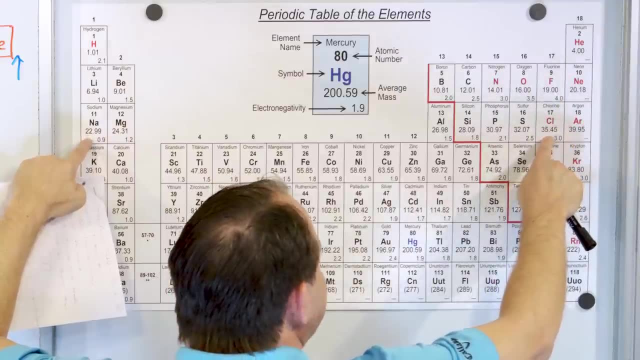 sucks the electron from this side and it goes into this side And that's why it's so strong. That's why sodium- chlorine react together, because chlorine really wants to grab an electron and has a very strong electric force to do so, But sodium has an outer electron that's not very tightly. 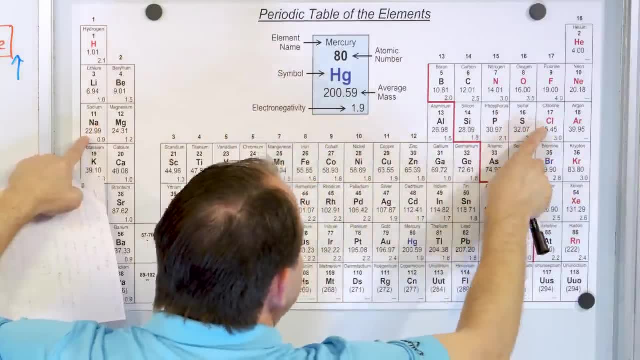 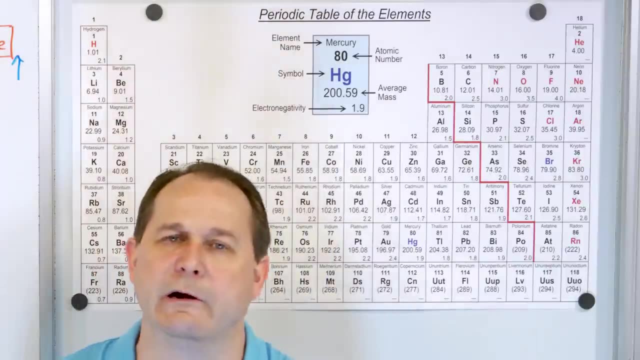 bound. So what happens is chlorine just sucks sodium electron over there and it satisfies both parties, And then they bond together and they become table salt. What I'm telling you here about predicting if you're going to gain an electron or lose an electron is one of the most 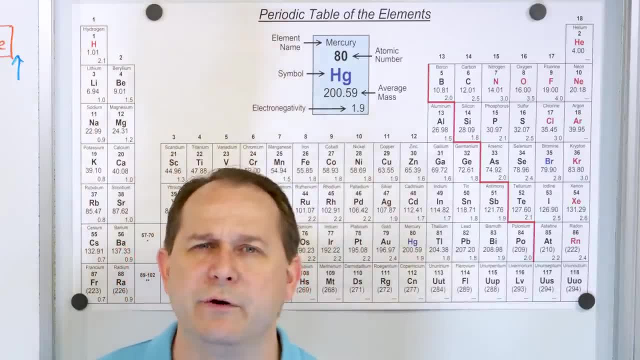 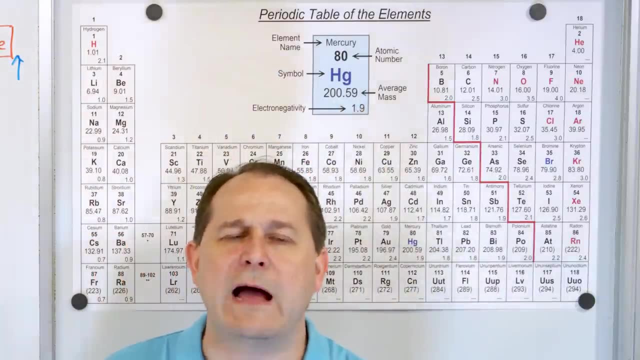 important things the periodic table is for. In fact, I will go as far as to say it's probably the most used thing on the table, except for the atomic mass. We use that a lot too. Mostly when you're looking at the table you're trying to figure out how many electrons something's trying. 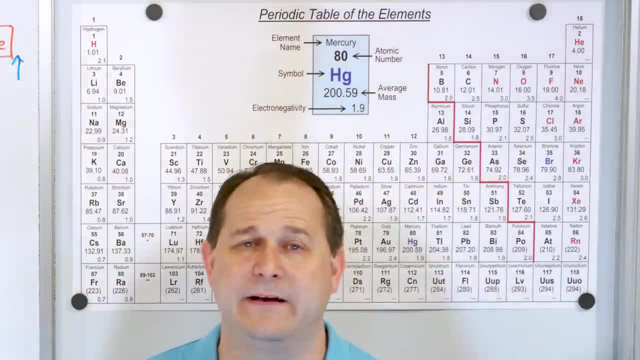 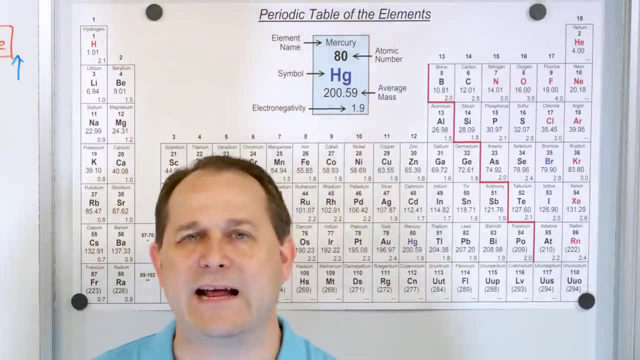 to gain or lose, because that's going to help you predict what's going to happen in the chemistry And by knowing the column it's in which we call groups- by the way, what group it's in, you can predict what's going to happen because you'll know how many electrons it's going to. 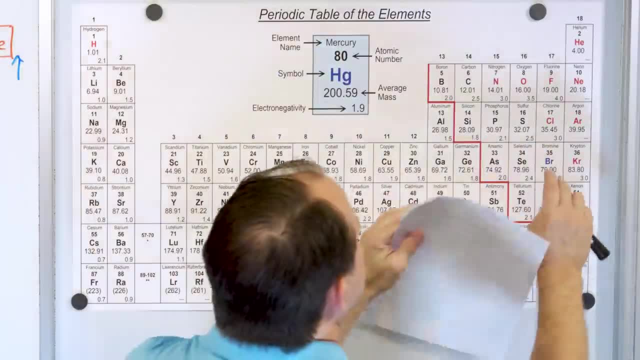 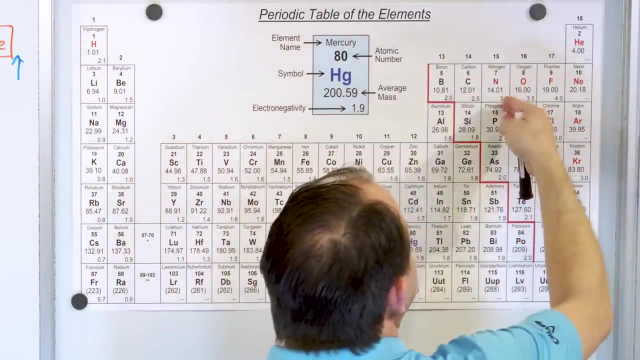 gain or lose. So in summary, on the right-hand side of the table, these elements in general are trying to gain electrons- They are called nonmetals, right- And they gain electrons and become more negative and they become and look like the outer electron configurations of the. 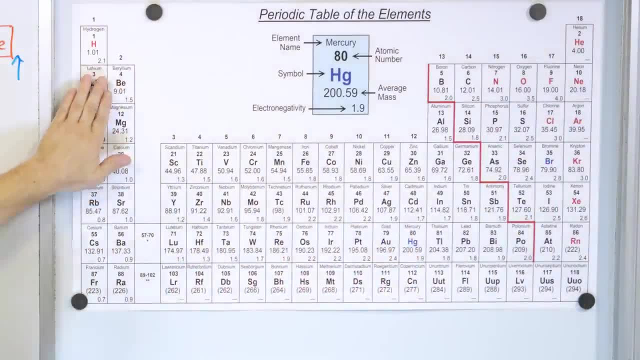 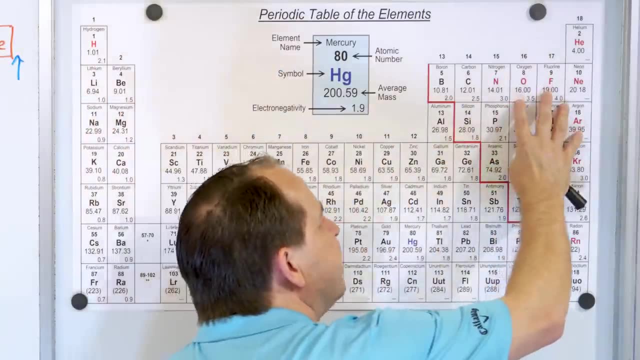 noble gas, These elements over here. they try to lose electrons and they try to lose as much electrons to also be like its nearest noble gas. So because half of the table is trying to gain electrons and the other half of the table is trying to lose electrons, they can party all day. 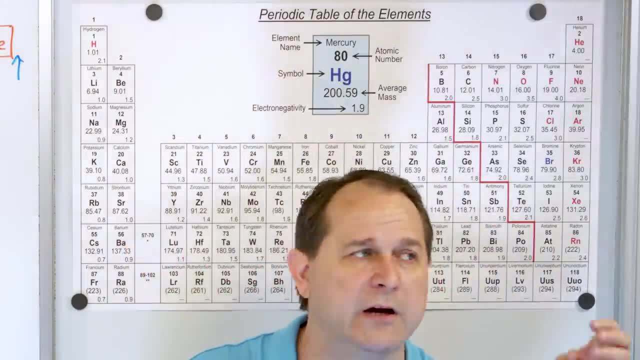 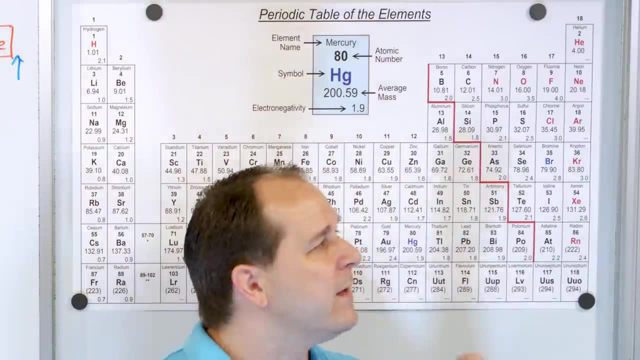 long, because one element is readily able to give up an electron, The other element is able to give up an electron and the other element is readily able to take an electron. and then they're going to party because they are a match made in heaven, okay, So we're going to talk a lot more about 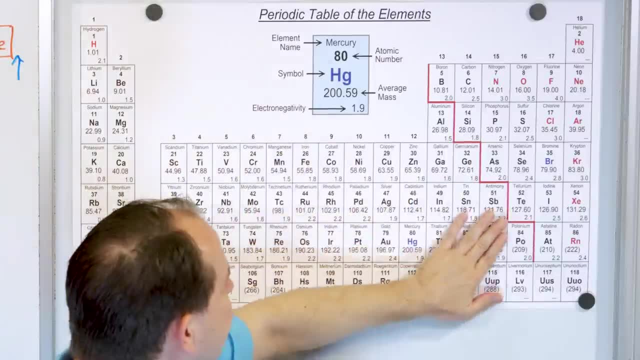 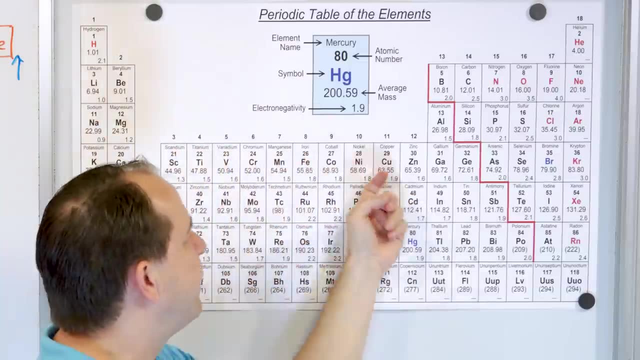 that, but that is the basic idea. The elements in the center: they're also metals. They generally do like to give up electrons as well, just like these, but they're not quite as reactive and the rules associated with these middle elements are not as cookie cutter. okay, The elements on the 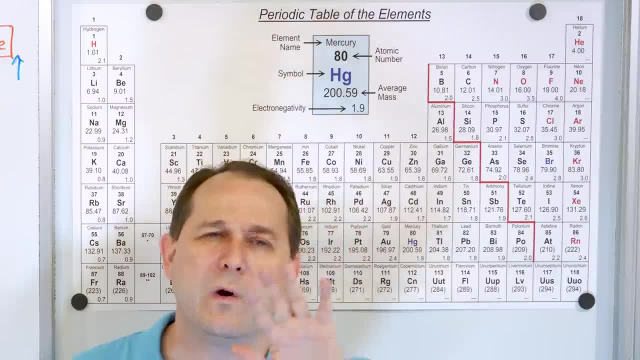 edges of the table, we can predict with great certainty what's going to happen. The ones in the middle of the table, they can do whatever they want to do. They can do whatever they want to do. They can do different things depending on what's happening. So it's not quite as like I said. 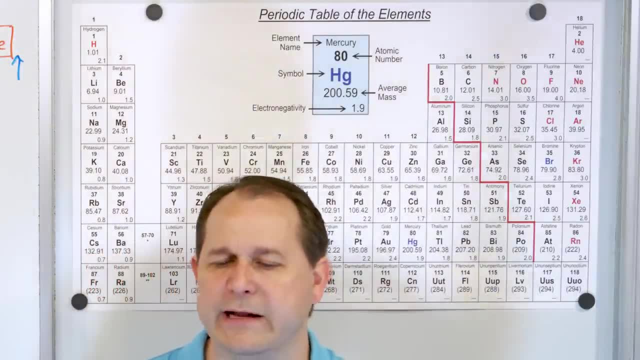 cookie cutter. So let me go down and make sure I have everything. So periodic tables are arranged by atomic number. Properties emerge. We have noble gases, are non-reactive. on the right We have right next to it. on either side we have very reactive elements. We have atomic number. 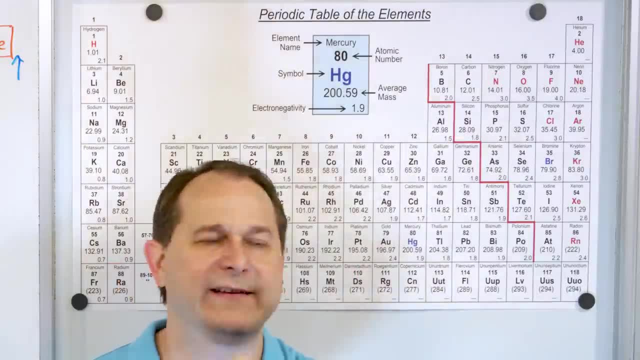 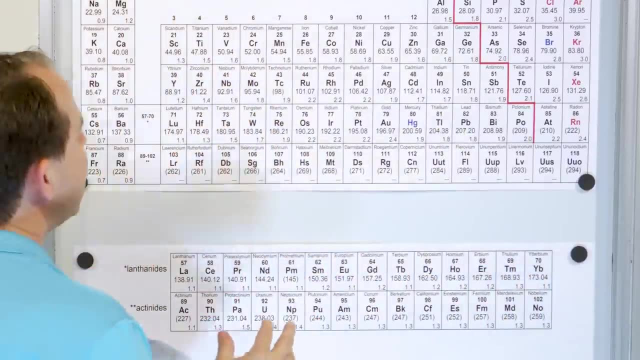 atomic mass periods, groups losing and gaining electrons. And then the next thing I wanted to show you was the bottom of this table has these two rows which are also always down below. I never really understood, when I first learned chemistry, why it was down below like this. 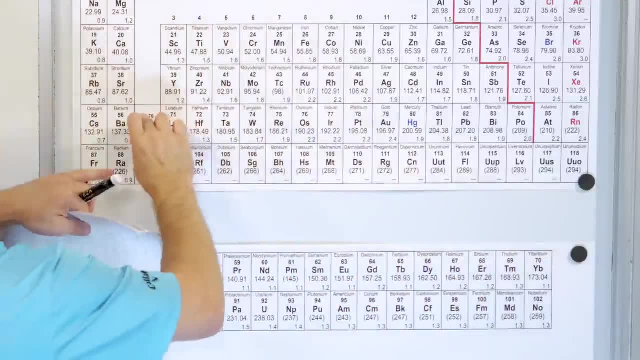 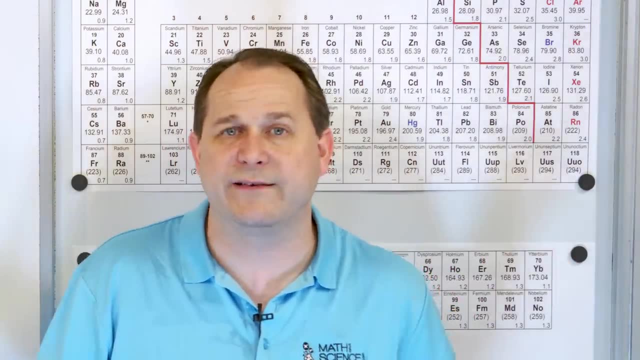 Let me show you. These elements really fit inside of these single boxes and they push the table out. but because they push the table wider, you can't print it so easily on a sheet of paper. So let me show you what it would look like if you did that. This is what the periodic table. 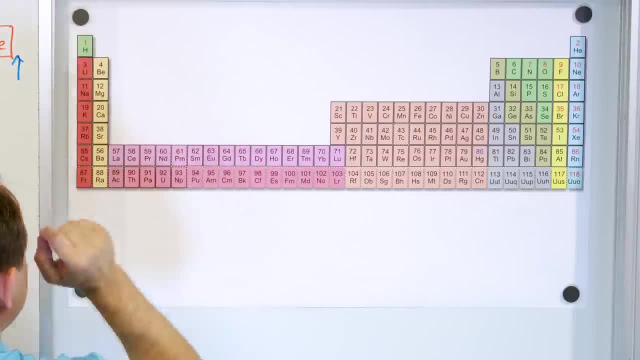 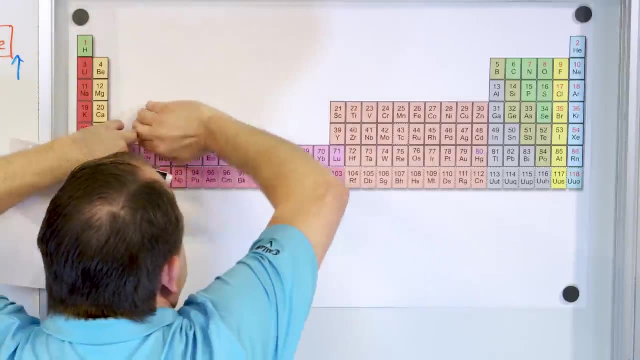 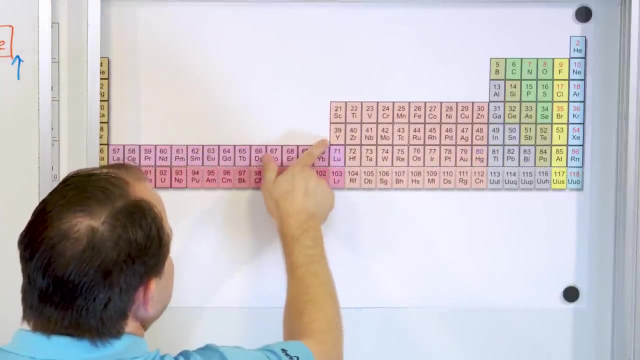 actually looks like with those two rows inserted or the two periods, these two periods inserted into place, Notice what happened is we stuck them in there and then this: basically the whole table got pushed to the right And it's a little more difficult to read it because it's so wide right now. but this is S, C and Y Yttrium. 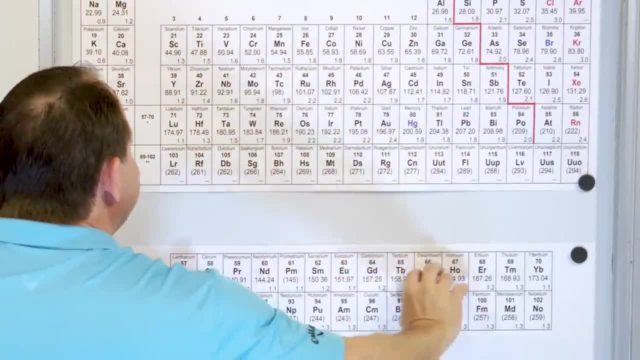 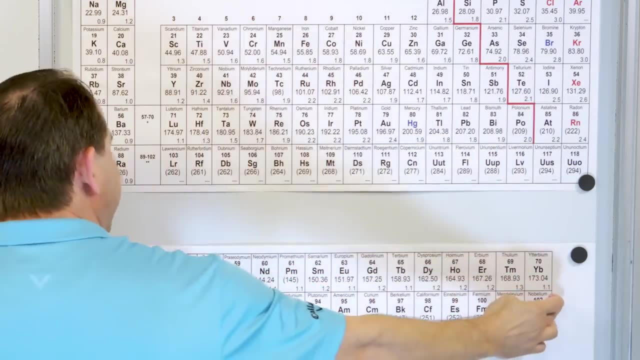 So here is scandium and Yttrium. So what happens is these two rows go in here and they push the and they basically cut it right here and it pushes the table to the right And every one of these elements exist in here And you can see that. 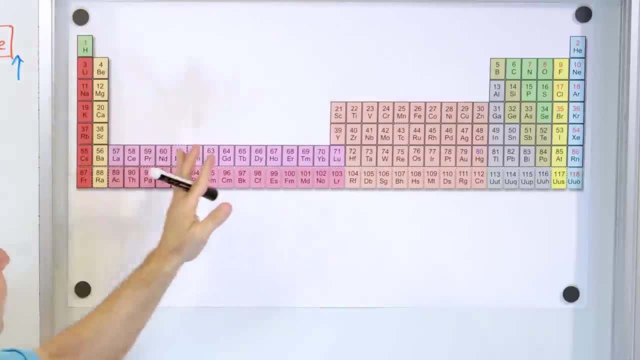 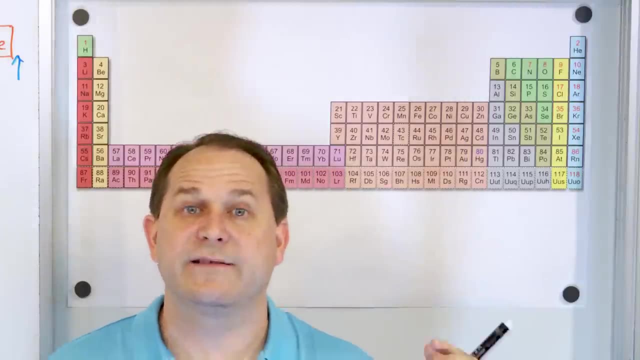 that is what happens here, So that goes in here. So when you look at the table like this, you know at first you kind of get used to the periodic table And then when you see it like this a lot of times, you're like: why is it do that? Why is? 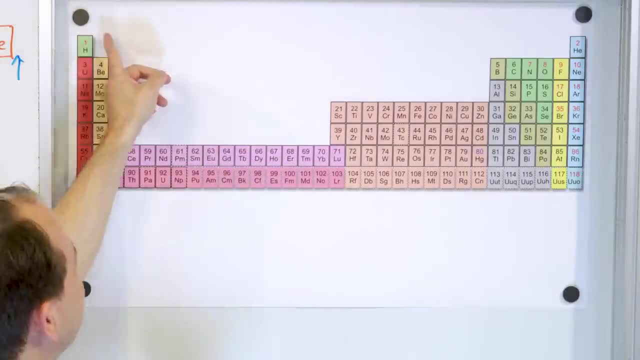 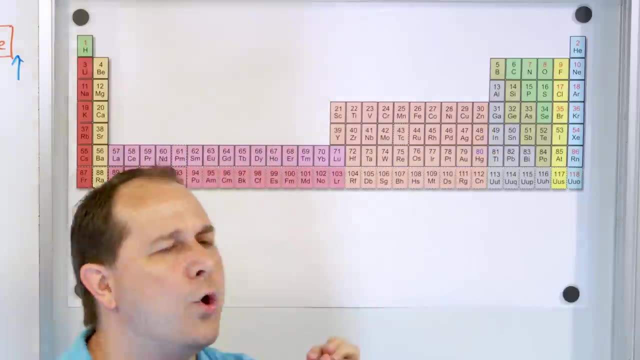 it that way? Why does it have just like these, these top two elements by themselves? And then we have some stuff here and there's a big gap over here, And then there's even a bigger gap right here. Why are the gaps everywhere? All I can say is: everything will be revealed in time, but it 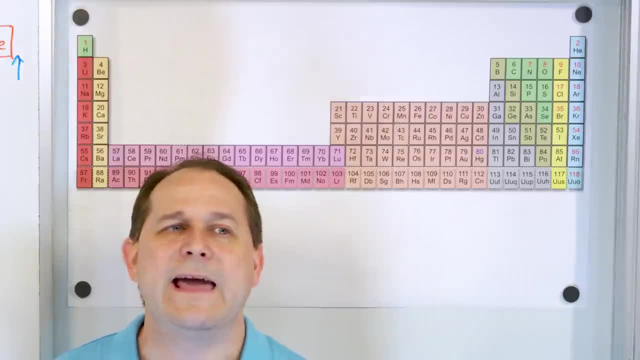 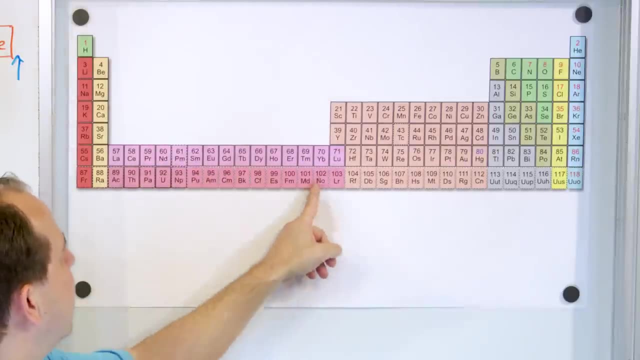 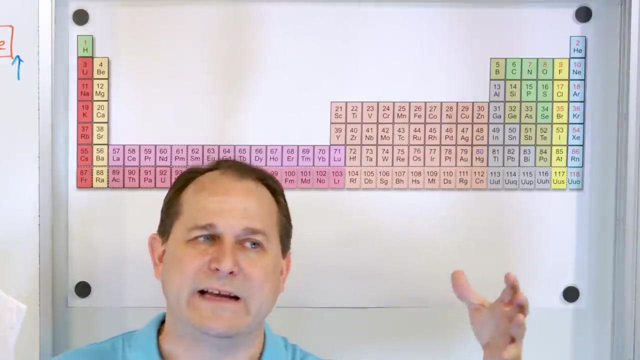 has to do with the electrons. Everything has to do with electrons and chemistry. It basically boils down to how the electrons fill up in the, the shells surrounding the atom, And that dictates all the spacing here. I'm not going to say any more than that because we have to talk in more detail. but that is the reason. It's because when 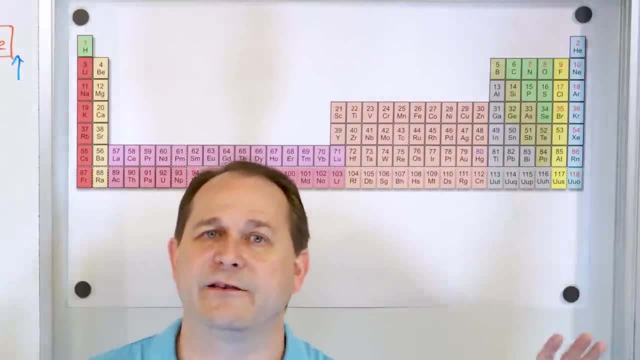 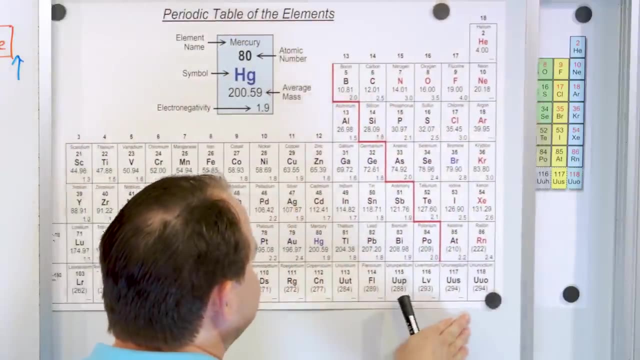 the electrons are filled up. they fill up in a certain way, and that dictates the structure of the table, which we will get to in a lot more details later. A couple more things I want to mention before we finish this lesson out and do our problem, And that is that I kind of glossed. 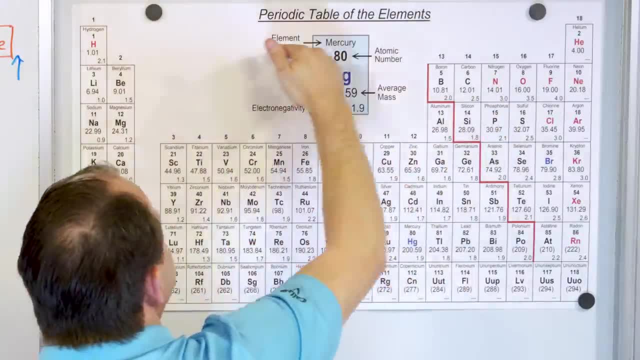 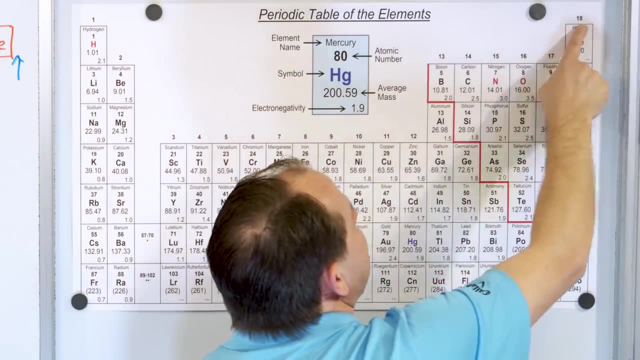 over this in the beginning. but I basically told you we have periods, period one, period two, period three, and then I said we have groups. This is group one, group two, three, four, five, all the way to group number 18.. Now that is the modern labeling: group one through group 18.. So that is the modern. 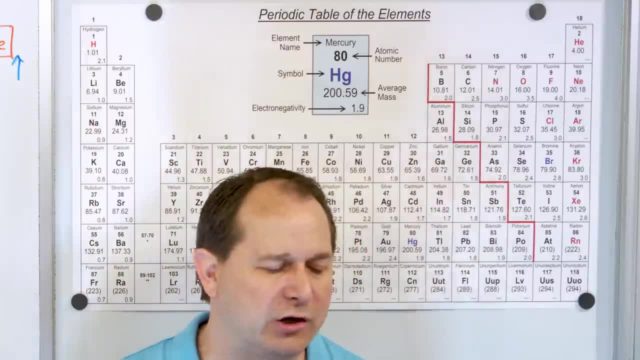 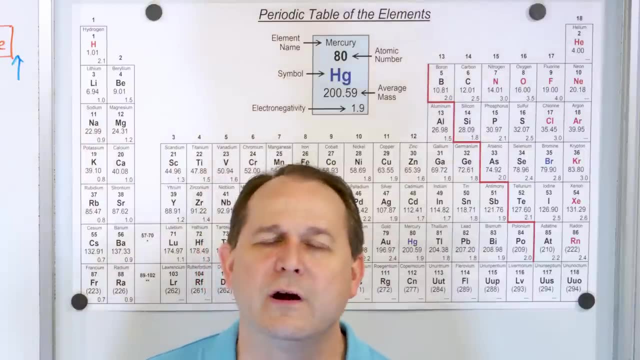 labeling, which is dictated by an organization called IUPAC. You're probably going to see that or hear about that in your class. IUPAC stands for International Union of Pure and Applied Chemistry, So it's a governing body who determines how things are named, basically, and how things are labeled. 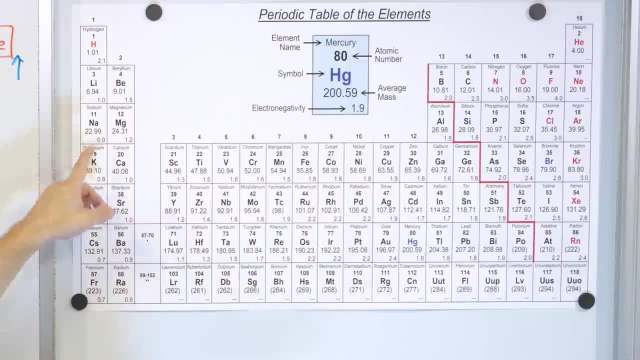 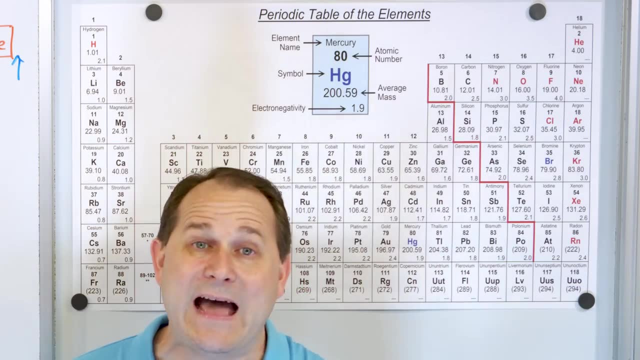 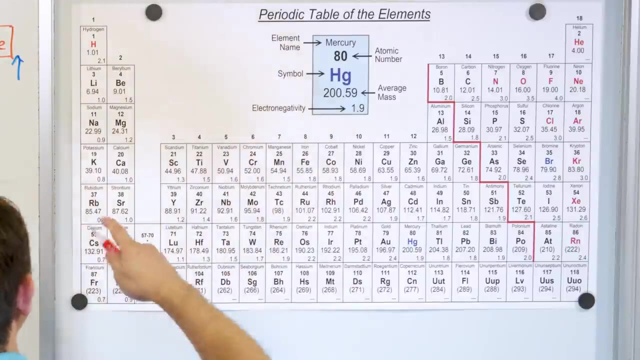 And so it leads to very little. it's very clear to say this is group one and this is group 12, and this is group 18, because everything is very clean. But in the past the periodic table has had different labels for the groups on top. So in the past I will put this in red. Some books: 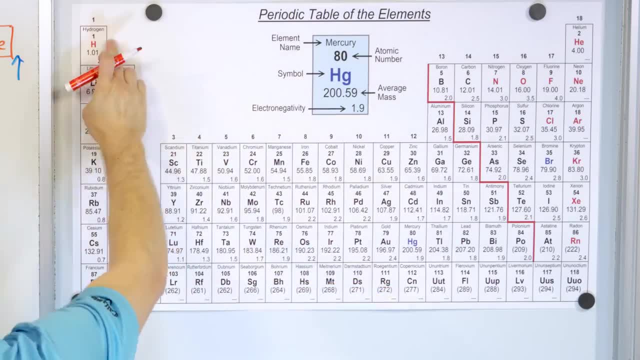 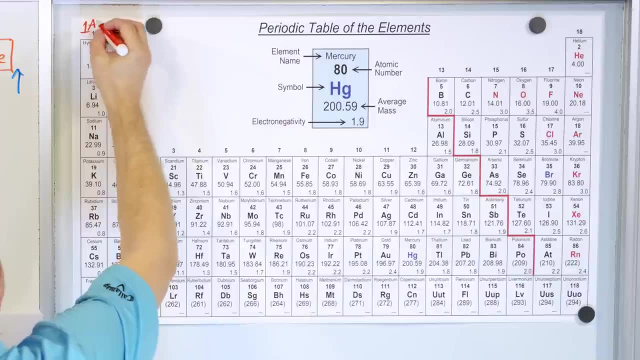 still use this, some literature still use this, but in general, we're going to use these numbers down here, But depending on what you're using, you may see something different. So I'm going to show you something different. This column was called column 1A and this column was called 1B. 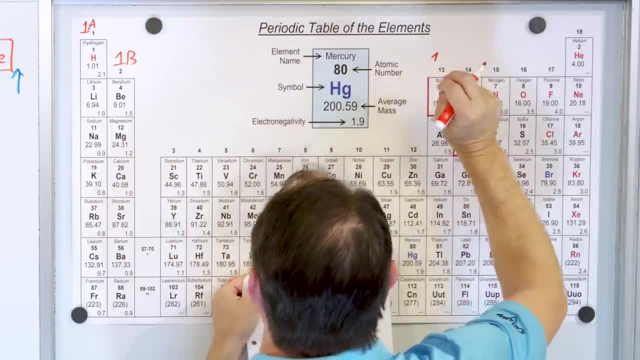 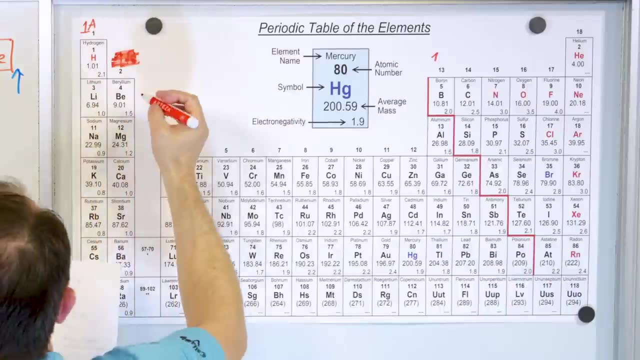 And then when you skip all the way over here, you have. you have actually sorry about that. I apologize for that. I'm on autopilot and made a mistake already. So this is 1A and this was going to this column. when you look at, another book will be 2A And then over here this will be 3A. 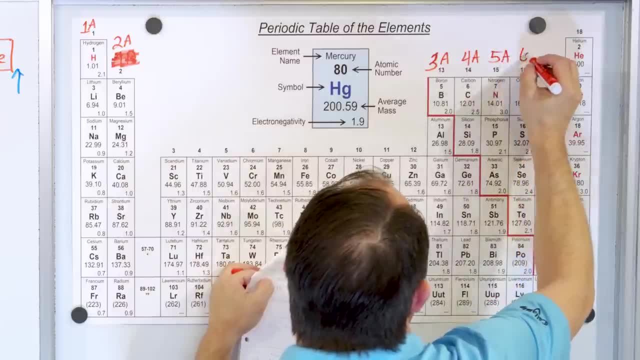 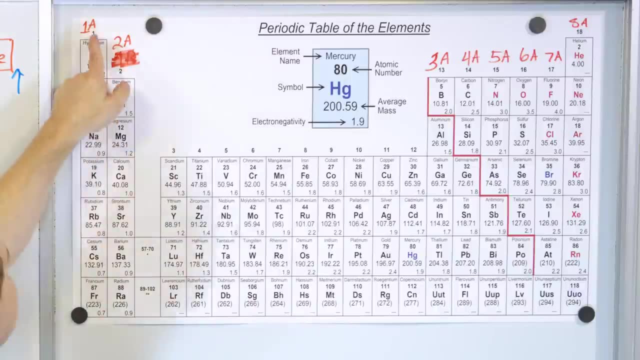 and then 4A, and then 5A, and then 6A, and then 7A, and this one over here was 8A. So first of all, you notice something different. There's this A business here. You'll. 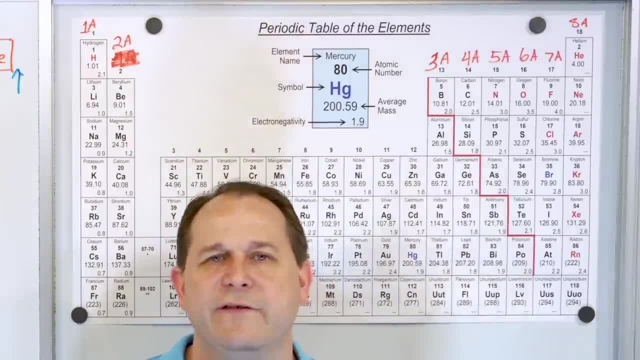 understand why in just a second, but I just want to. I just want to call to your attention that, depending on what book you might be using or what, what periodic table you might be using, you might see different labels up there. It's just a label. Who cares if we call this group 2A or? 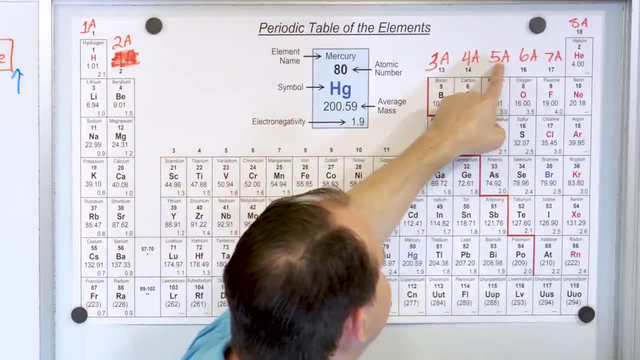 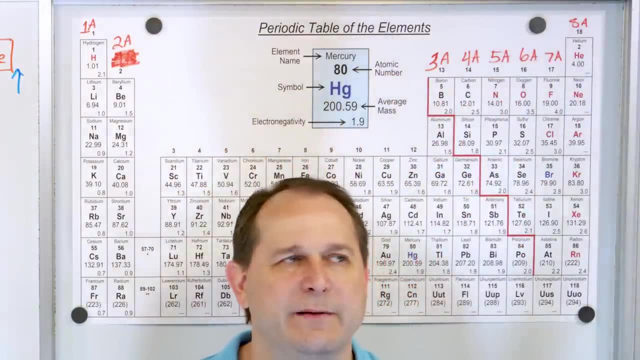 group 2?? Who cares if we call this thing group 15 or group 5A or group 18 and group 8A- And you'll understand more about the numbers here later. It again has to do with electrons. It depends. 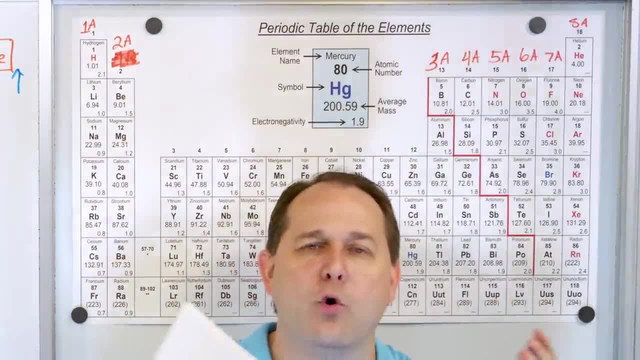 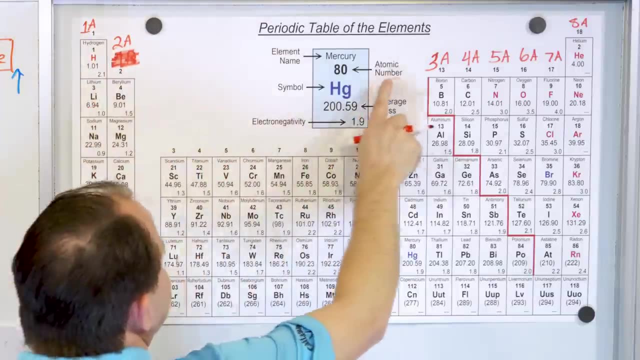 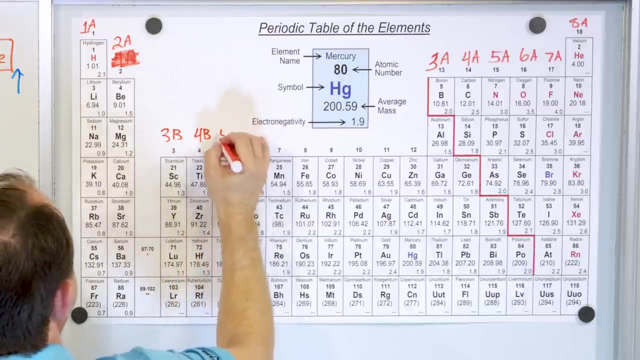 it has to do with how many electrons fit in around in the orbitals around the atom. okay, But down here below- I'm not going to fill this entire table out- but this is 1,, 2, and this is 3A. This one down here was 3B, and this one here was 4B, and this one here was 5B, And so these: 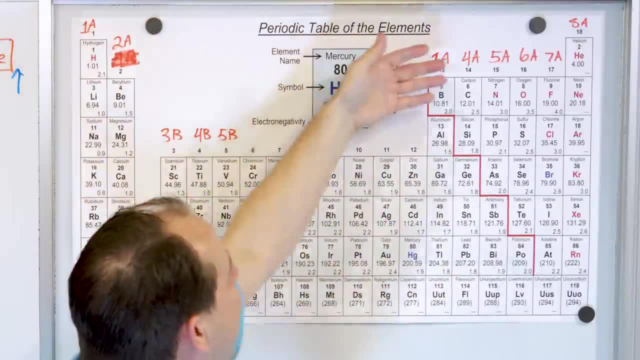 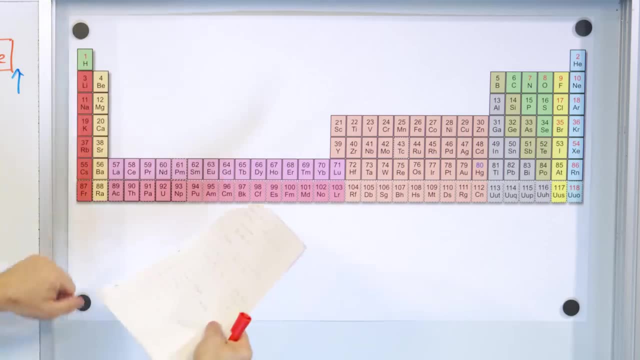 are the Bs here And again, the reason why there's an A, a set of A elements and a set of B elements is because of how the electrons are. I told you just a second ago that the reason this table looks the way it is with these weird blocks here that are set down and this is spaced out. it all has. 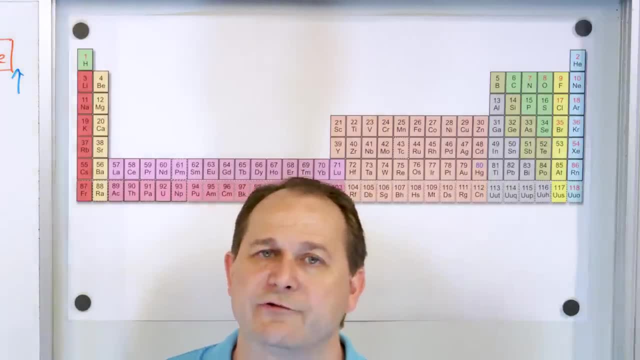 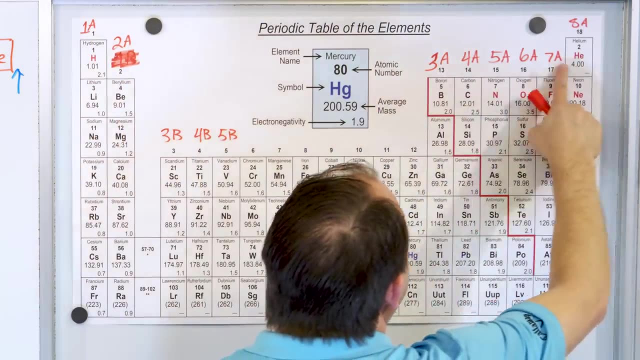 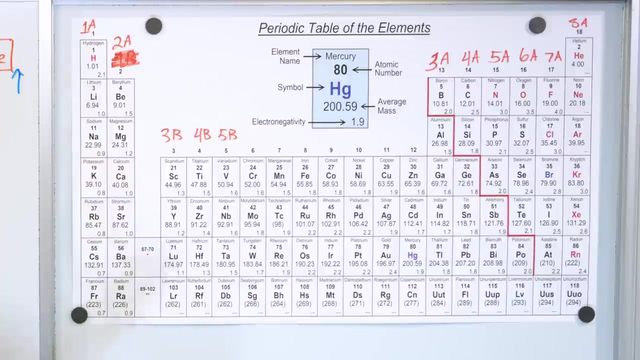 to do with, when we talk about electron configuration, how the electrons fill up. For the exact same reason, when they did the original labeling, they called some of these A group or A groups, and that has to do again with electrons, and some were the B groups, and again that has to. 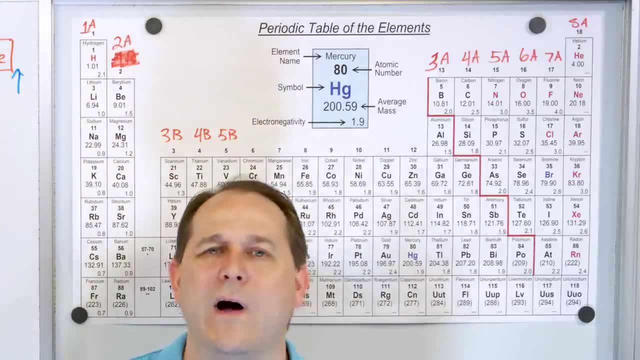 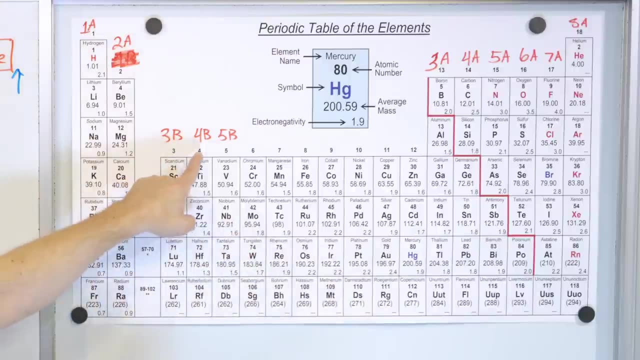 do with electrons For our class. I don't want to get into the history of why it was done that way. I'm just letting you know that, depending on the book you use, some people might refer to this as group 4, and some people might call it 4B. Some people might. 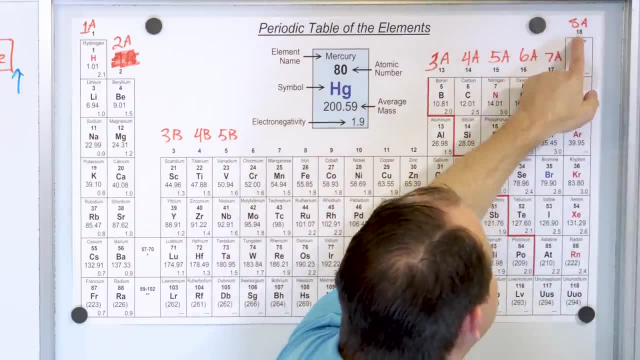 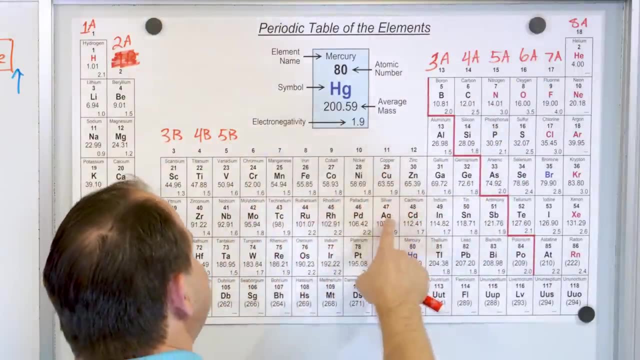 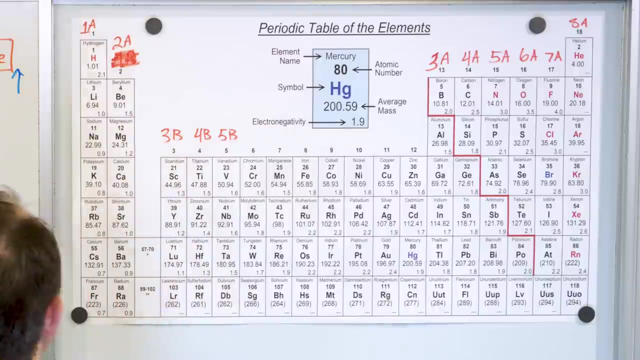 call the noble gases group 8A and some people might call them group 18.. And then we have the different labeling there as well. We talked about copper, silver and gold being the coinage group, because we used it to make our coins. And then there's a couple of other things I want to talk. 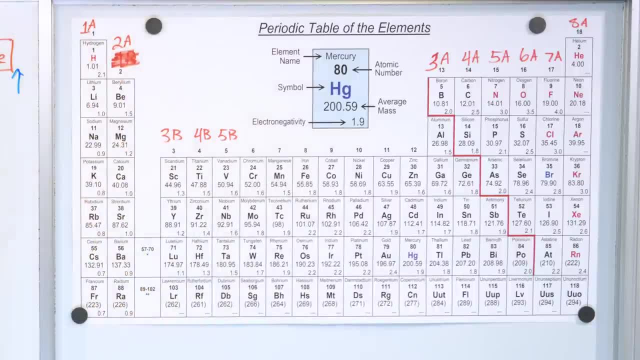 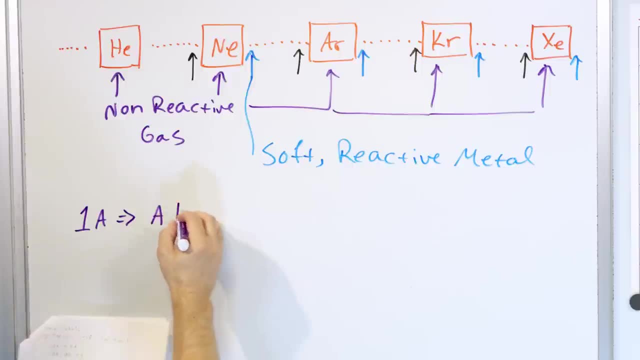 about Group 1A. is this column Group 1 or group 1A, however you want to call it, or however you want to refer to it? these have a special name that you're going to see, which is called alkali. 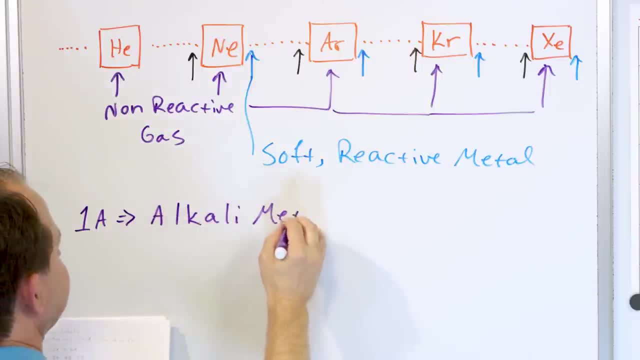 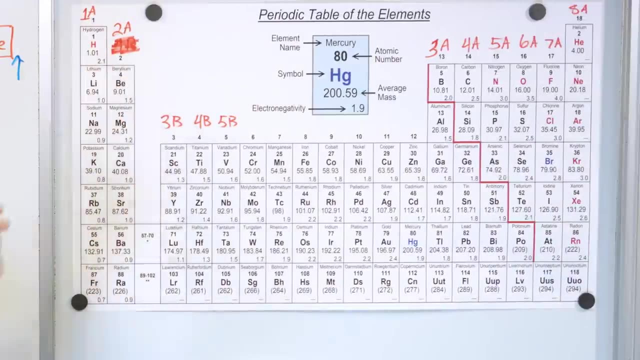 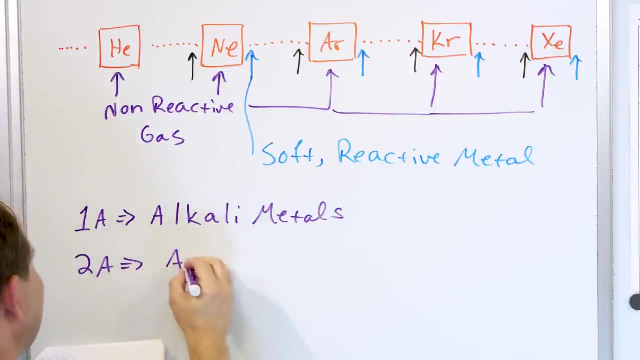 metals. So if you're ever in a book or just reading a research paper and something talks about the alkali metals, you know it's got to be one of these here. And then we have group 2A, which is not alkali, it's called alkaline. 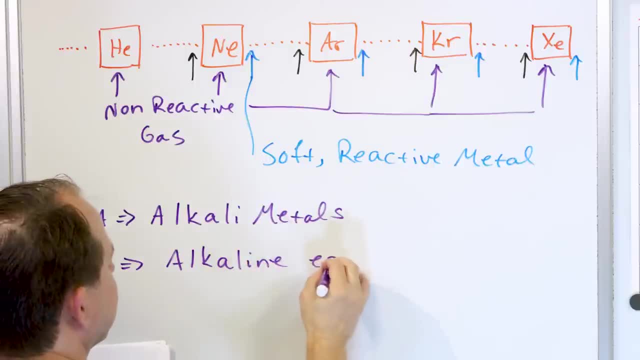 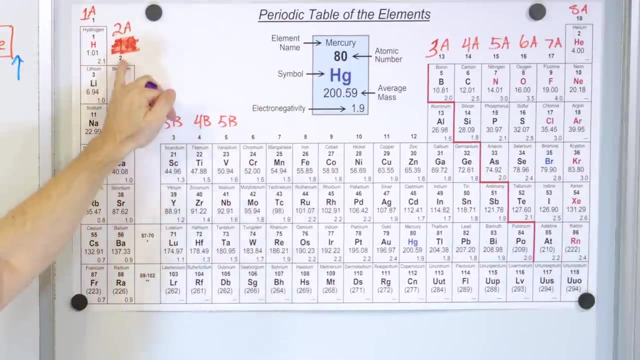 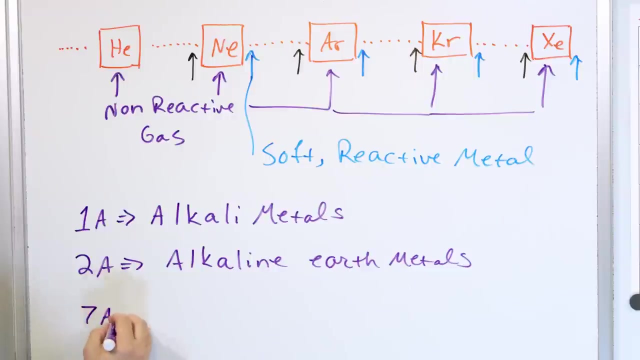 earth metals. So we have the alkali metals here and we have the alkaline earth metals right next door. It's just something you might see referenced, that's all. And then over at 7A we have the halogens. 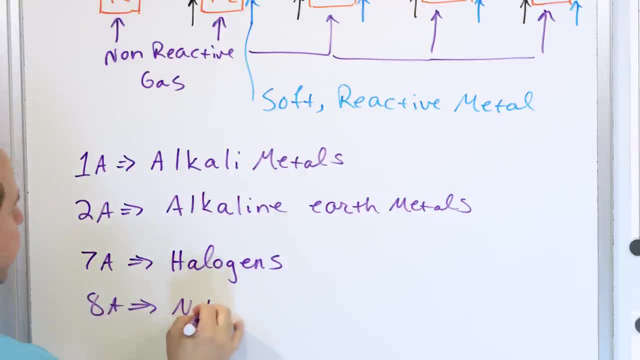 And over here at 8A we have those noble gases. There are other names for other groups, but these are the most important ones. You have the alkali metals and the alkaline earth metals on the left side of the table, And then you have 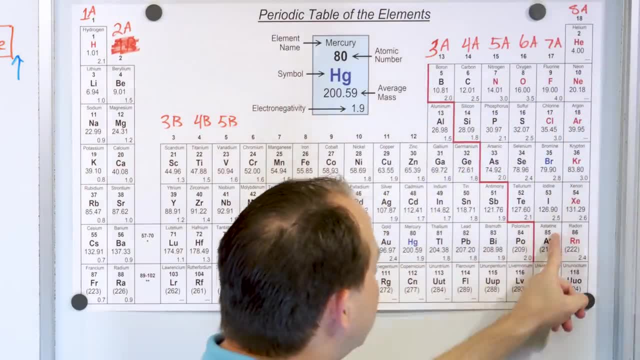 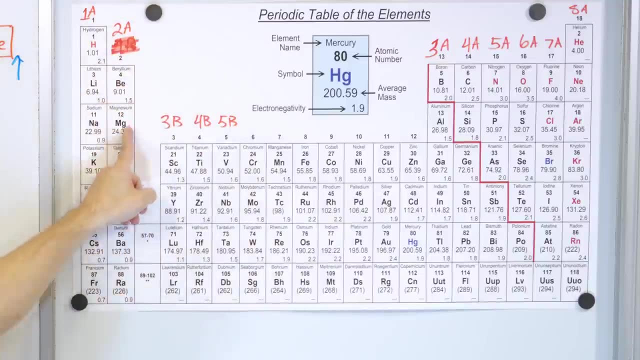 the halogens and the noble gases on the right side of the table, And then you have the alkali metals on the right side. So this group right here is called the halogens And this group is called the noble gases, And this group is called the alkaline earth metals And this one's called the alkali. 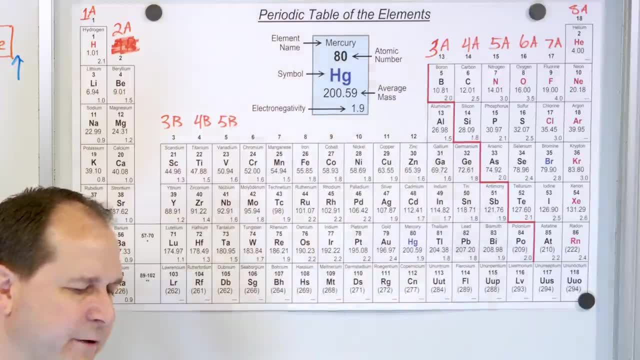 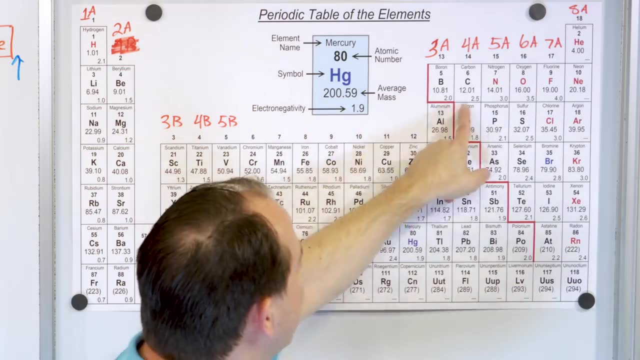 metals. All right. What else do I want to say? Metals are on the left. We lose electrons on the left of the table. Non-metals are on the right. We gain metals over here. Metalloids are the elements that are near the stair-step line, because they have properties of metals and non-metals. 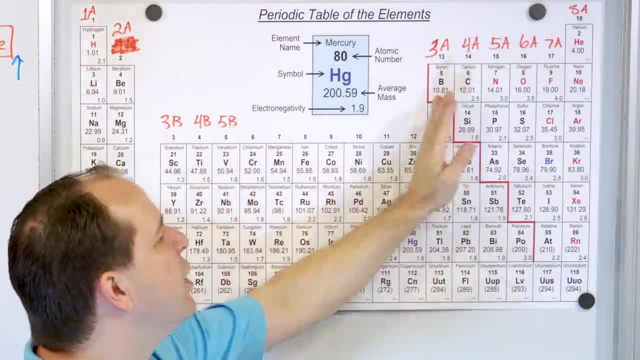 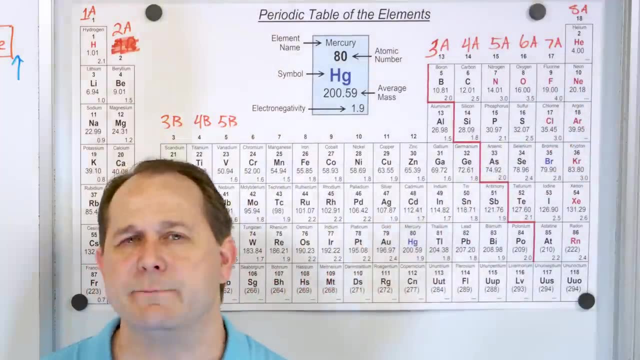 So, in general, as you start here and work your way to the right of the table, you get more and more non-metallic-like eventually until you reach the complete non-metals. And what is the difference between a metal and a non-metal anyway? In general, a metal is. 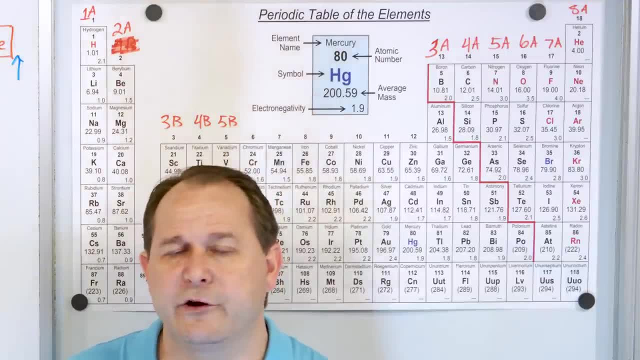 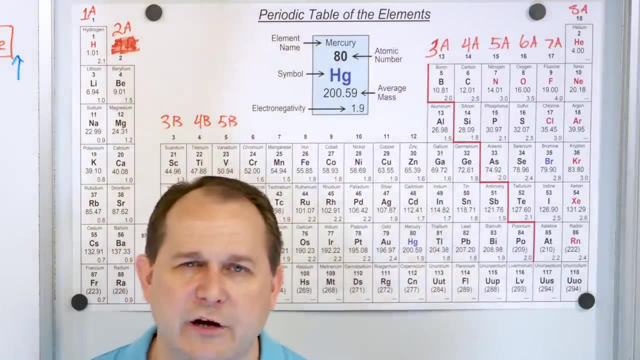 something relatively shiny, has some luster, It's pliable and ductile. You can usually draw it into a wire of some kind, right? It's usually a good conductor of electricity and a good conductor of heat. And these, in general, are the elements on the left-hand side of the periodic table. 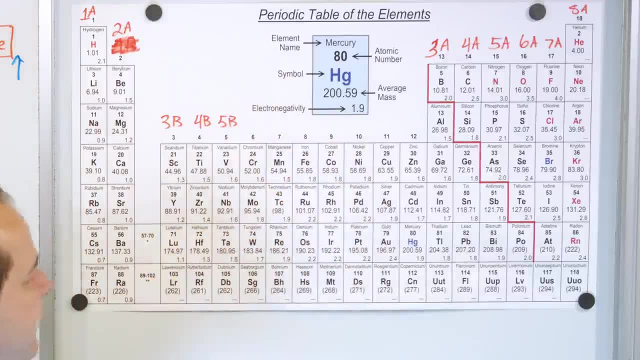 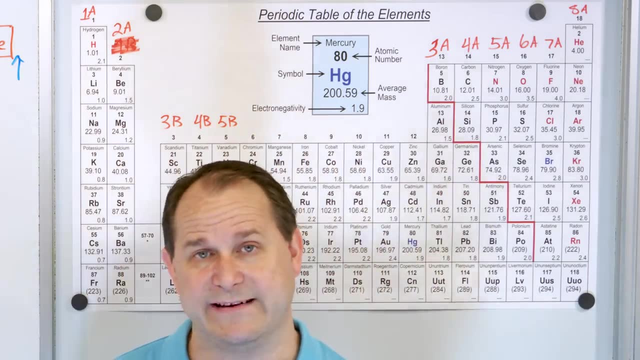 All right, You can see the copper. Everything we make wires out of is on the left-hand side. These are metals, And, of course, the ones in the middle. we call them transition metals because we're transitioning from the metal side to the non-metal side of the table. Now, in your mind, 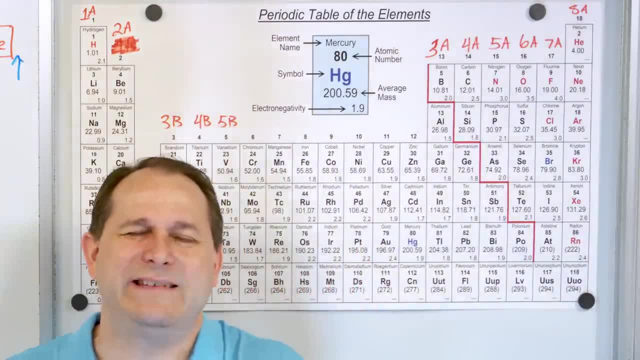 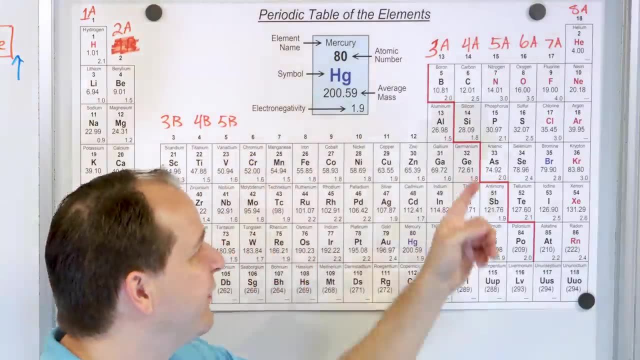 what is a non-metal? A non-metal is something that's not metallic in the sense you can't draw it into a wire. It's brittle. If you try to pull on it it's probably going to break. Think about charcoal, which is carbon. If you just think of carbon like a carbon briquette, you could break. 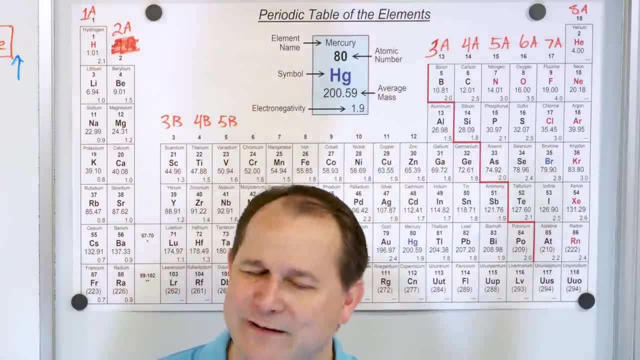 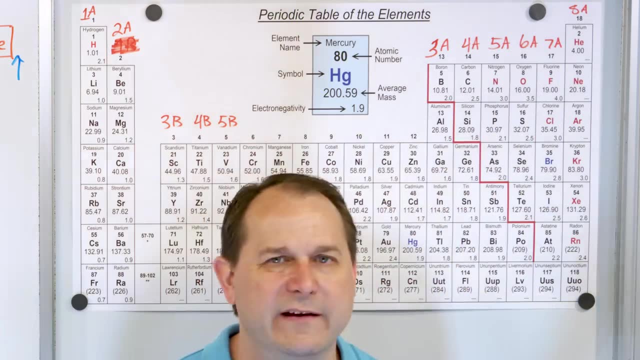 it. If you try to pull on it it's going to break, right. They're not shiny or ductile, You can't pull them. And also gases: Gases are non-metal, So you have a lot of gases over here, like oxygen. Of course it looks. 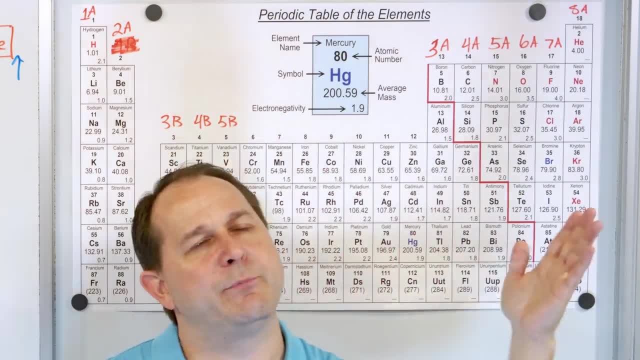 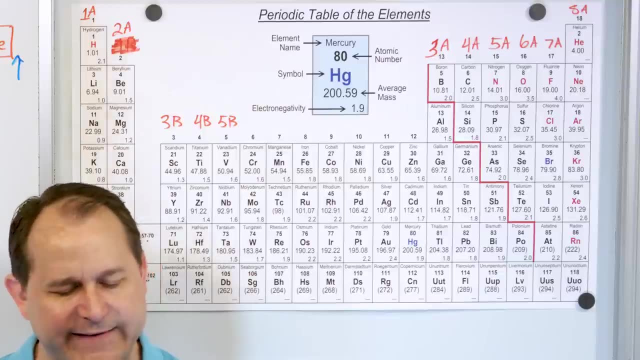 nothing like a metal. So as you move from left to right along the periodic table, you get from a metallic character gradually transforming to the non-metallic character on the right-hand side, And the last thing we'll say is that the groups up here that have the A's up here, 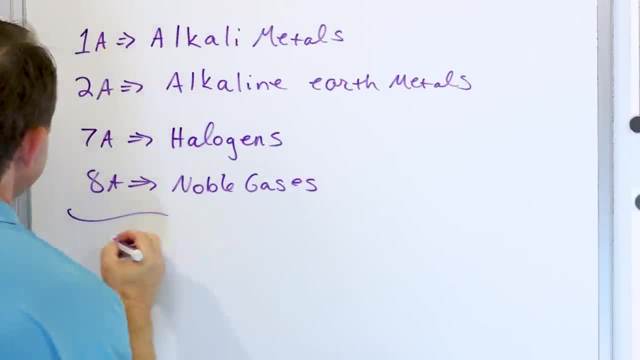 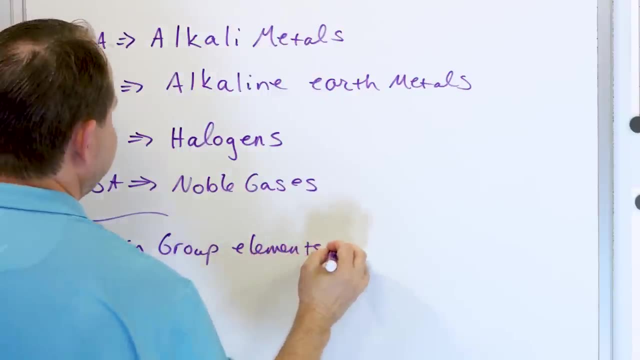 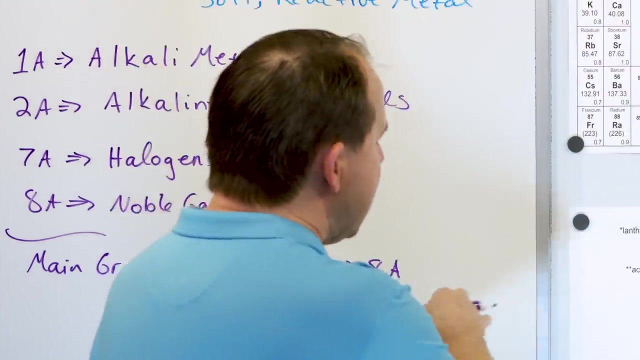 these are called the main group elements. I guess I'll write that down: Main group elements And just to help us remember that's 1A through 8A, 1A to 8A- Those groups. Now why do we have a special label for the main? 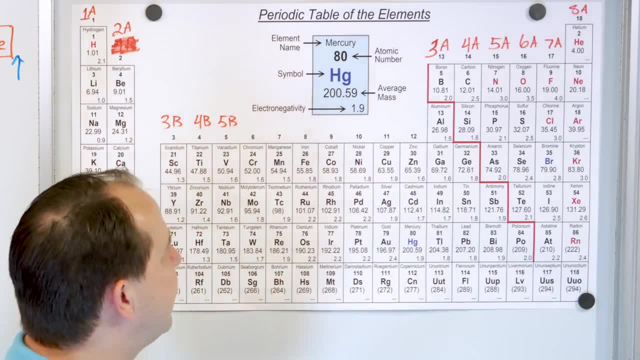 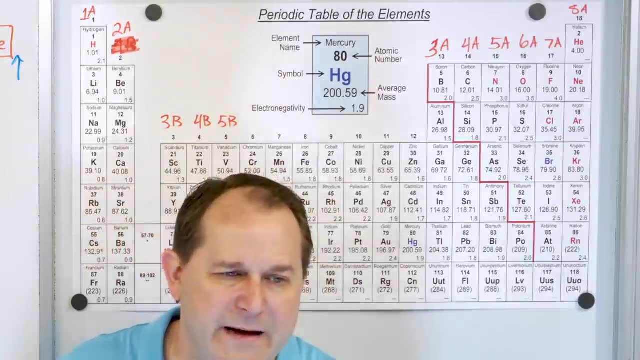 group elements over here like these and then these, and you exclude everything else. That is because those elements are what we're mostly going to be concerned with in a beginning chemistry class and even in organic chemistry- Again, the chemistry of life, the complexity we have around. 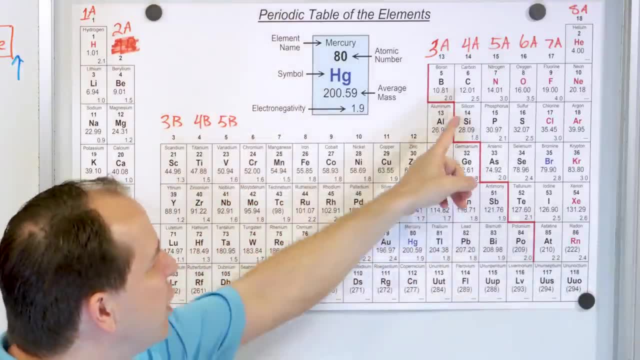 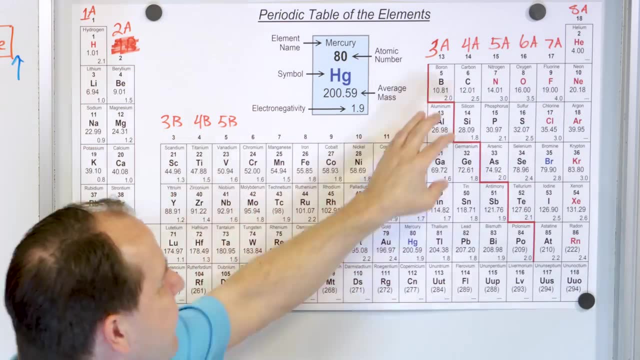 this really is only a handful of elements that participate in that. It's mostly carbon nitrogen. there's some other things that are involved as well, depending on what you're talking about, But generally life is concerned with a handful of elements there, plus the hydrogen. 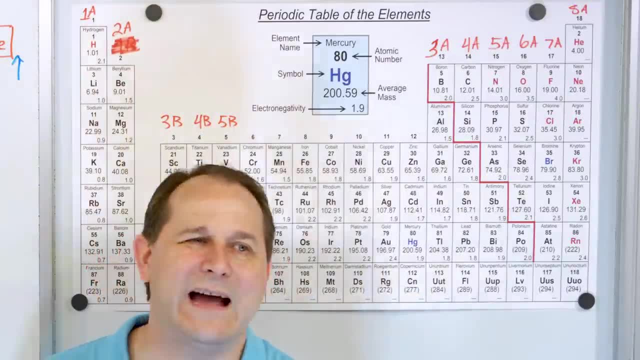 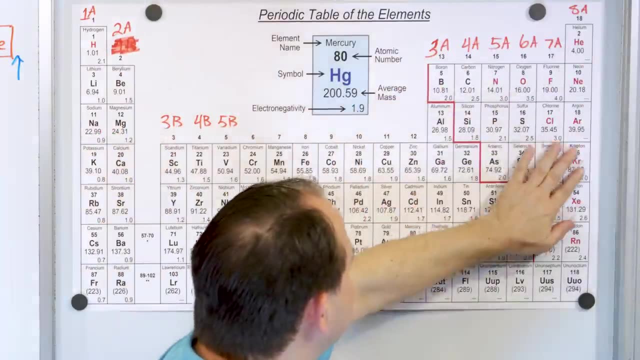 And then you have other things like salt, sodium, chloride, calcium for your bones, things like that. These are in this column here. So this column is very important And these columns- or groups, I should say- are all very important. These are important as well, but they're kind of 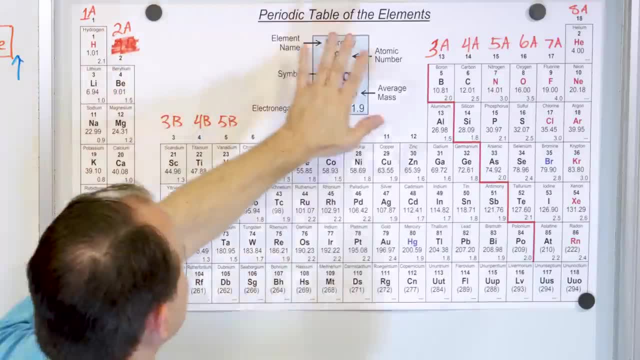 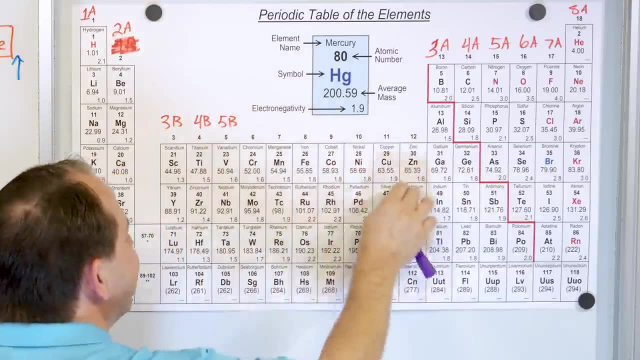 secondary. They're important for other things. So we call these the main group elements because we really are going to focus on these And we're going to focus on these And we're going to focus on these mostly in this class. We will, of course, do problems and talk about what happens with these. 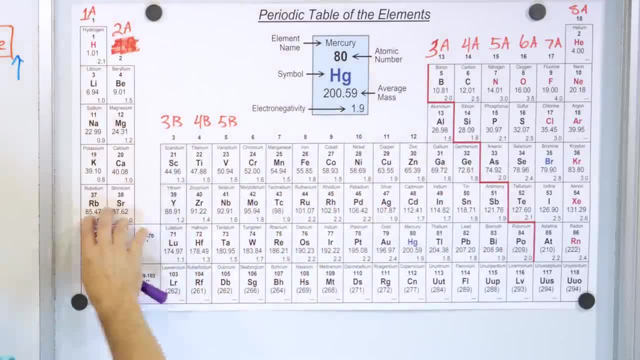 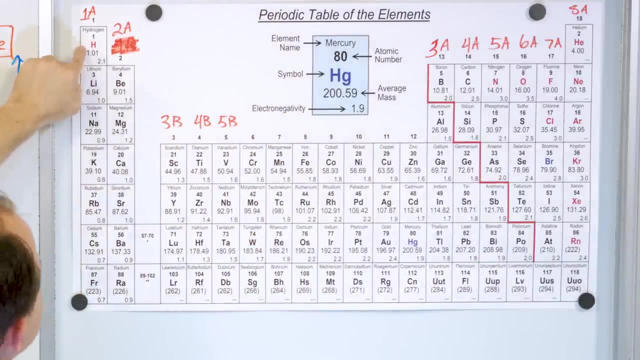 But mostly you study that stuff a little later in more detail. These main group elements are more important for us here in the beginning. The last thing I'm going to say before we actually solve our problem is that: notice, hydrogen is over here hanging out with the metals. These are all. 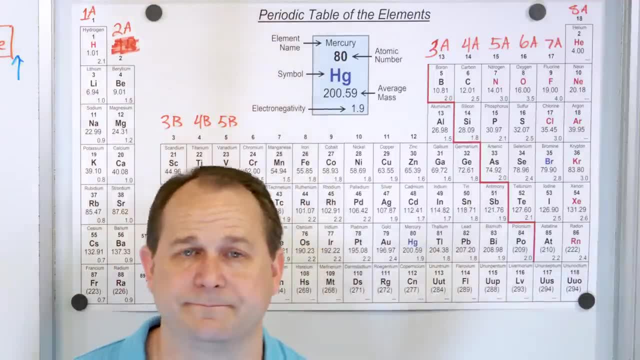 metals and hydrogen is over here. Obviously, hydrogen is not a metal, But the reason it's over there is because hydrogen is a little bit of an oddball. It's the lightest and the simplest element we have. There's only one proton. There's only one hydrogen. There's only one hydrogen. There's. 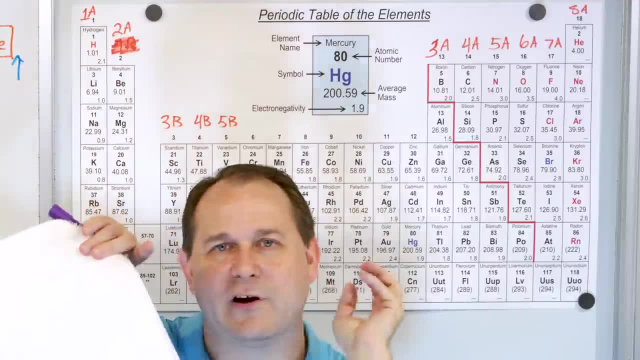 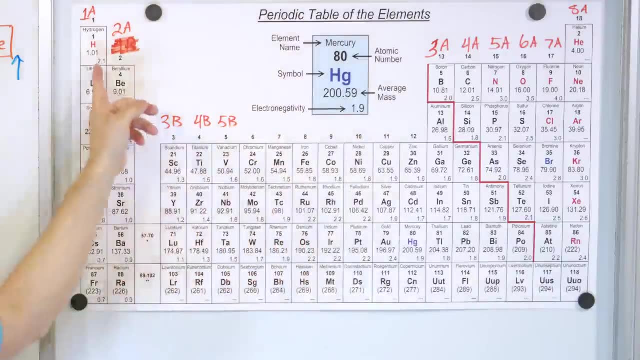 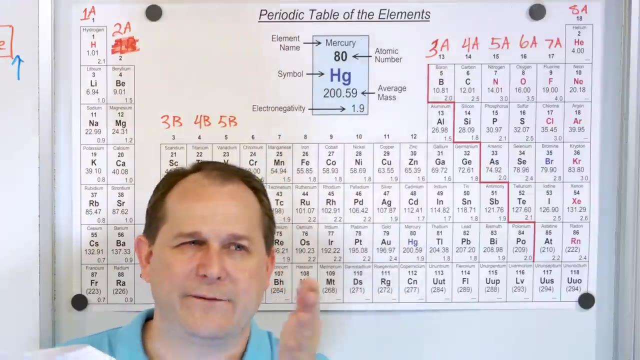 a nucleus and one electron. It's just one proton, one electron and that's it. And what happens is hydrogen can go both ways. Hydrogen can lose electrons, just like the metals do here, can lose electrons, or it can also gain electrons as well. So because it gains or lose electrons, you've got. 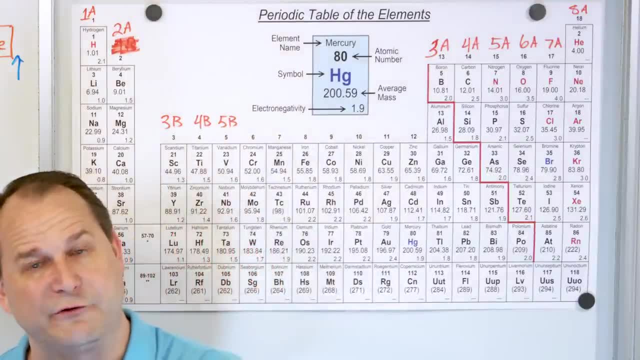 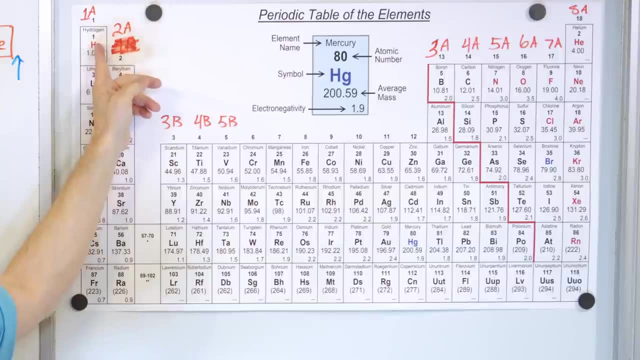 to figure out where to put it, because you know, generally the metals like to lose the electrons and the nonmetals like to gain electrons. But hydrogen can do both, depending on what's going on. So we just kind of put it over here in the metal column, even though it's not really a metal. But 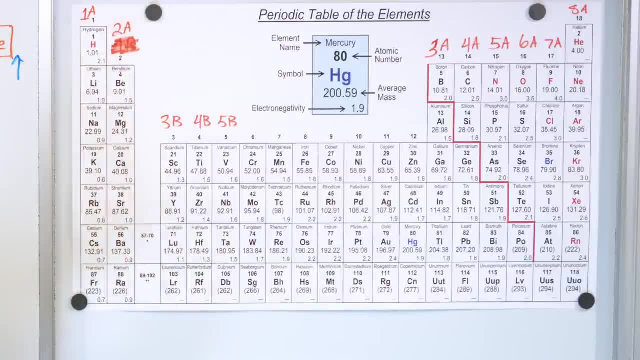 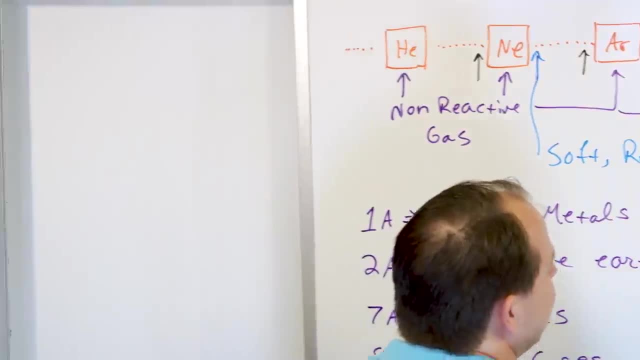 it does, it can behave like a metal, So that's why it lives over there, All right. So now that we have that done, what we want to do is we want to solve a quick little problem, which is going to be very simple, And this problem is going to be that I'm going to write an element on the board. 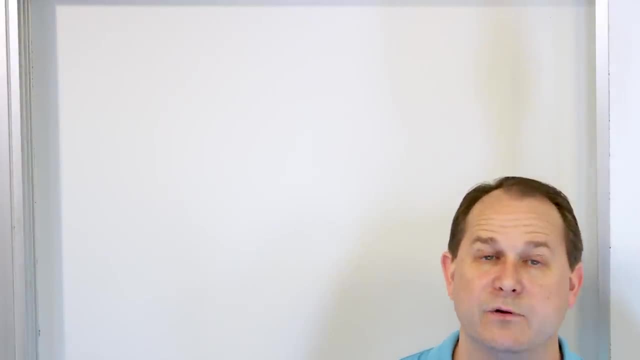 And then what we want to do is classify it as a metal, a nonmetal or a metaloid. All right, So the first one, chromium. So let's take a look at chromium. Right? So we want to. we want to write down the, the symbol for the element. We want to write down its atomic number. 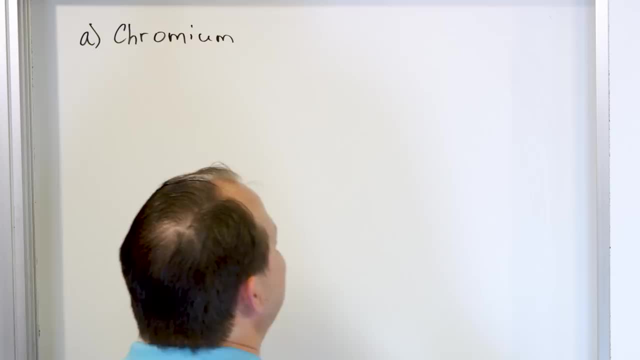 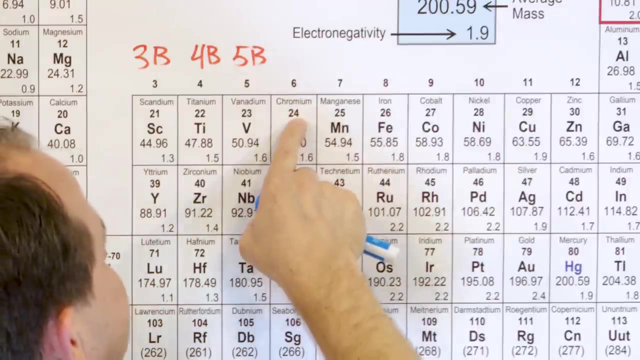 and we want to also classify it as a metal or a nonmetal. So just getting practice with the periodic table, So chromium. So chromium is right here. It says chromium and CR is the symbol and 24 is the atomic number. That means chromium has 24 protons in the nucleus And for the neutral, 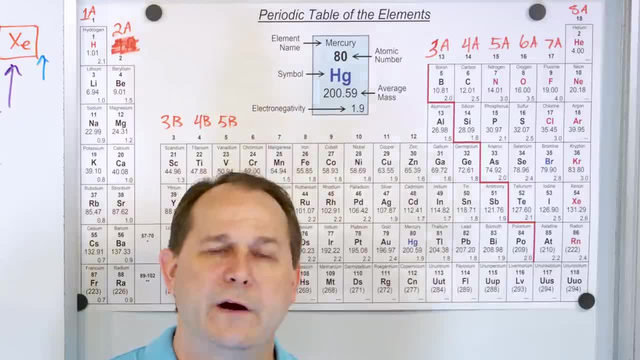 atom of chromium. it has also 24 electrons. There also are neutrons in the nucleus, but these don't tell us how many are there. Different flavors of chromium, which we call isotopes, can have different numbers of neutron. neutrons that are there, But as far as the protons in the 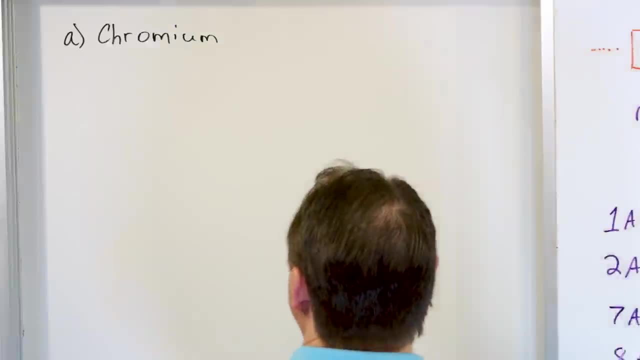 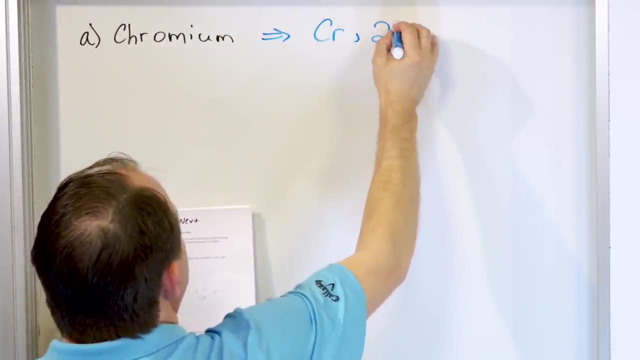 nucleus, it has 24 and 24 electrons to balance it out. So chromium, the symbol, there is CR and there's 24 for the atomic number, And it's a metal. It's not to mention that part. Why is it a metal? 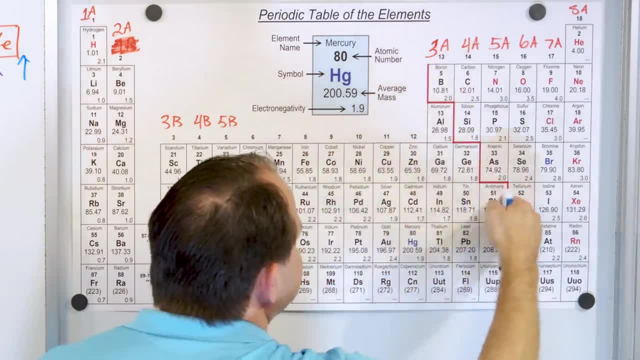 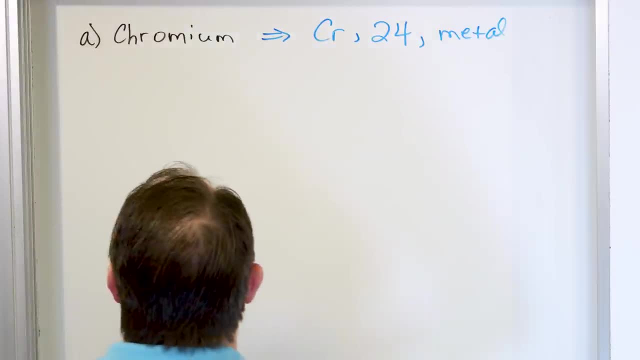 Chromium is a metal only because it's on the left-hand side of the periodic table, to the left of the stair step boundary. Okay, So I think what I'm going to do next is I'm going to write down the remaining ones here and then. 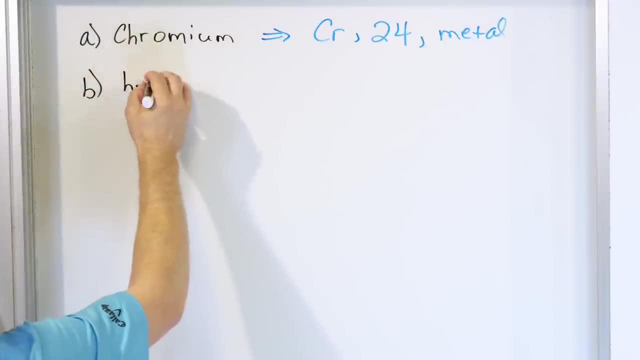 we're just going to look them up. So next we're going to do helium, And then after that we'll do phosphorus, And after that we'll do zinc, And then after that we'll do magnesium, And then after. 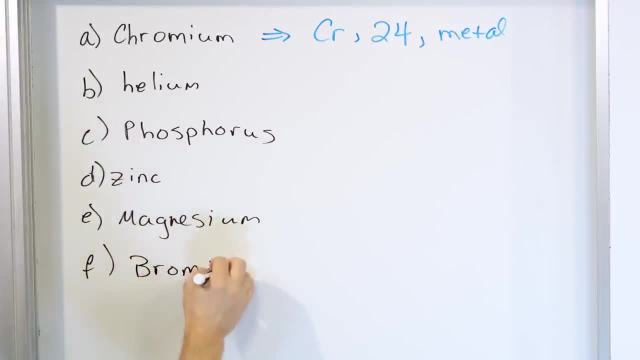 that we'll do bromine And then after that we'll do arsenic. Don't want to eat any arsenic, Not good for you. All right, So let's go take a look at helium. Is it a metal, Is it a non-metal? What's its atomic number? So here's. 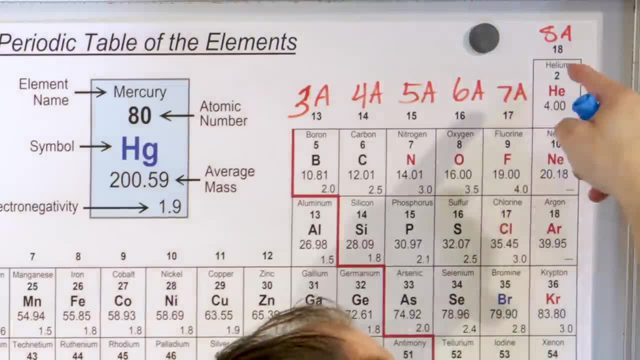 hydrogen. All the way. on the right-hand side of the periodic table is helium. It is a non-metal because it's on the right And it has two protons because its atomic number is two. The symbol is HE. How many electrons does helium like to gain or lose? Well, actually, helium is a noble gas. 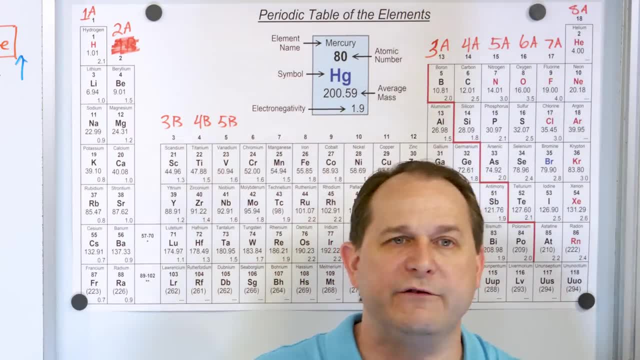 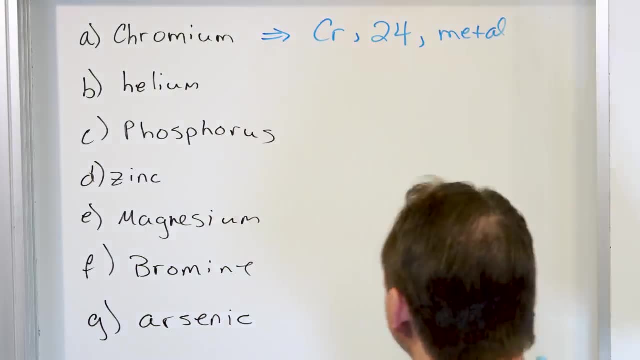 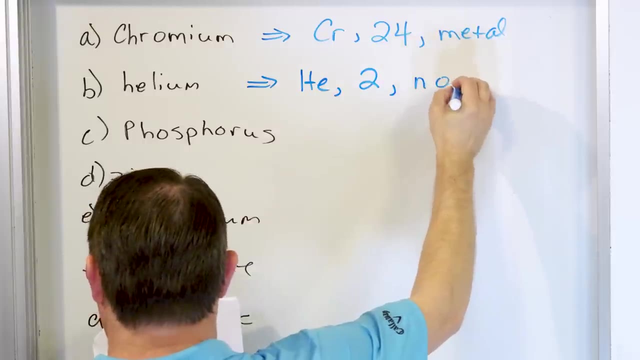 It doesn't gain or lose any electrons. It's a very non-reactive. It hangs out and it has its two electrons and it doesn't do anything. So it doesn't really like to gain or lose any electrons there. So, helium, the symbol is HE, The atomic number is two and it is a non-metal. All right, Next one. 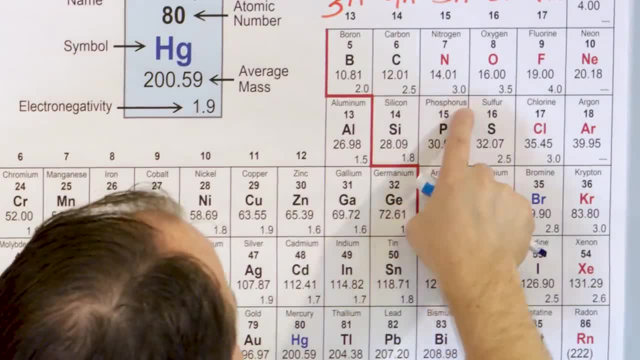 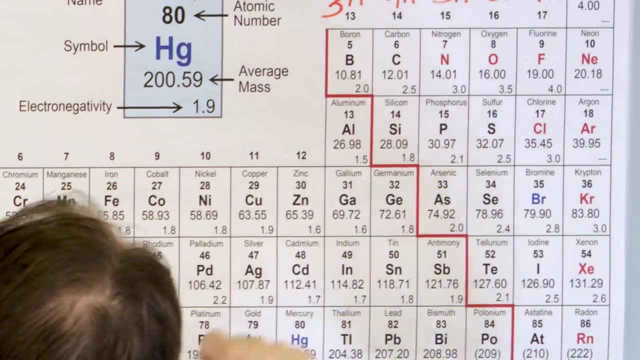 Let's take a look at phosphorus. Phosphorus- right here It says phosphorus, Symbol is P, The atomic number is 15. And so that means 15 protons in the nucleus and 15 electrons surrounding the nucleus, And it's a. 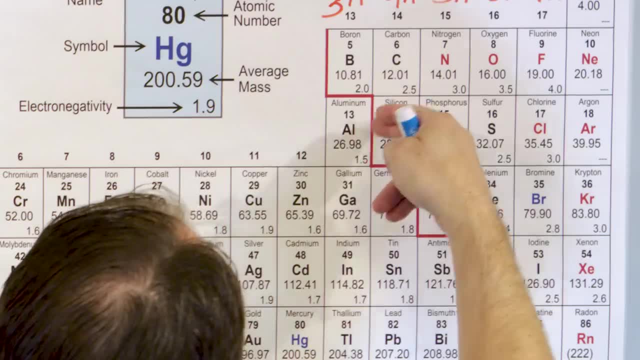 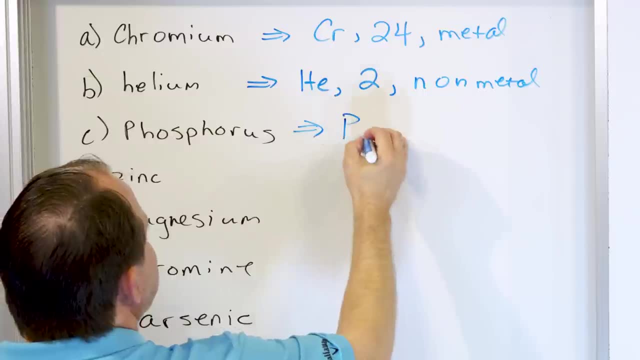 non-metal Because it's to the right-hand side of the periodic table, It's not really on the border here. So it's not a metalloid, It is a non-metal. So symbol is P And there are 15 protons in the nucleus, atomic number. 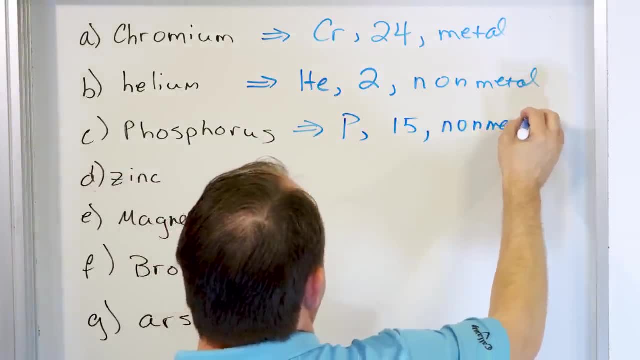 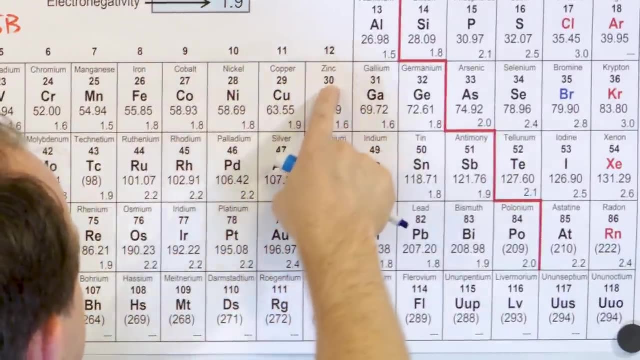 15. And it's a non-metal. Okay, Next let's talk about zinc. Where does zinc live on this periodic table? We look over here for zinc. Here it is Zinc atomic number 30. And the symbol is ZN. 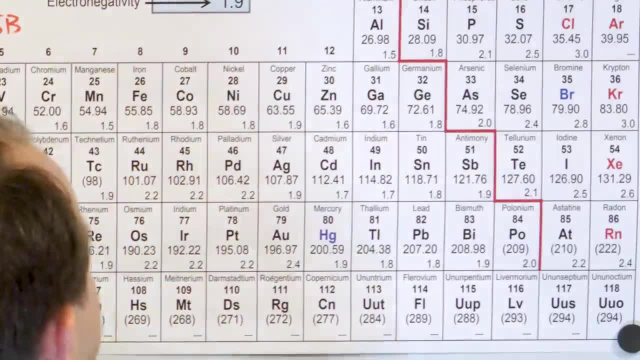 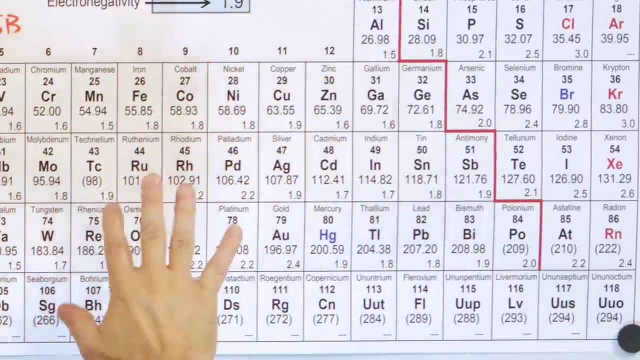 And it is a metal because it's to the left-hand side. Now we know that zinc likes to lose electrons, because in general, all these metals like to lose electrons. But exactly how many electrons zinc loses, you can't really say so much from the periodic table. 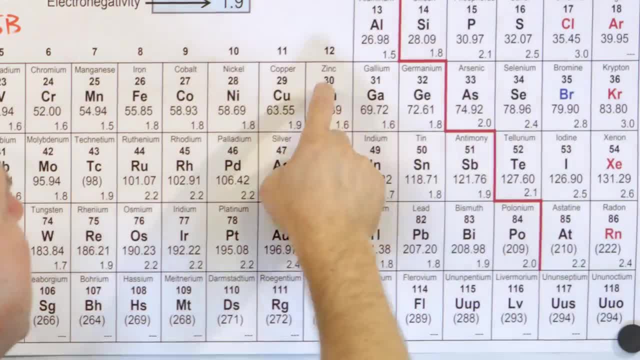 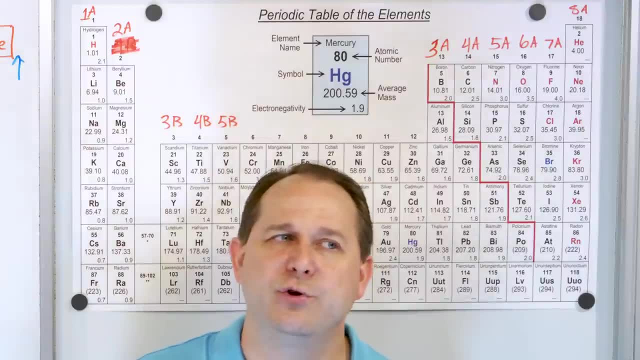 The ones on the edge are very easy to predict. They're very reproducible. But zinc you have to maybe look it up in a table. You'll probably memorize it after a while of dealing with zinc. But I'm just saying that you can't just count based on the 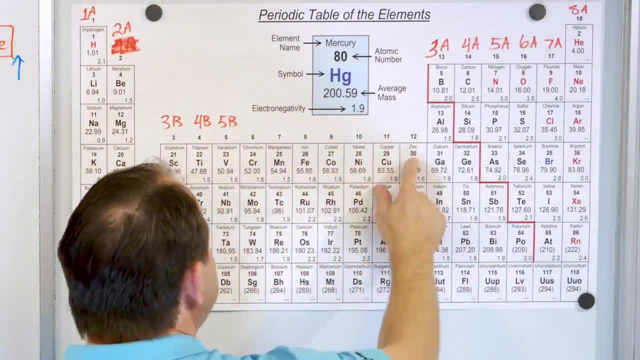 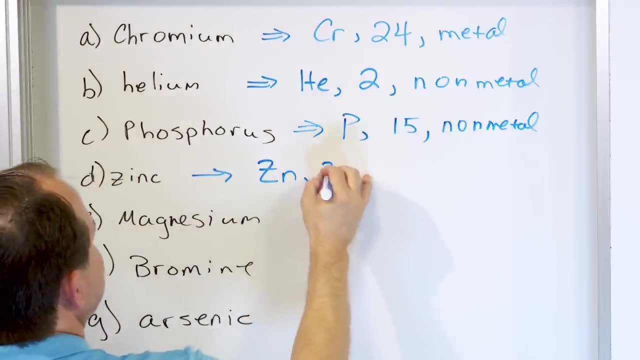 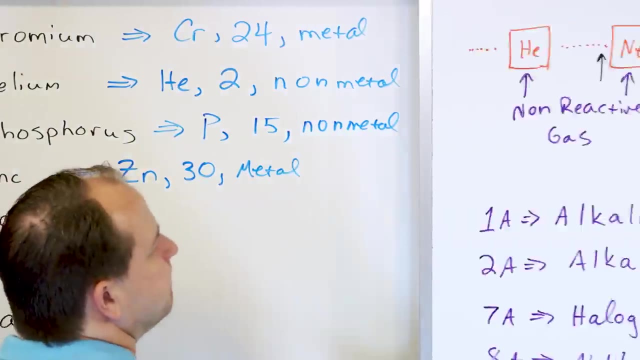 periodic table for the elements in the center there. So atomic number 30,, ZN is the symbol, All right. So ZN, atomic number 30, and that was a metal, And so because of that it likes to lose electrons, All right. What about magnesium, Magnesium? Magnesium is right here. 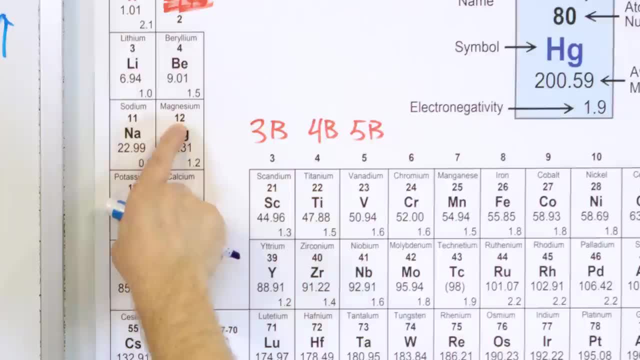 Is magnesium. Mg is the symbol, Atomic number is 12.. Now bonus question: How many protons does it have 12.. How many electrons does it have 12 electrons, And does it like to gain or lose electrons? in chemical reactions It likes to lose electrons. It wants to lose. If it loses one, it's going to lose electrons. 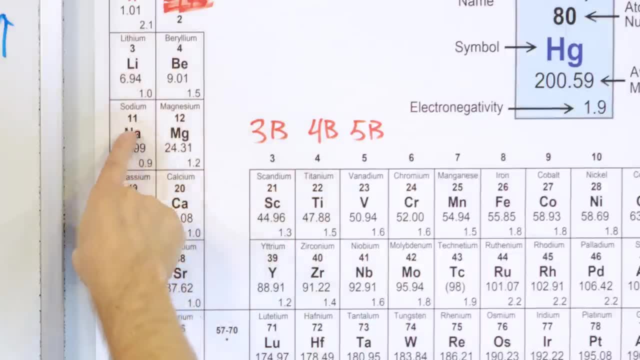 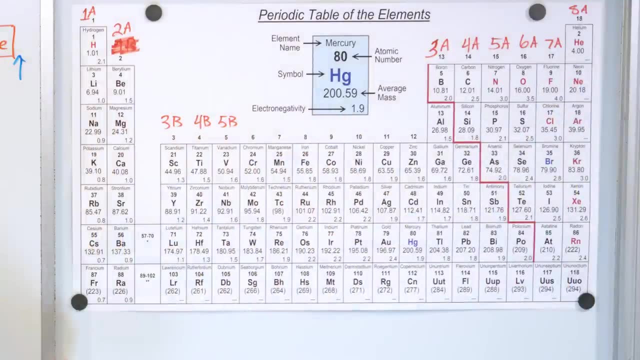 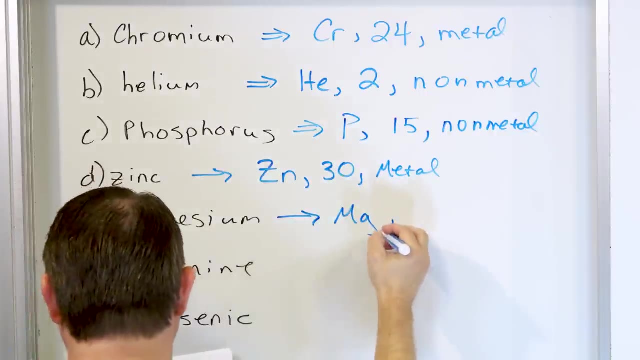 If it loses one electron, then it would have an electron configuration similar to sodium. If it loses two electrons, it'll look more like neon, So it always likes to lose two electrons. So what we could say is magnesium, the symbol is Mg and the atomic number is 12, and it's a metal. 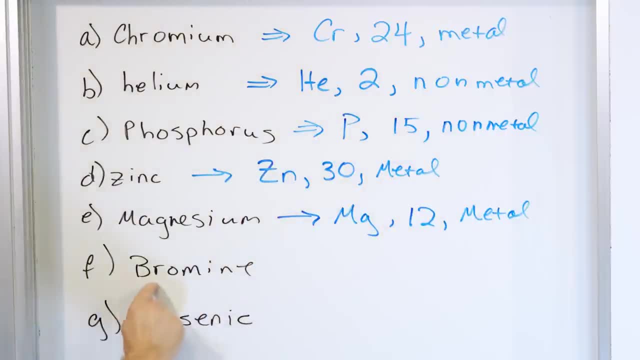 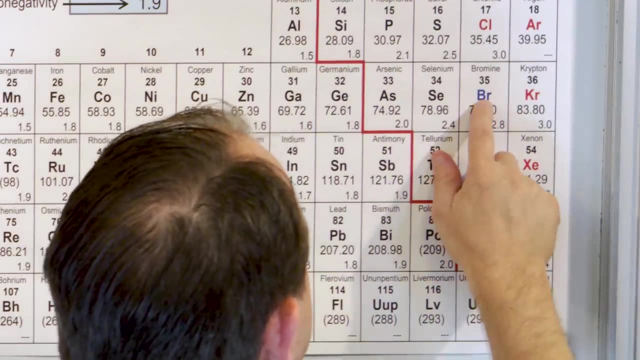 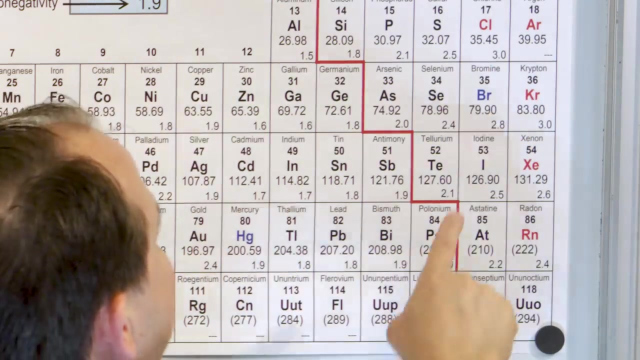 And it's a metal because it's on the left-hand side of the periodic table. What about the element bromine? What about the element bromine? So bromine is right here And its symbol is Br. Its atomic number is 35.. So 35 protons, 35 electrons, And it would like. 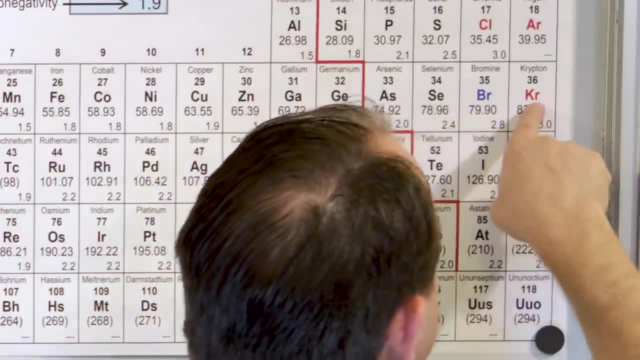 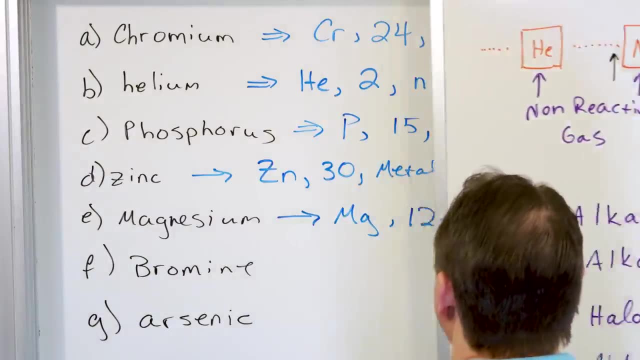 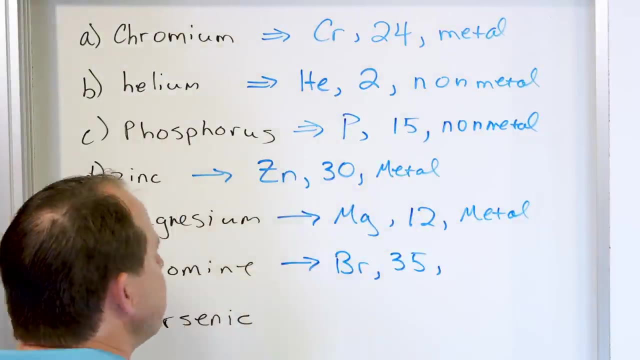 to gain one electron, to be as close as it can be to the electron configuration of krypton, which is right next door. So it likes to gain an electron there. So Br is the symbol, 35 is the atomic number. So Br is the symbol And 35 is the atomic number. Is it metal or non-metal? Everything on the right is non-metal. 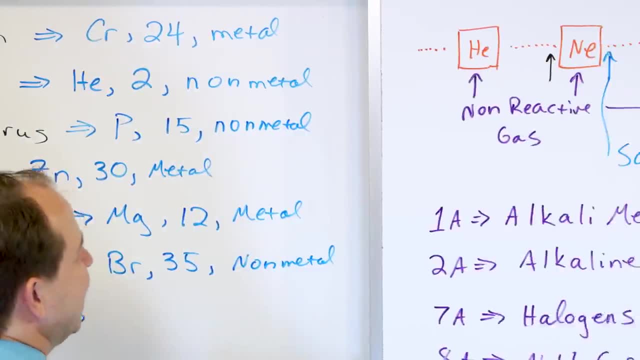 So that's what that is. And the last one here is arsenic. Don't want to eat any arsenic, it's poison. So where is arsenic Arsenic's right here? The symbol is As, The atomic number is 33.. 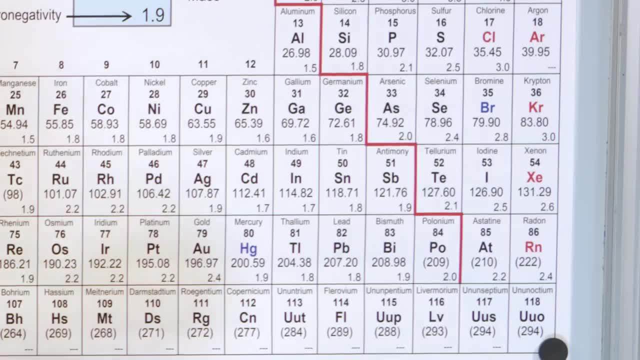 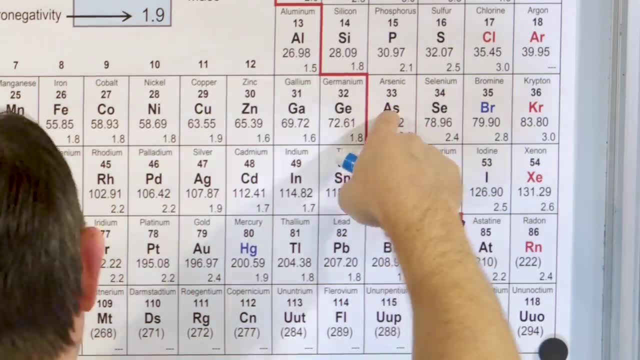 So 33 protons, 33 electrons, And is it a metal or a non-metal? Well, it's actually right on the border of this line here. So it's neither metal nor non-metal. It's what we call metaloid. 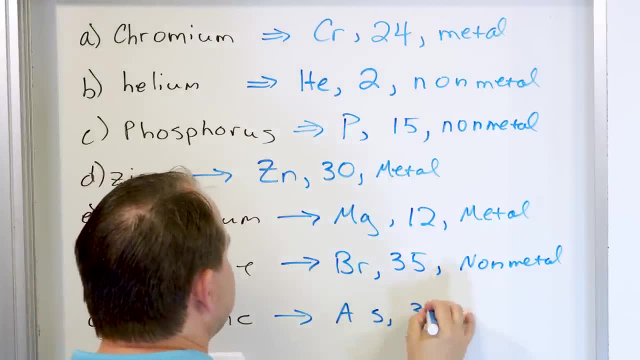 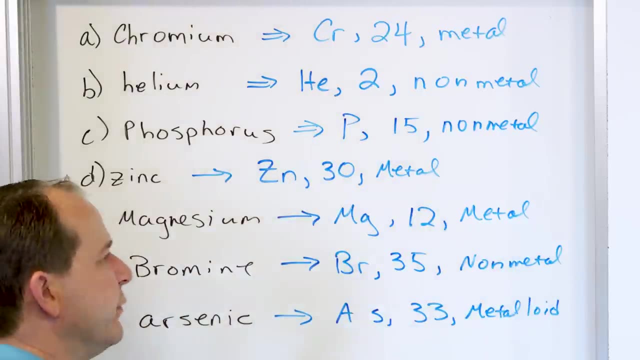 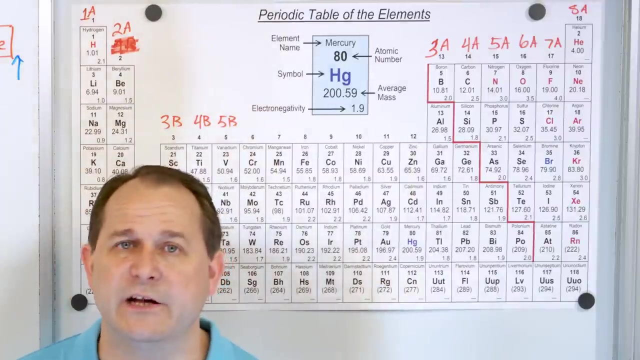 So atomic symbol is, As 33 for the atomic number, metaloid. All right, So in truth, this is the lesson that, when I started chemistry, I wish somebody had for me, Because these things that I'm telling you, these are, I mean, there's always. 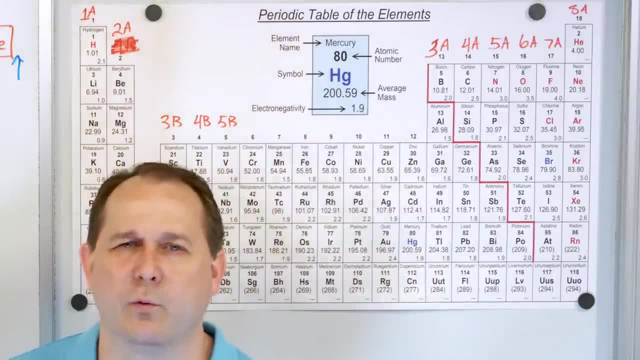 in every textbook, in every lecture that you have by a professor or whatever, or a teacher, you always have an overview of a periodic table. But these are the things that I think are the most important things about the periodic table. I could have broken this into probably two or three lessons. 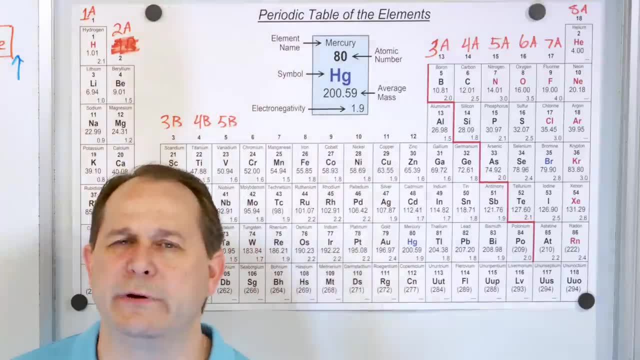 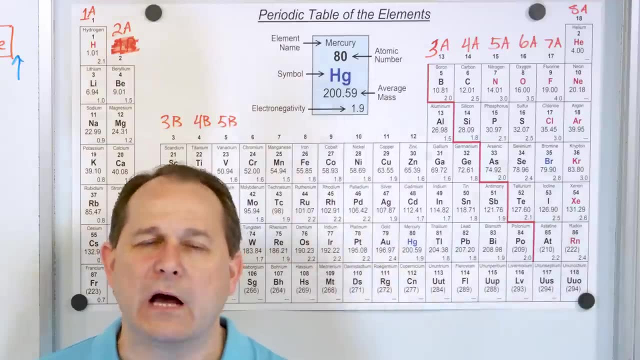 and made it shorter, but then you would lose the continuity of what I'm trying to say. The most important things for you to understand about this table is that it has the funky shape that it has because of the way electrons fill around these atoms, And we haven't learned that yet, so I can't really teach it to you. 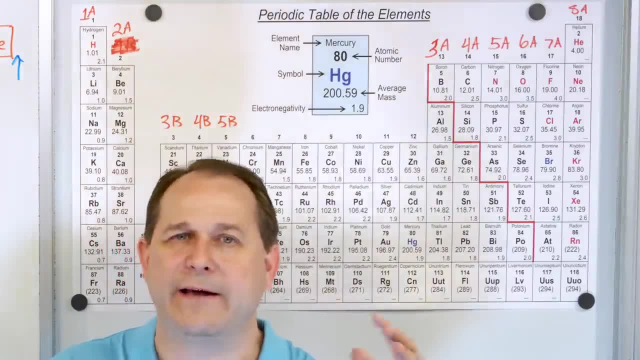 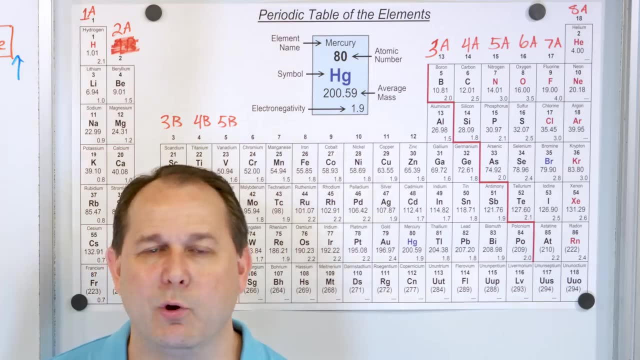 But trust me later on when I teach you how the electrons work and how they fill up, you'll understand exactly why it looks the way it does. But we got to get there right. Secondly, it's called the periodic table because as you increase the number of protons in the atoms, 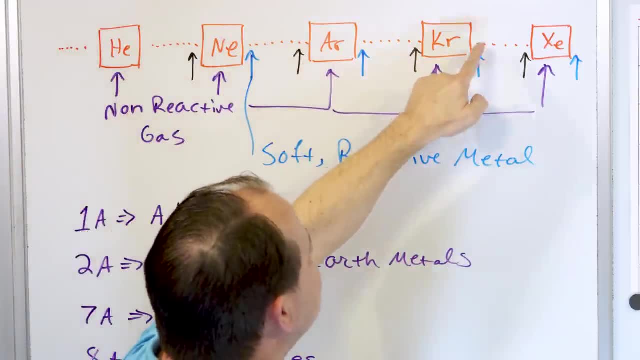 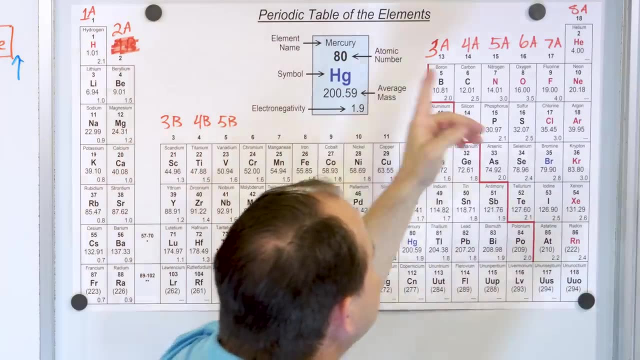 you're actually going to increase the number of neutrons in the atoms, And that's the thing you'll notice when you start to think about this. And that's why we have these special gases which are usually spaced, which we now call noble gases. They don't react with anything. And now we 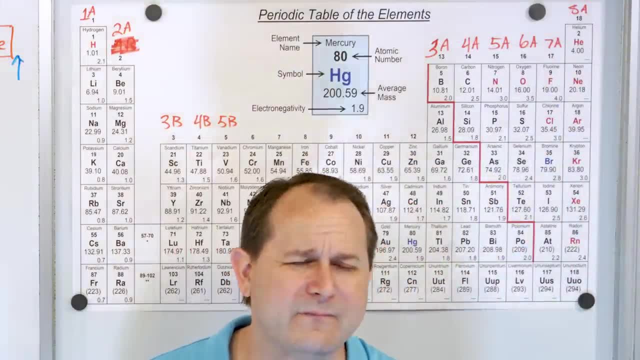 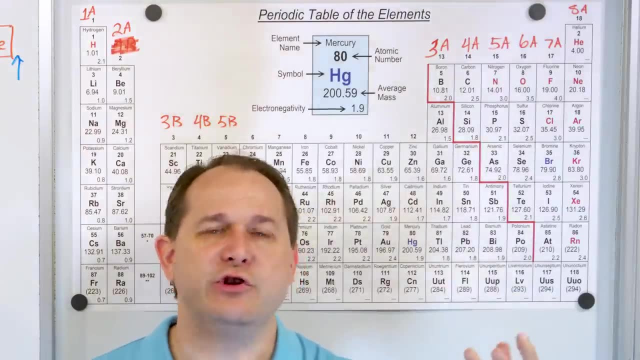 know that they're that way because they don't have, or because they have a very stable electron configuration. They don't like to gain or lose electrons. When I say stable, I mean the nucleus can hold it very tightly. I mean the nucleus of those guys, the way the electrons are distributed. 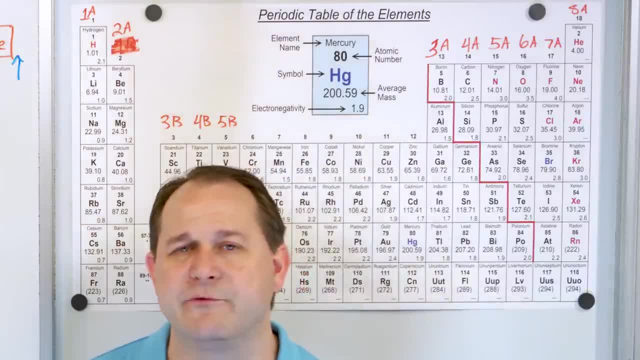 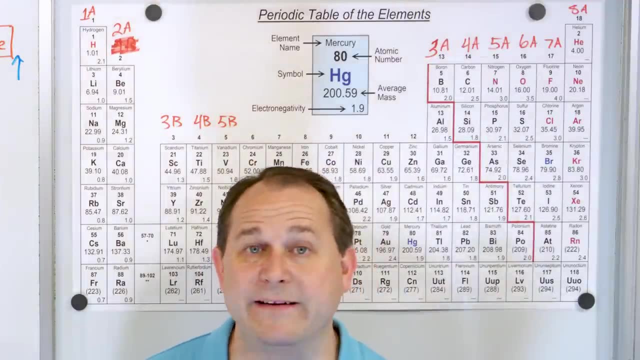 the nucleus is able to hold them all very tightly And because the electric force in these atoms is so incredibly strong- millions of times stronger than gravity- we've said that a million times- because of that it can hold these electrons very tightly and not let them go. that's basically the 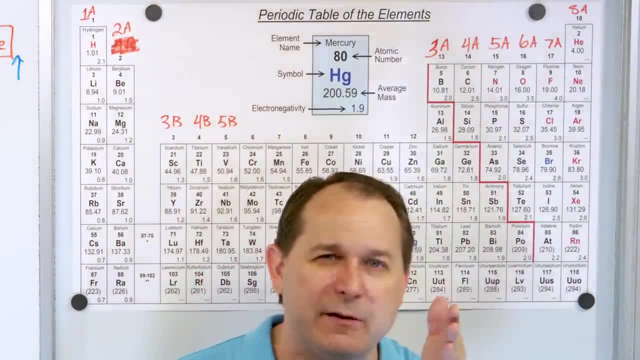 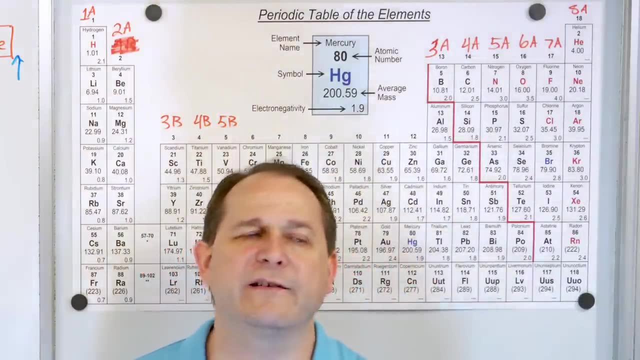 bottom line, and i'm going to teach you why that's the case later now. the elements next to the noble gases on either side are very reactive because they're always trying to get an electron structure as close as possible to the noble gases. why? because the noble gases are really stable and 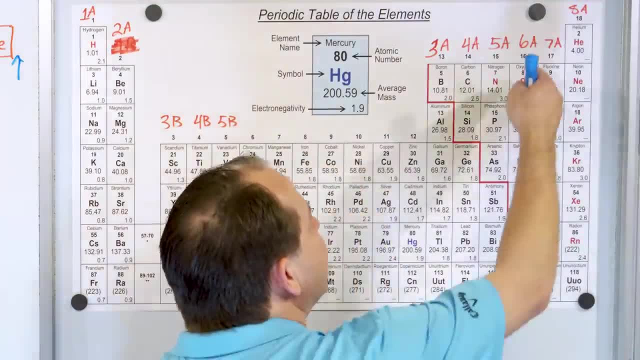 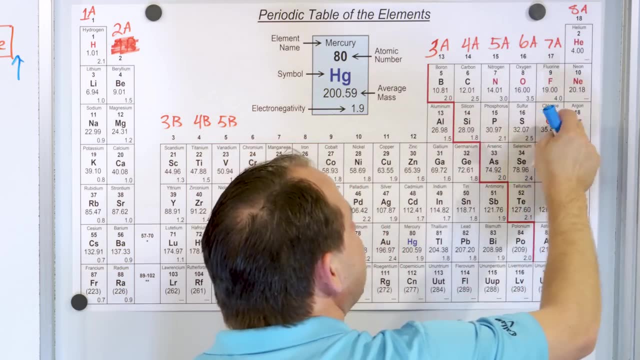 the force, the electric force can hold everything in place. so everything to the left is trying to gain a single electron to be close to these. every uh thing two spaces over is trying to gain two electrons to be close to its noble gas. over here, this, this group, is trying to lose an electron to 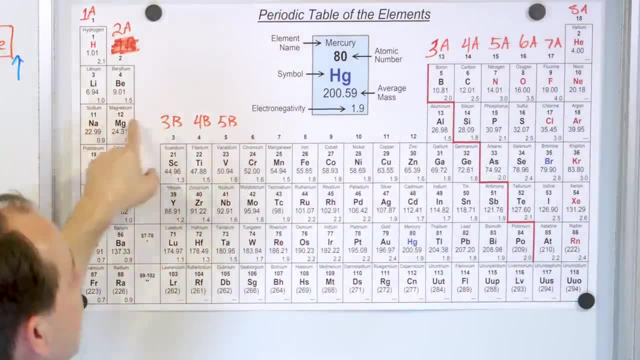 become like its nearest noble gas. it's trying to lose an electron to be like its nearest noble gas, and the same thing this one's trying to lose to be like its nearest noble gas. and then the one here is trying to lose two electrons and lose two electrons. so there's a symmetry right. the ones. 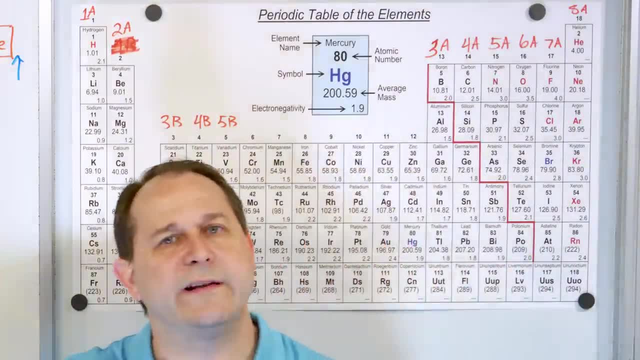 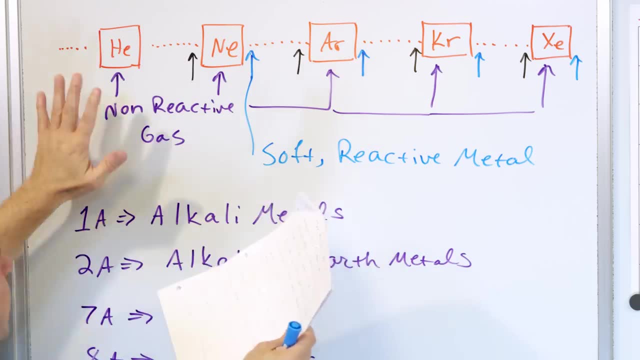 near the right hand side are trying to gain one or two electrons. the ones on the other side of the table are trying to lose one or two electrons and this is the pattern that we laid out in the beginning of the lesson that i was telling you, the periodic nature. we said this table has rows which 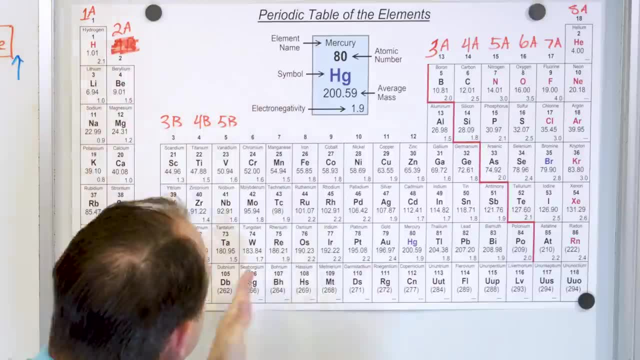 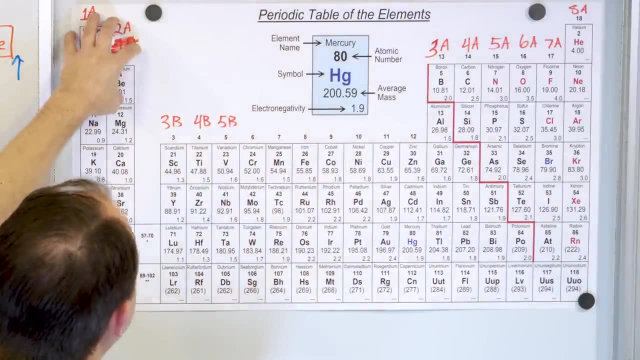 we call periods and it has uh, columns which we call groups, and we said that the, the names of the groups, have basically changed over the years. in older books you see these main group elements which are all of these and all of these labeled one a, two a, and then all the way through through 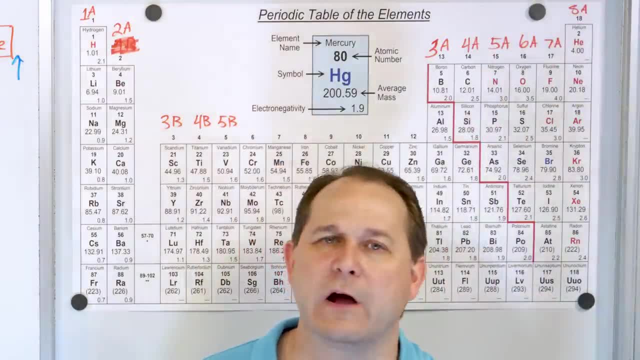 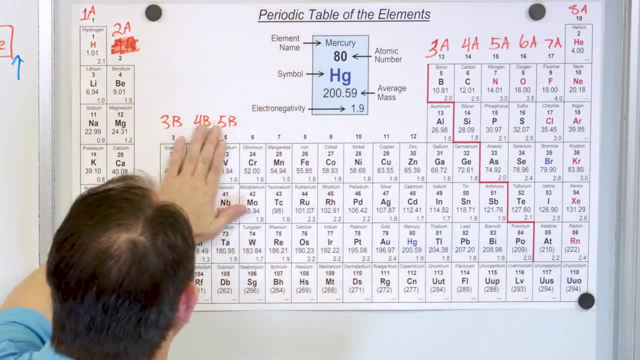 eight a. the reason there's eight is because of electrons. we'll talk about later why. but they're very important and that then. that's why. but that's why they're this way. we call these the transition uh metals and they have b's associated with them. again, to differentiate the difference in. 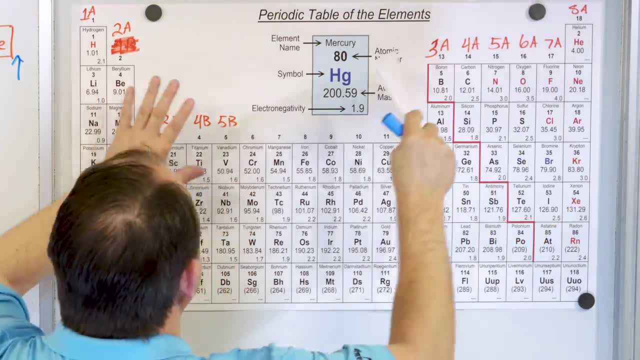 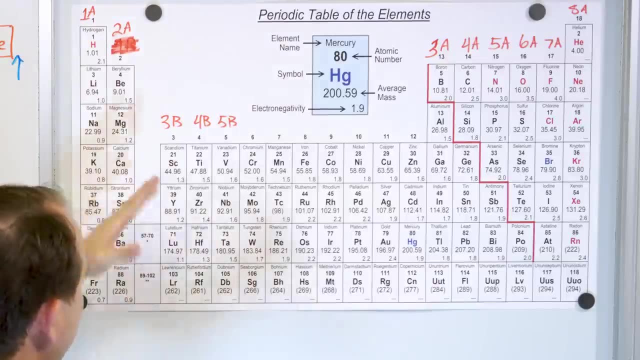 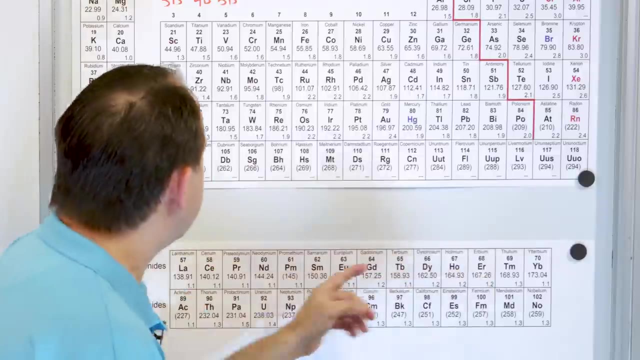 the way the electrons are laid out between the, this group of elements and then these right here. all right, and then we basically said that this table is constructed always on every book you'll ever see, it's got the book. uh, here the table listed as we have here, with two extra rows down here: one row called the or period called 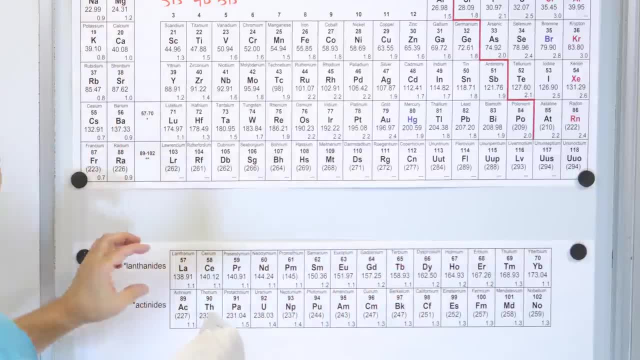 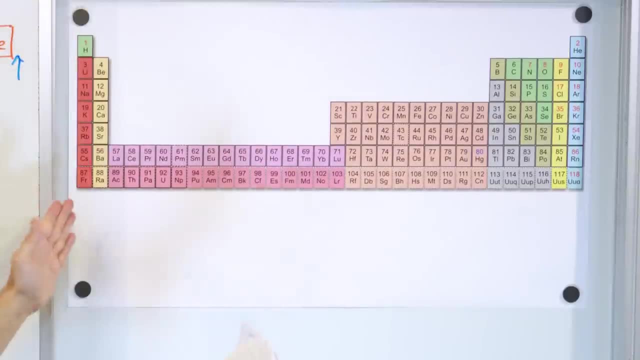 and the other one called the actinides, and the way it's supposed to be drawn is to show you that this kind of fits in there and kind of spreads the table apart. so if you really drew the actual table, it would actually look like this, with the table spread far apart. this is going to help us a lot. 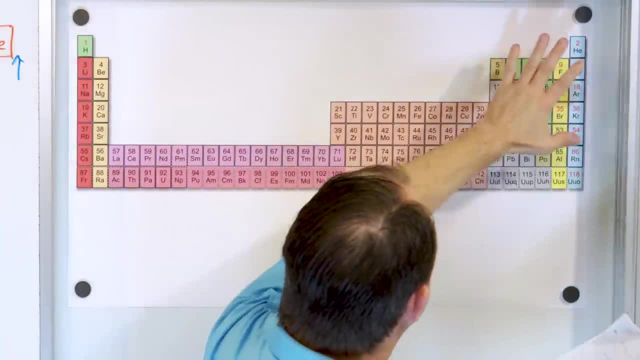 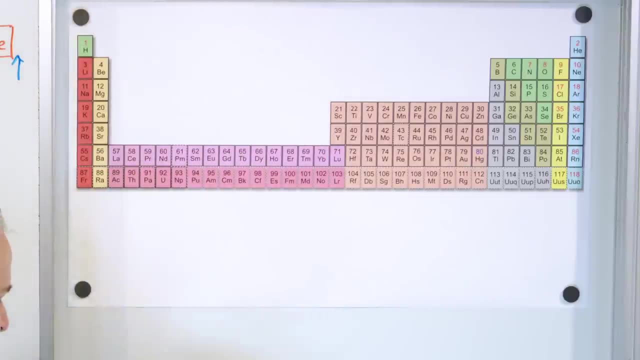 when we study electrons, to know what these different things, what these different areas of the table are. but you just don't usually see it like this because you can't print it on a page very easily. all right, then we said that we had some special names for some of these. 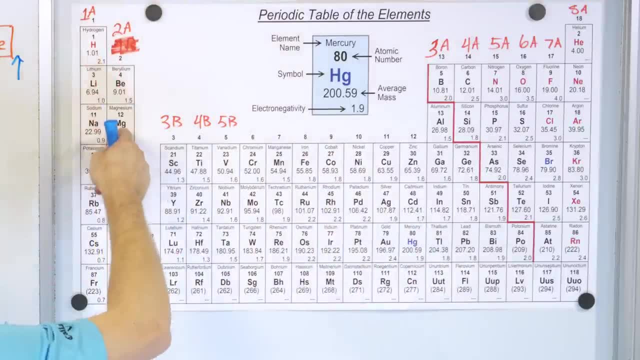 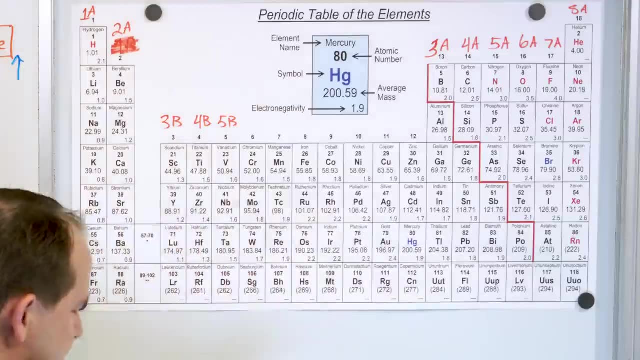 different groups. we had the alkali metals, we had the alkaline earth metals and then we had the halogens- this one here- and then we had the noble gases. and then we talked about metals and non-metals on the left and on the right: metalloids, right here near the stair step line: transition metals. 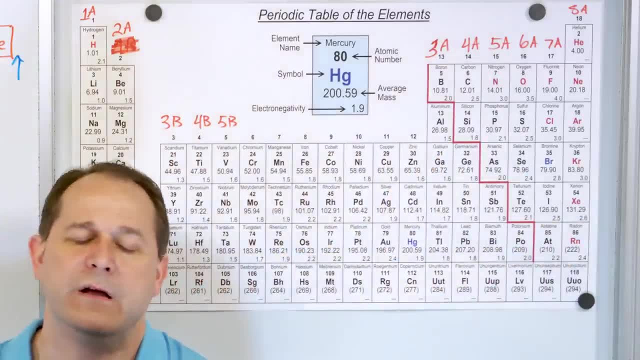 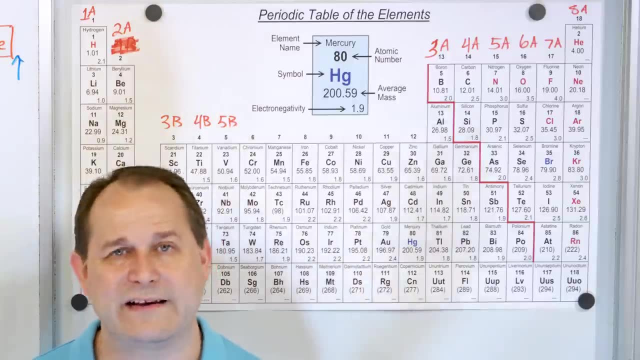 throughout here and that's basically it. then we did some practice, so i just wanted to go through it again, because it is a lot of information and i could have written all this stuff down, but at the end of the day it's going to be faster. if you just watch this lesson a few times, you know. 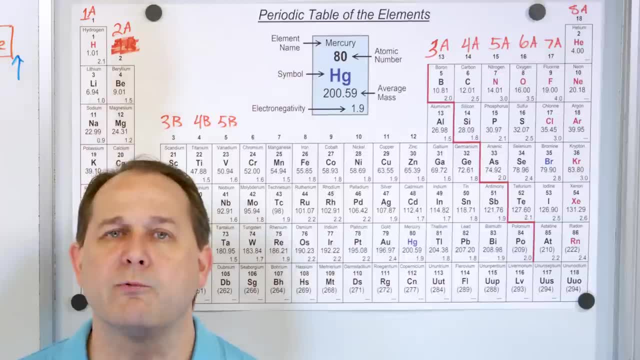 it's going to be faster. if you just watch this lesson a few times, you know, i promise you, what we'll do in the next lesson. we'll solve a few more problems here and then, as we really study chemistry and use what's on this table because of this introductory lesson, you're 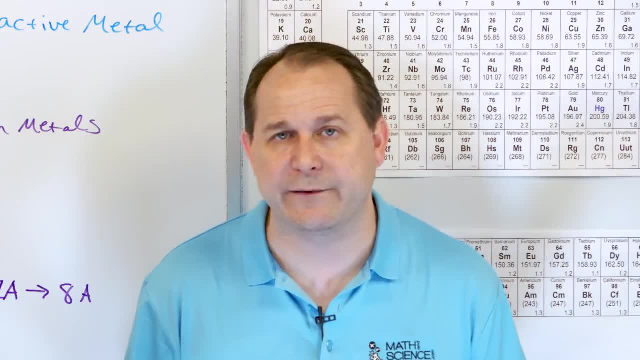 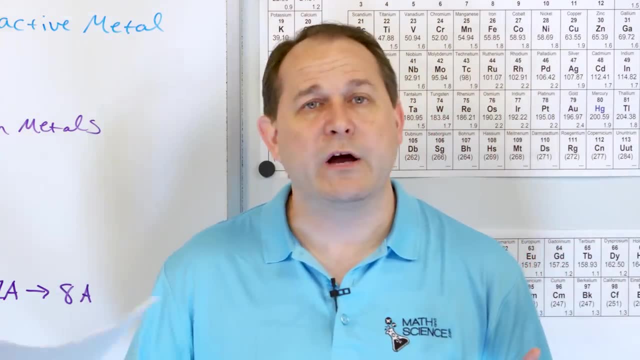 already. you already know now what this table is used for. i have not hidden anything from you. a lot of books and teachers will kind of hide what the table is for until later. i've given it to you, so now, when we go in the next few lessons and write down what a chemical compound looks like, 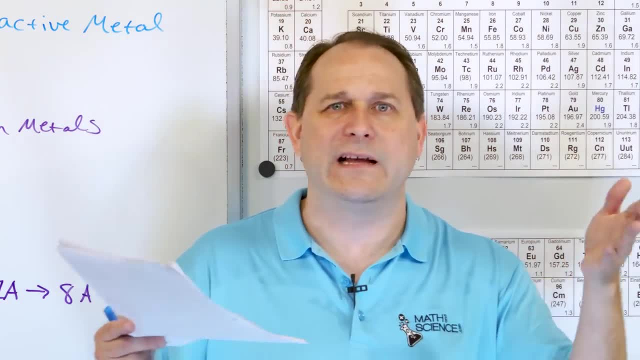 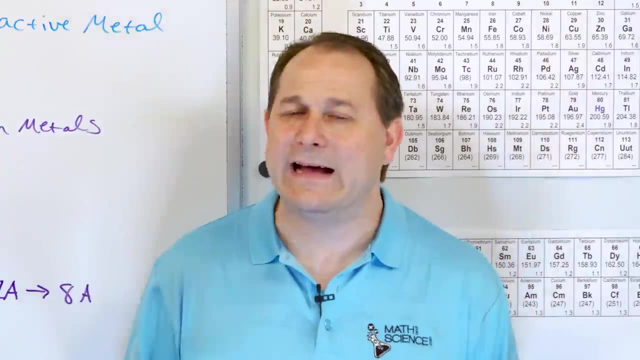 you're going to know. we're going to review it again, but you basically know how the electrons are doing their thing and we're going to apply that in future lessons and it might take a few times for you to really for it to sink in. that's okay. it took hundreds of years to discover this stuff, so if it takes, 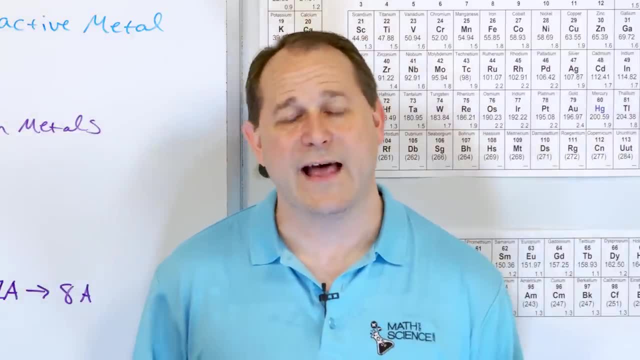 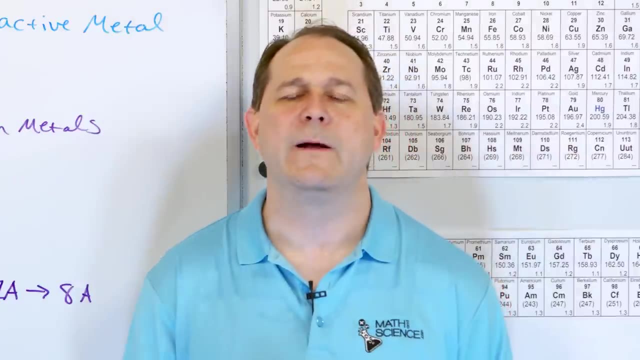 you a few watching a few viewings of a video. please cut yourself some slack. nobody learns this stuff overnight. i'd like you to watch this a few times when you feel like you understand what's going on. follow me on the part two. we'll do a couple more problems. 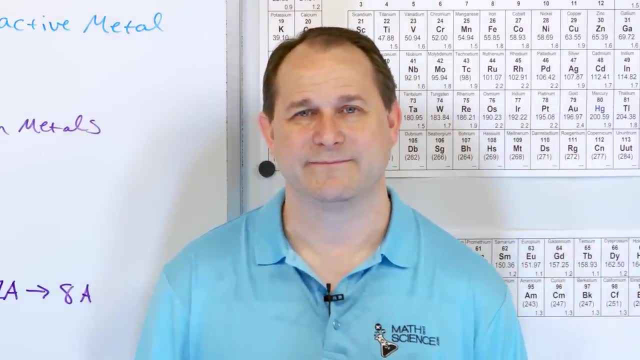 just getting practice with using the periodic table.